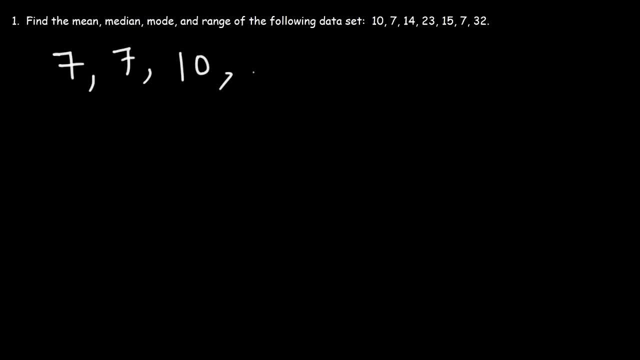 them. After that, the next number is 10, and then 14,, 15,, 23, and 32.. Now, to calculate the mean, what we need to do is we need to take the sum of the seven numbers and divide it by the seven numbers that are in the data set. So this is going to be: 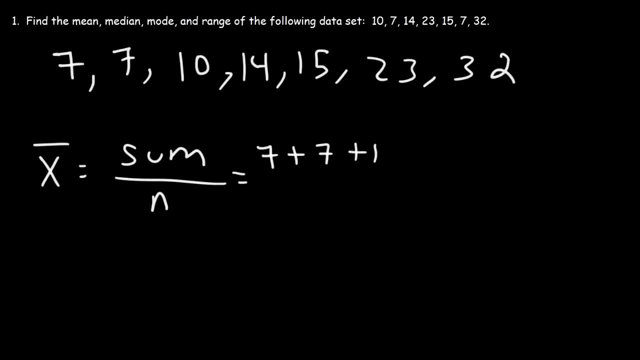 7 plus 7 plus 10 and so forth, And then we're going to divide it by the seven numbers, So the mean is basically the average of those numbers. So the total sum that I got is 108.. If you take 108 and divide it by 7, that's. 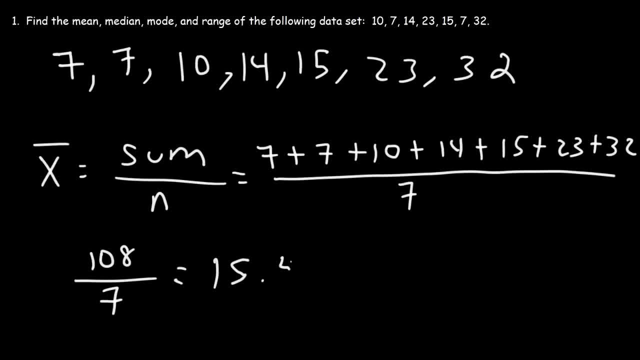 going to give you 15.43.. I'm going to round it to 3,, so it's approximately 15.43.. So that is the mean. That's how you can find it. Now, what about the next thing? How can we find the median of this data set, The? 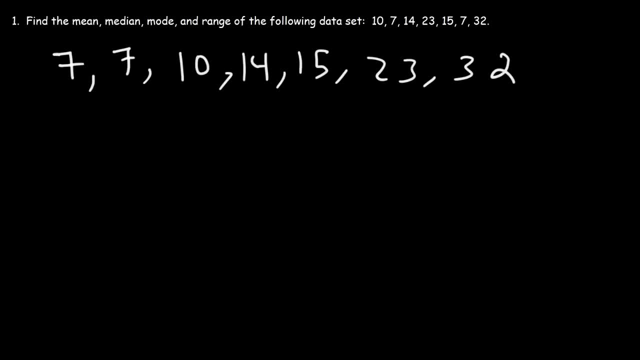 median is basically the middle number. so what I'd like to do is eliminate the first and the last number and then, working towards the middle, I'm going to eliminate the next two numbers until I'm left with the middle number. so, as we could see in this example, the median is equal to 14. it's simply the middle. 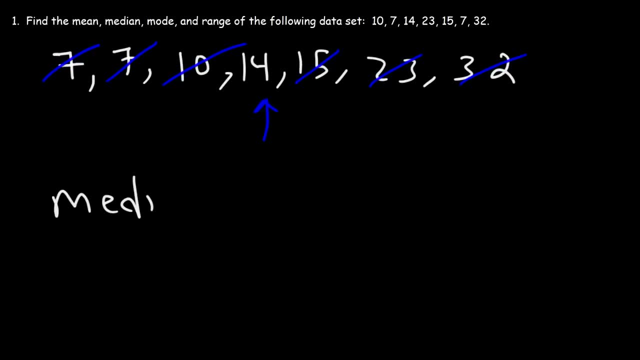 number of the data set. now what about the mode? what is the mode in this problem? the mode is simply the number that occurs the most frequently. I think I said that wrong. it's basically the, the most frequent number in the data set. and notice that seven appears twice in this data set. so seven is the mode. now what? 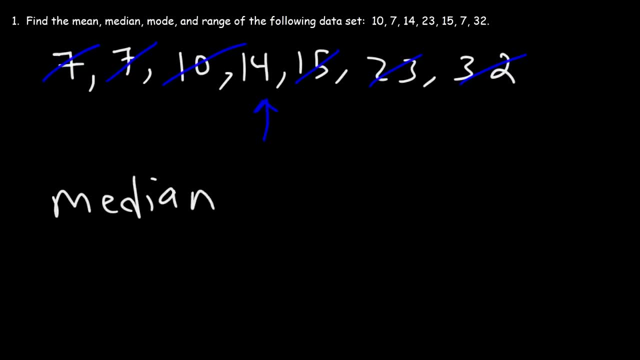 this example, the median is equal to 14.. it's simply the middle number of the data set. now what about the mode? what is the mode in this problem? the mode is simply the number that occurs the most frequently. i think i said that wrong. it's basically the the most frequent number in the data set. 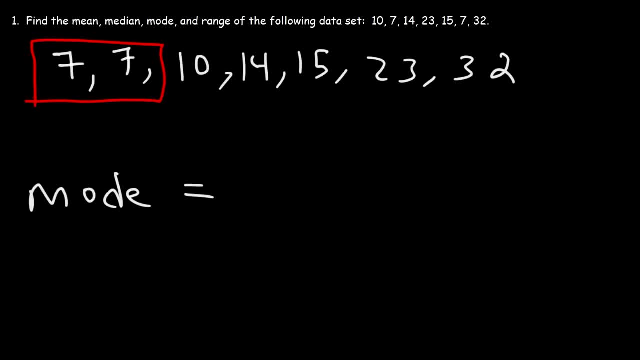 and notice that 7 appears twice in this data set. so 7 is the mode. now what about the range? the range is simply the difference between the highest number and the lowest number, so it's going to be 32 minus 7, which is 25.. 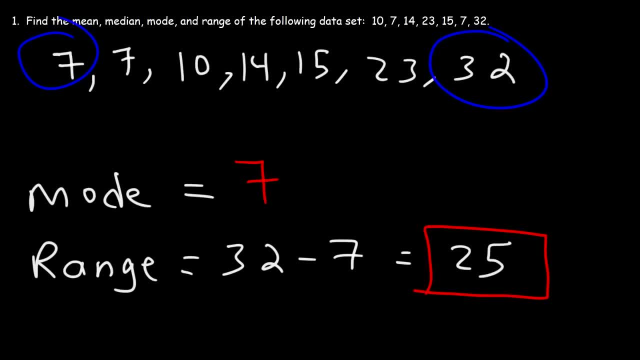 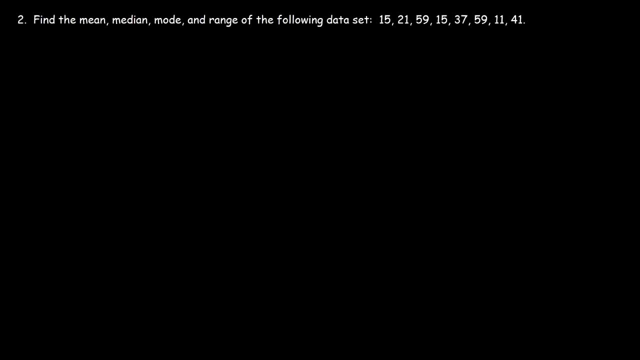 and so now you know how to find the mean, median mode and range of a data set. now let's move on to number two. now, this is going to be a similar problem, but it's not exactly the same. as you can see, we have eight numbers in our data set, as opposed to the seven that we had. 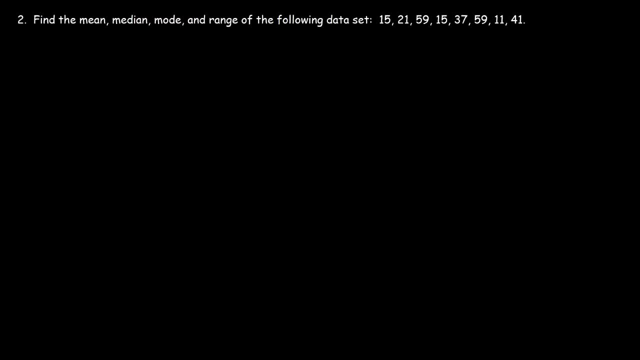 previously. so let's begin by putting these numbers in order. so the lowest number is 11, and then the next number is 15, and then we have 21, and then 37, 41 and 59. so let's begin by calculating the mean. so the mean represented by the symbol x bar is equal to the sum divided by the 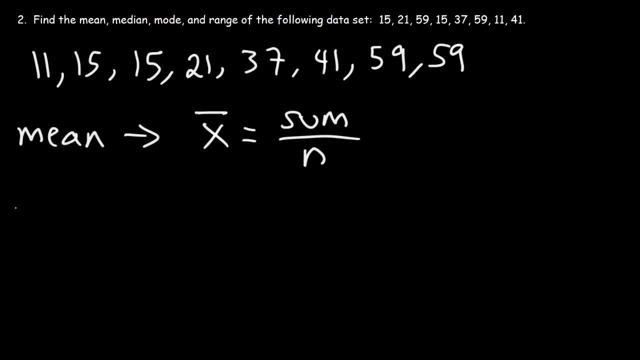 number of numbers in the data set. so let's add up the eight numbers- this is going to take some time- and then divide the sum by those eight numbers. so we have 11 plus 15 plus another 15, and then 21, 37, 41 and 259. so i got a sum of 258 if we divide that by 8. 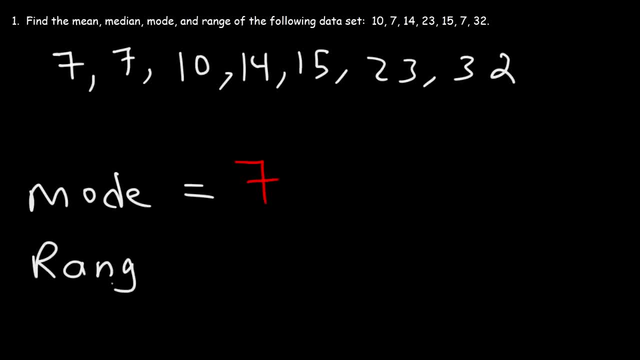 about the range. the range is simply the difference between the highest number and the lowest number, so it's going to be 32 minus 7, which is 25, and so now you know how to find the mean, median mode and range of a data set. now let's. 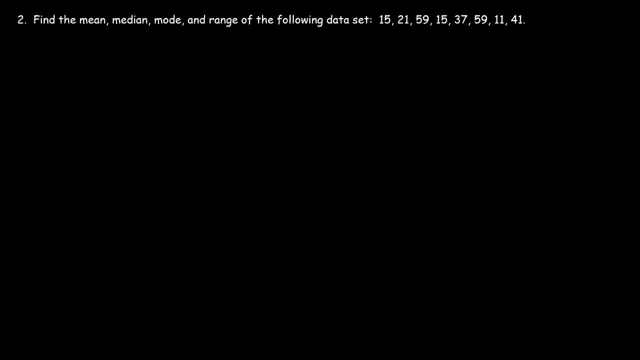 move on to number two now. this is going to be a similar problem, but it's not exactly the same. as you can see, we have eight numbers in our data set, as opposed to the seven that we had previously, so let's move on to number two now. this is going to be a similar problem, but it's 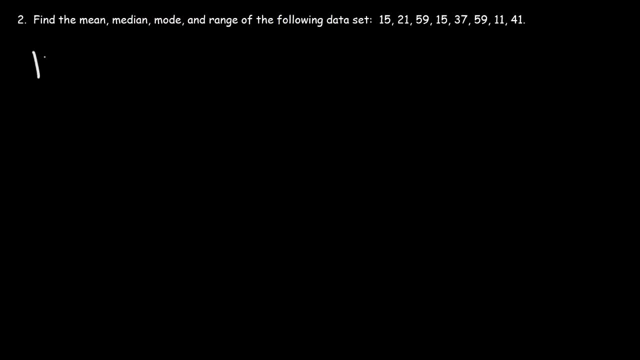 let's begin by putting these numbers in order. so the lowest number is 11, and then the next number is 15, and then we have 21, and then 37, 41 and 59. so let's begin by calculating the mean. so the mean represented by the symbol X bar is equal. 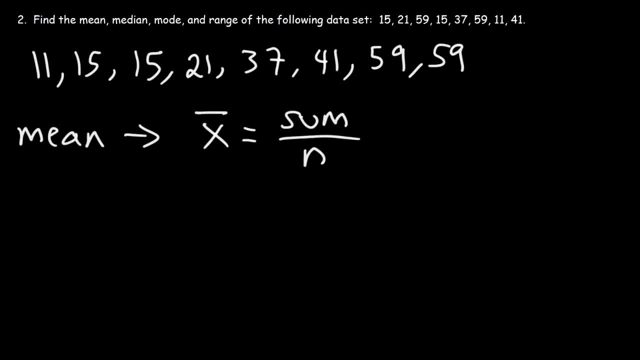 to the sum divided by the mean. so the mean represented by the symbol X bar is equal to the sum divided by the mean. so the mean represented by the number of database. so let's add up the eight numbers you toел. this is going to take some time and 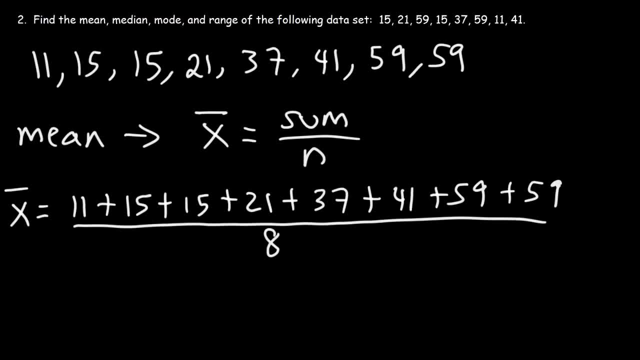 then divide the sum by those eight numbers, so we have 11 plus 9 real installed. so that's it now. our problem is that we'll continue our argument after 15 plus another 15, and then 21, 37, 41 and 259. so I got a sum of 258 if we divide. 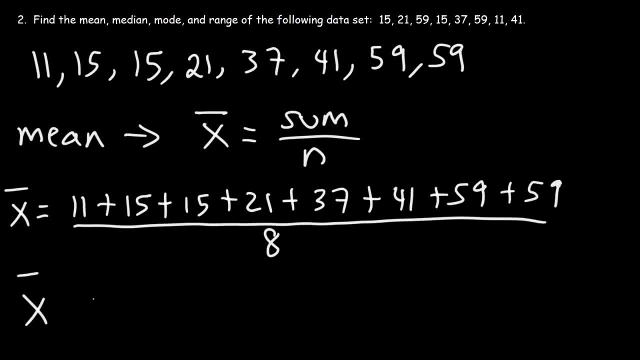 that by 8, you'll find that the mean is 32.25. so that's the answer for the first part of the problem. now let's move on to the second part. let's calculate the median. as we said before, the median is simply the middle number. so let's. 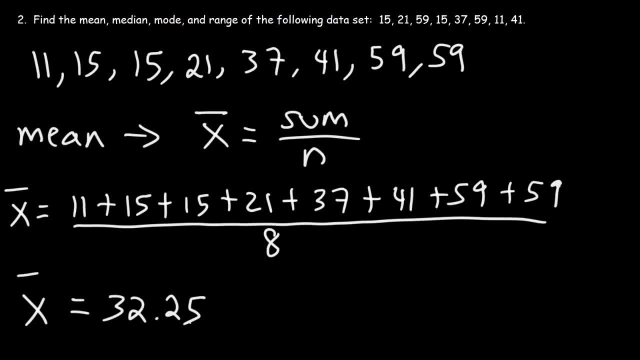 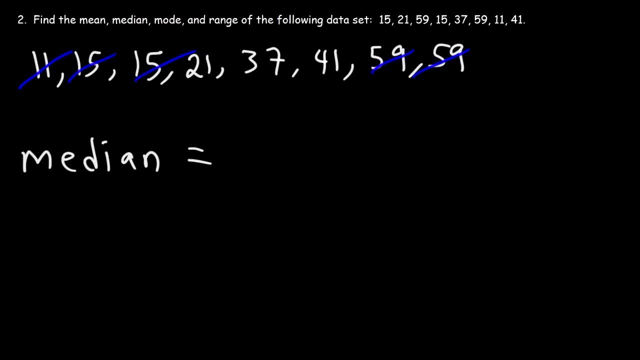 you'll find that the mean is 32.25. so that's the answer for the first part of the problem. now let's move on to the second part. let's calculate the median. as we said before, the median is simply the middle number. so let's eliminate the first and the last numbers, and then the next two and the next two. 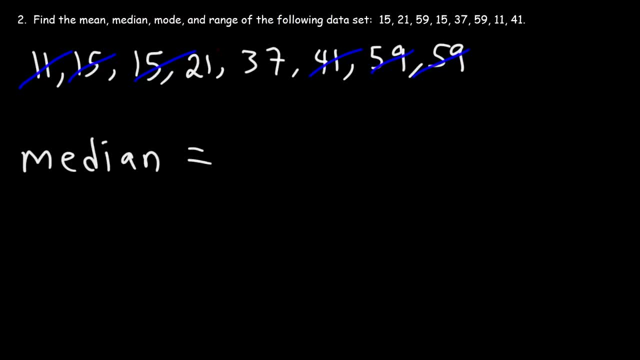 notice that we don't have one number in the middle, but this time we have two numbers in the middle. so what should we do if we come across a situation in this case? what you need to do is take the average of those two middle numbers, so you need to add them up and divide by two. 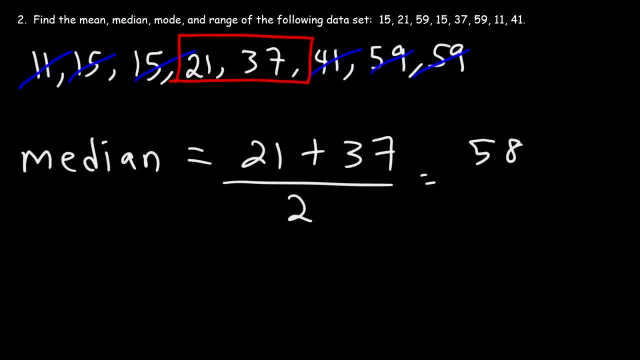 two plus three is five. seven plus one is eight. so 21 plus 37 is 58.. and if you divide it by two, this gives you 29. so 29 is the median in this data set. now, what about the mode? what is the mode in this? 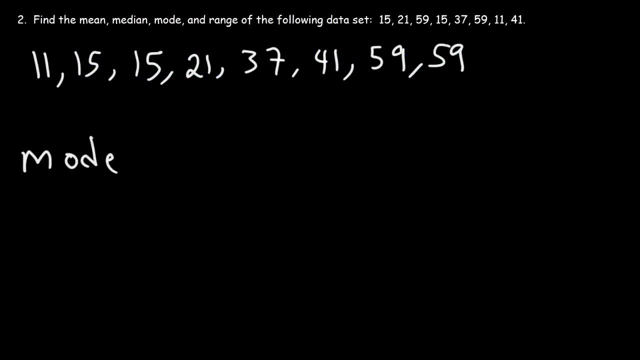 example. now, as we said before, the mode is the number, that is, basically it's the most frequent number in the data set. but this problem is different from the last one, because we have two numbers that appear twice, 15 and 59. so which of these is the mode? it turns out that they both represent the mode, so the 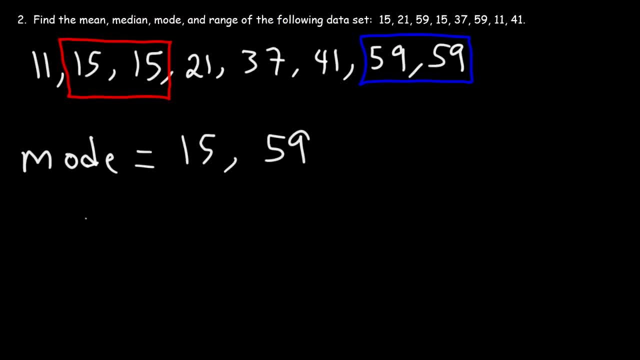 mode is 15 and 59.. so what we have is something known as a bimodal data set, because there's two modes instead of one. it's not unimodal. now, what about the range? well, there's nothing different about the range in this problem compared to the last problem. 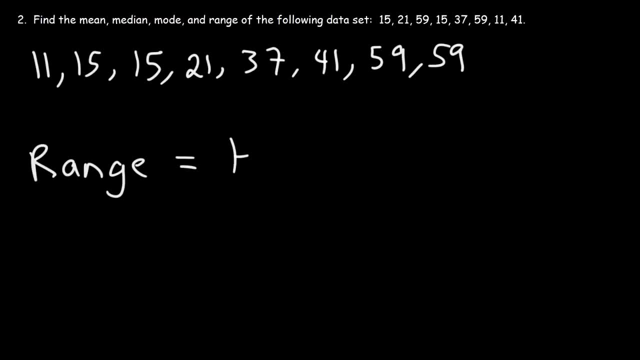 it's simply the highest number divided by the lowest number. so you can say h minus l, so the highest number is 59.. as we can see here, and the lowest number is 11.. so 59 minus 11 is 48.. so now you know how to find. 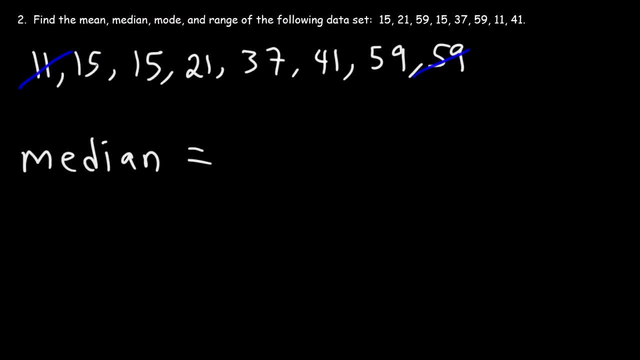 eliminate the first and the last numbers, and then the next two and the next two, notice that we don't have one number in the middle, but this time we have two numbers in the middle. so what should we do if we come across the situation in this case? what you need to do is take the average of those two. 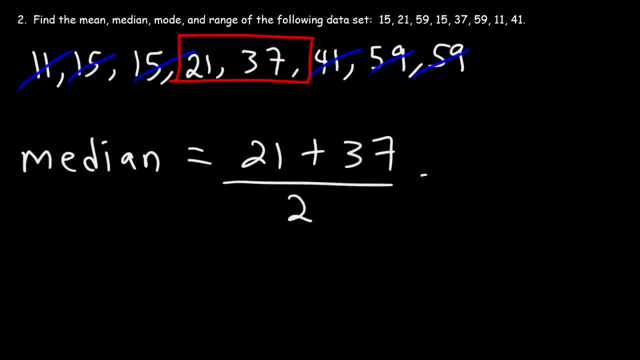 middle numbers. so you need to add them up and divide by 2. 2 plus 3 is 5, 7 plus 1 is 8. so 21 plus 37 is 58, and if you divide it by 2, this gives you 29, so 29 is. 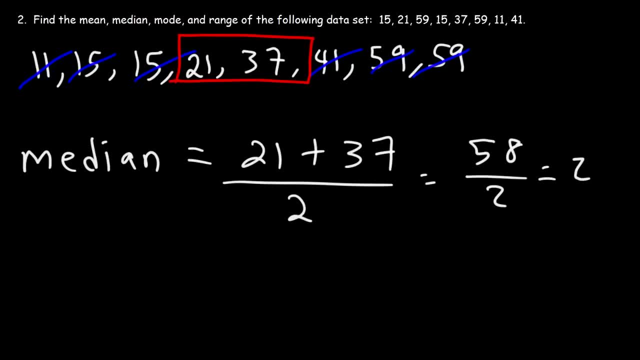 the median, and this is a data set. now, what about the mode? what is the mode in this example? now, as we said before, the mode is the number, that is, basically, it's the most frequent number in the data set. but this problem is different from the last one, because we 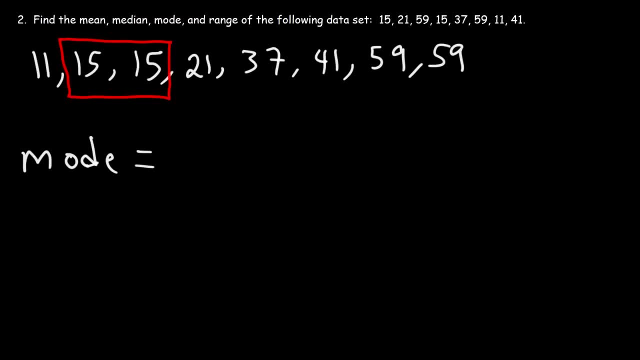 have two numbers that appear twice: 15 and 59. so which of these is the mode? it turns out that they're both represent the mode, so the mode is 15 and 59. so what we have is something known as a Bimodal data set, because there's two. 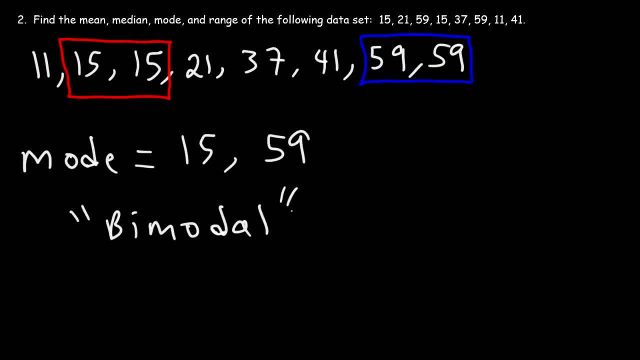 modes instead of one. it's not unimodal. now, what about the range? Well, there's nothing different about the range in this problem compared to the last problem is simply the highest number divided by the lowest number. so you can say H minus L, so the highest. 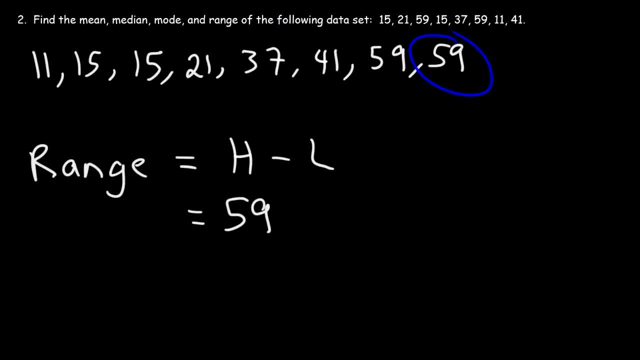 number is 59, as we could see here, and the lowest number is 11. so 59 minus 11 is 48. so now you know how to find the mean, median mode and range of a data set. now let's talk about finding the quartiles and the interquartile range. so 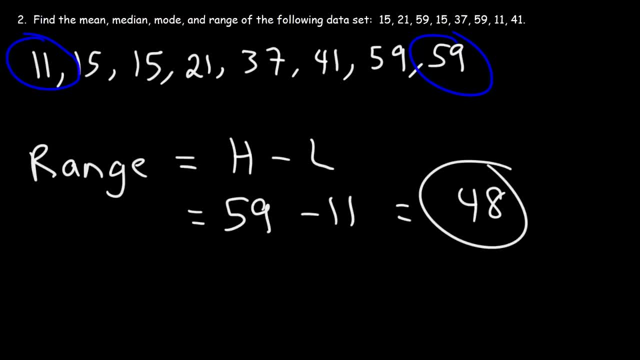 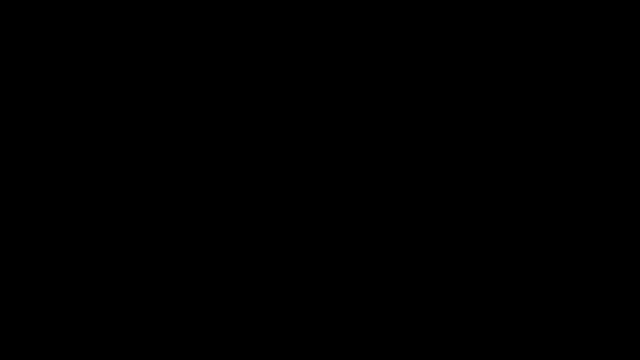 the mean, median, mode and range of a data set. now let's talk about finding the quartiles and the interquartile range. so what i'm going to do right now is i'm going to make basically a number line with a beginning and an end, and let's say, this number line represents 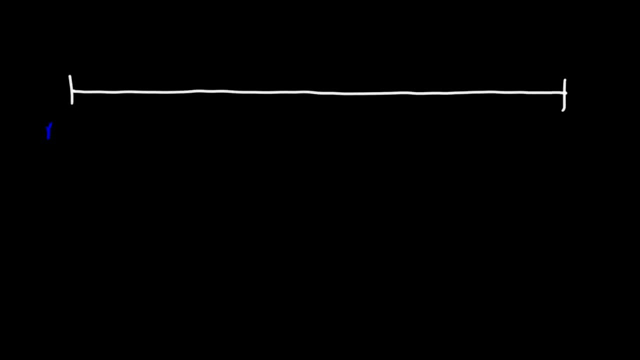 our data, the lowest value is known as the minimum. the highest value in our data set is the maximum. now we're going to break this number line into four equal parts. the first part is known as q1. this is the first quartile. the second one is q2. the second one is q2. 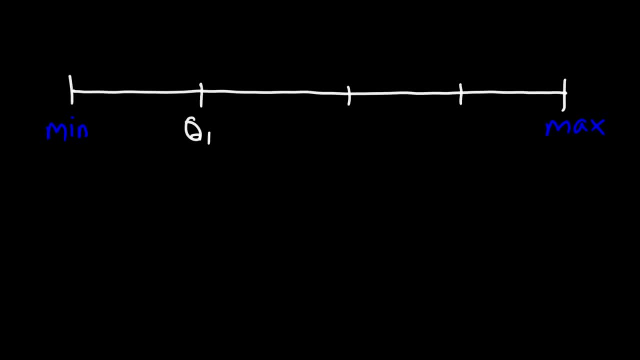 p. this is the first quartile, the second one is q2, the second one is q2, the second one is q2, the second quartile, and then this is the third quartile. So let's say, if the data was normally distributed, this would be at a 0% level. this would be 25,, 50,, 75,. 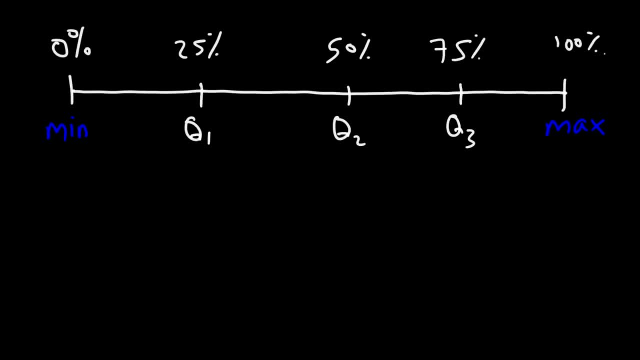 and then this will be 100. So you could see how the quartiles are related to each other respectively. Now how do we go about finding Q1,, Q2, and Q3? How do we do that? Q2 is basically the median of the entire data set. Q1 is the median of the 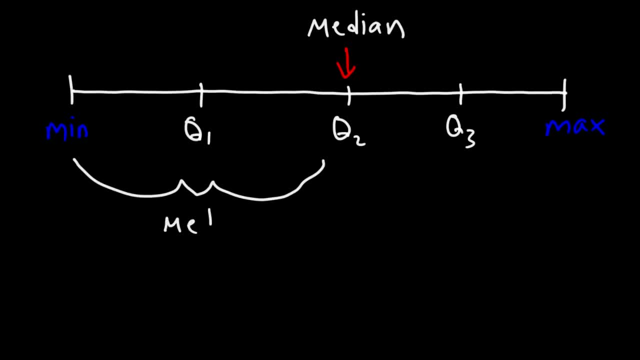 lower half of the dataset And Q3 is the median of the upper half of the dataset. Now, how do we go about finding out and able to estimate the of the data set? Now the interquartile range represented by IQR. this is the 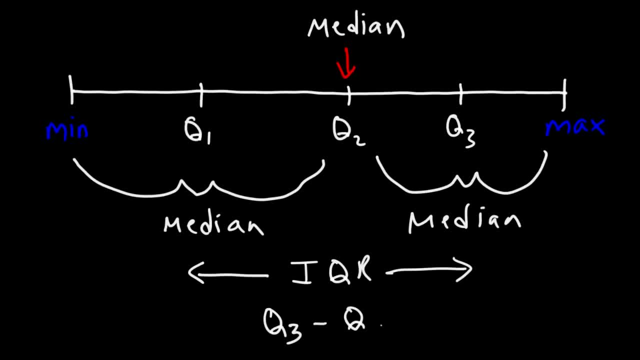 difference between Q3 and Q1.. So once you find Q1 and Q3, you can now calculate the interquartile range. Now the next thing that I want to mention is the ability to find or identify if a number in the data set is an outlier. So here's what you. 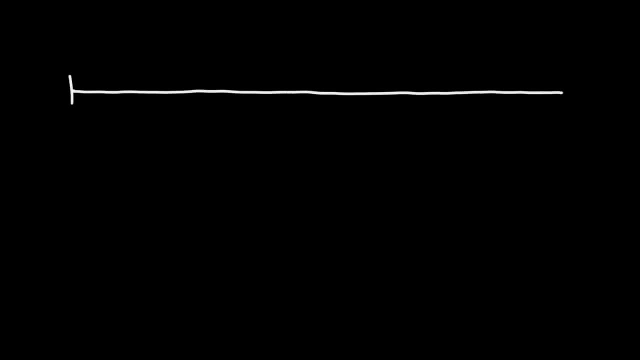 what I'm gonna do right now is I'm gonna make basically a number line with a beginning and an end and let's say this number line represents our data. the lowest value is known as the minimum. the highest value in our data set is the maximum. now we're going to break this number line into four equal parts. the first: 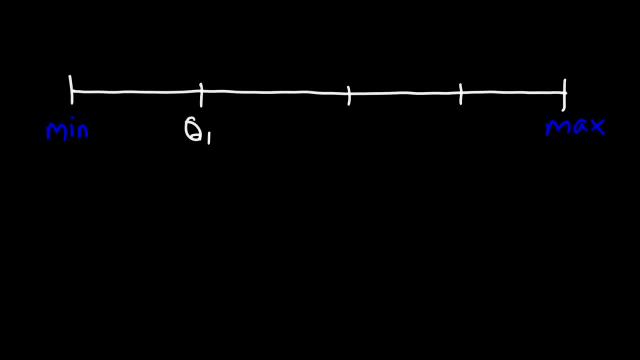 part is known as q1. this is the first quartile. the second one is q2, the second quartile, and then this is the third quartile. so let's say, if the data was normally distributed, this would be at a 0% level. this would be 25,, 50,. 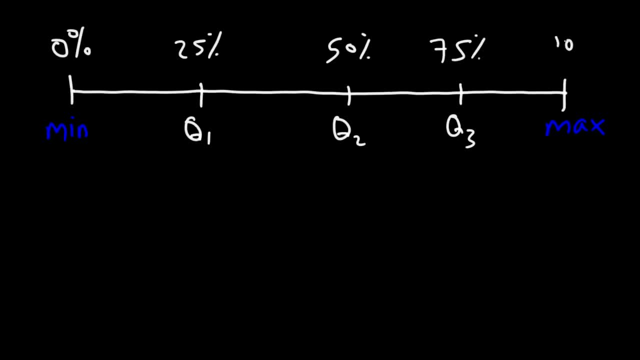 70,, 75 and then this will be 100. so you could see how the quartiles are related to each other respectively. now how do we go about finding q1, q2 and q3? how do we do that? q2 is basically the median of the entire data set. q1 is the median of 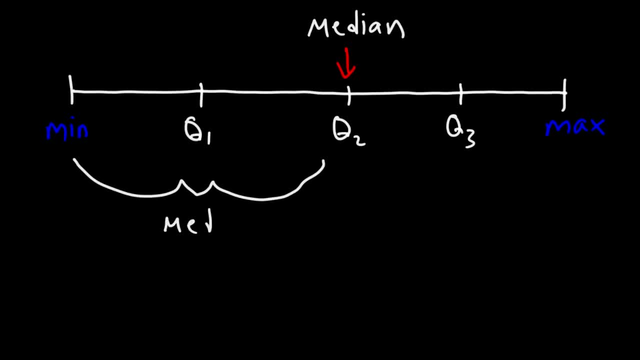 the lower half of the data set, and q3 is the median of the upper half of the data set, now the interquartile range represented by IQR. this is the difference between q3 and q1. so once you find q1 and q3, you can now calculate the interquartile range. 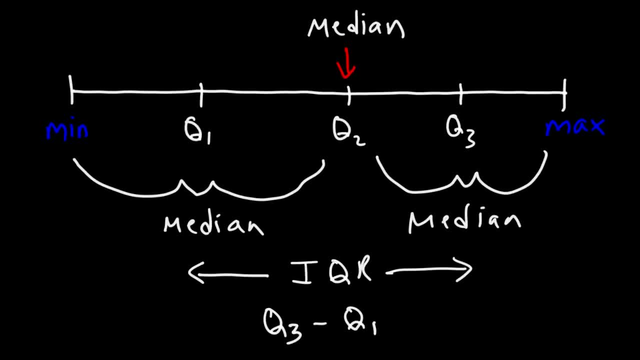 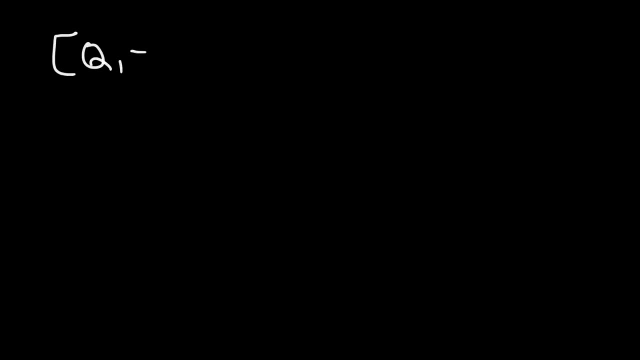 now, the next thing that I want to mention is the ability to find or identify if a number in the data set is an outlier. so here's what you need to know: it's not going to be an outlier if it's within this range, if it's between q1 minus 1.5 times the IQR. so that's the lowest that. 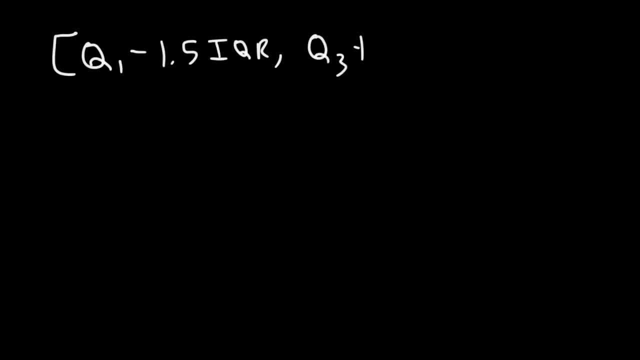 it can be, where the highest it can be is q3 plus 1.5 times the IQR. So if you have a number that is within this range, it is not an outlier, But if you have a number in the data set that is outside of this range, 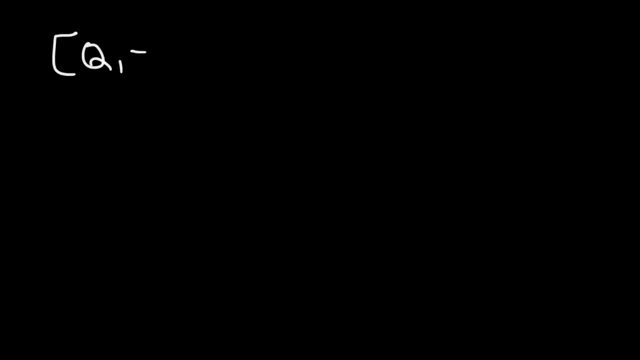 need to know It's not going to be an outlier if it's within this range, If it's between Q1 minus 1.5 times the IQR. So that's the lowest that it can be, or the highest it can be is Q3 plus 1.5 times the IQR. 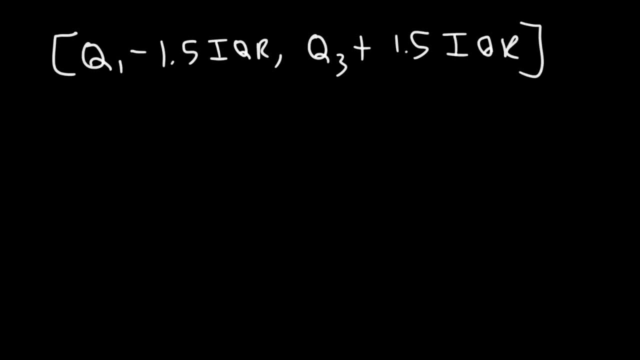 So if you have a number that is within this range, it is not an outlier, But if you have a number in the data set that is outside of this range, and then that number is an outlier. So let's work on an example. Let's say we have the numbers. 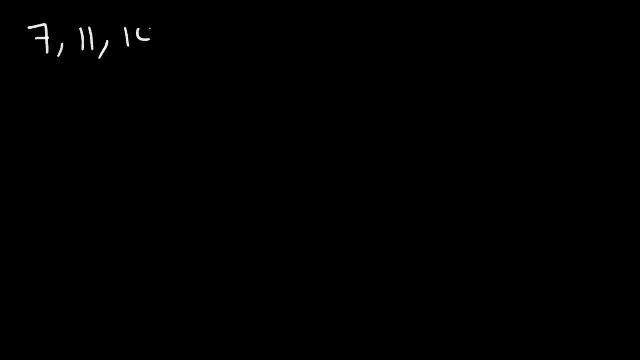 7,, 11,, 14,, 5,, 8,, 27,, 16,, 10,, 13,, 17, and 16.. Go ahead and identify Q1,, Q2, and Q3.. Calculate the interquartile range and determine if there are any outliers in its. 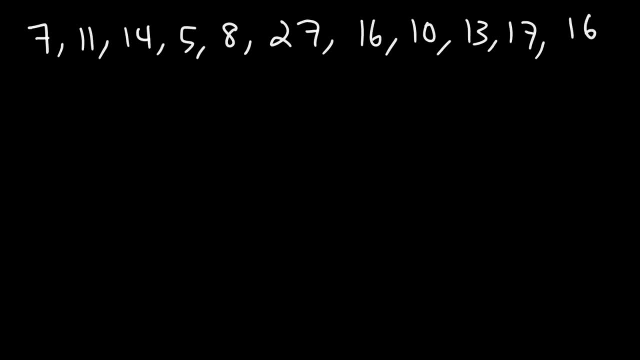 data set. Feel free to pause the video and use what you know to try it. now, as always, the first thing we should do is organize the data. the lowest number is 5, and then we have 7, 8, 10, 11. perhaps it's best if we cross it off as we go along and then 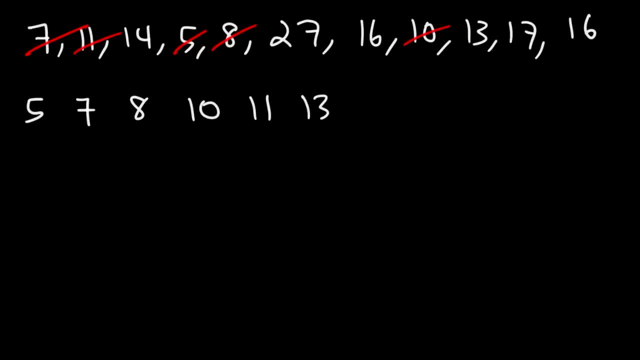 the next number is 13, and then 14, 16, there's two 16s and then the 17 and then 27. now, what do you think is our next step in order to find the interquartile range and the three quartiles? what's our next step, the best thing to do at this? 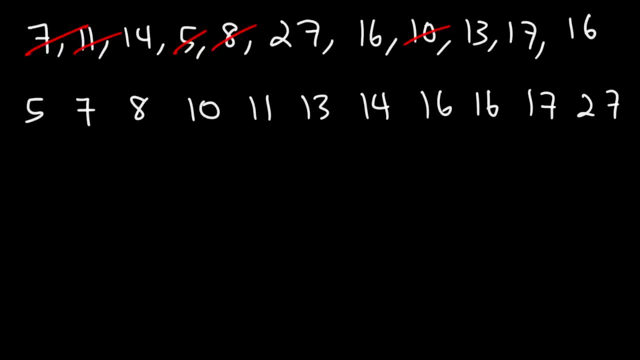 point is to determine the median of the entire data set, which is going to be q2, so we could eliminate the first two numbers, the first and the last number, and then the next two until we get a number. you in the middle, so notice that 13 is in the middle. so therefore, 13 is going to. 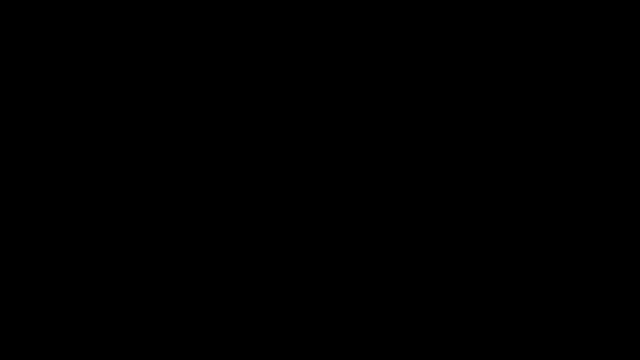 then that number is an outlier. So let's work on an example. Let's say we have the numbers 7,, 11,, 14,, 5,, 8,, 27,, 16,, 10,, 13,, 17, and 16.. 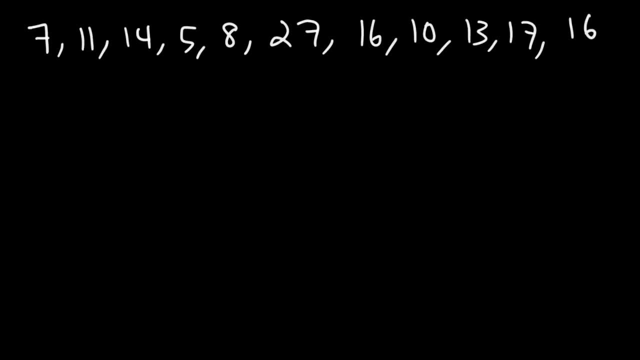 Go ahead and identify Q1,, Q2, and Q3.. Calculate the interquartile range, the IQR, and determine if there's any outliers in this data set. Feel free to pause the video and use what you know to determine if there's any outliers in this data set. 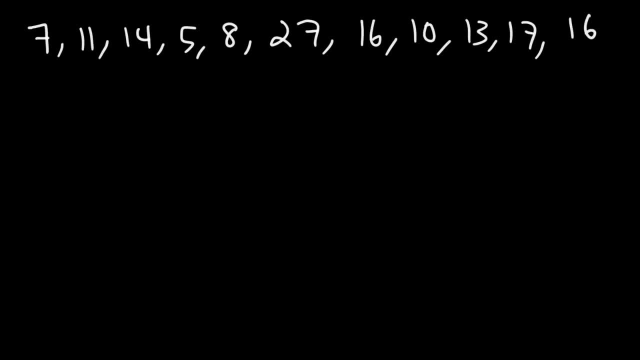 Now, as always, the first thing we should do is organize the data. The lowest number is 5. And then we have 7,, 8,, 10,, 11.. Perhaps it's best if we cross it off as we go along. 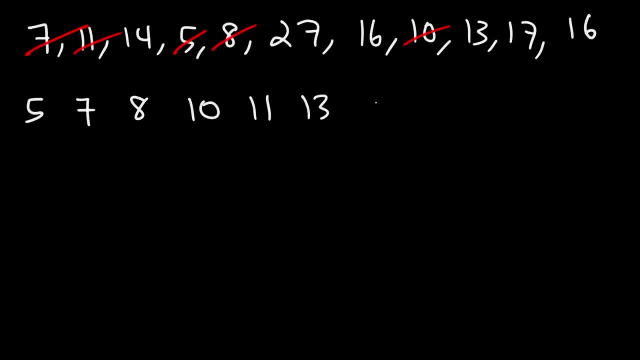 And then the next number is 13.. And then 14,, 16. There's two 16s, And then the 17. And then 27.. Now, what do you think is our next step in order to find the interquartile range? 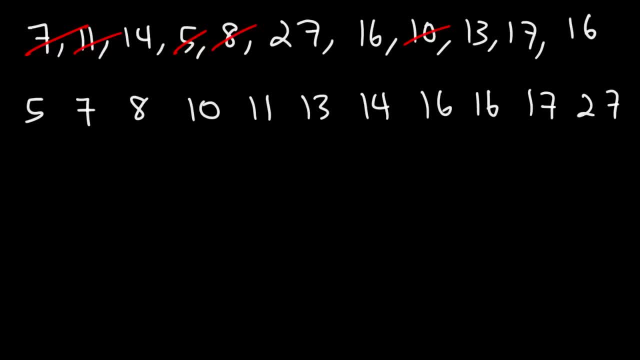 and the three quartiles. What's our next step? The best thing to do at this point is to determine the median of the entire data set, which is going to be Q2.. So we could eliminate the first two numbers, the first and the last number. 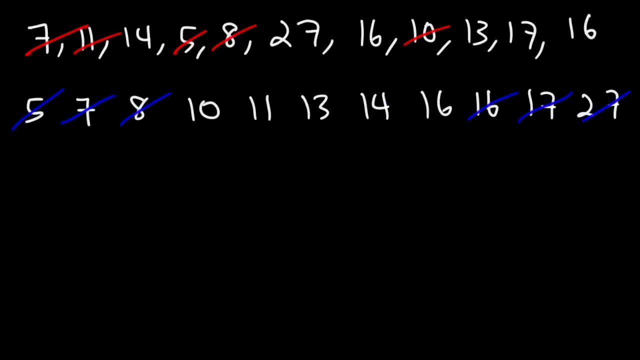 and then the next two until we get a number in the middle. So notice that 13 is in the middle. So therefore, 13 is going to be Q2.. Now what I like to do is I'm going to get rid of this number for now. 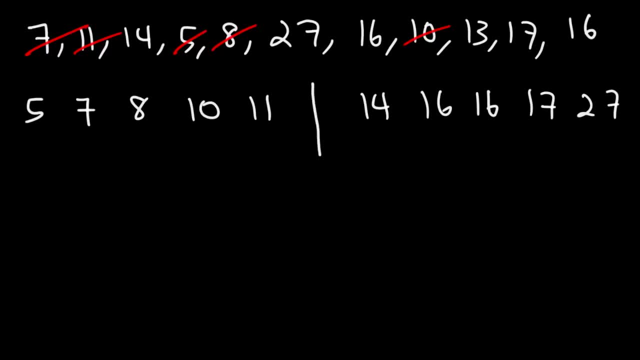 And I'm going to put a line between the left side and the right side. So I want to separate the lower half of the data set with the upper half. So I'm going to put a line between the left side and the upper half of the data set. 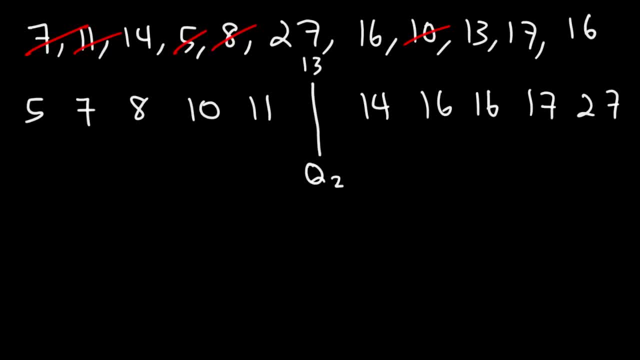 But the 13 is still here though, So just keep that in mind. So that's our Q2 value. Now, Q1 is the median of the lower half of the data set. So what is the median of those five numbers? 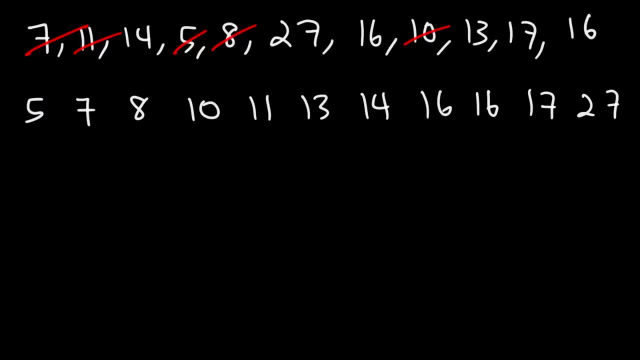 be q2. now what I like to do is I'm gonna get rid of this number for now and I'm going to put a line between the left side and the right side, so I want to separate the lower half of the data set with the upper half of the data set, but 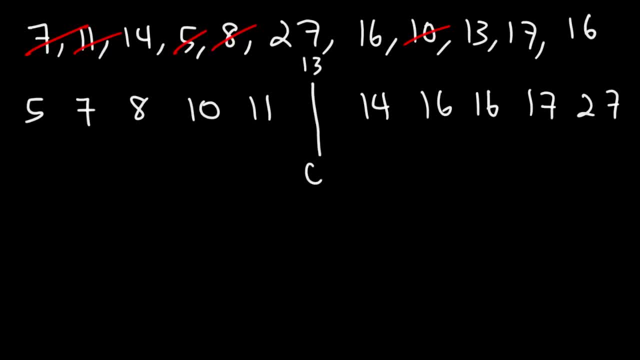 the 13 is still here, though, so just keep that on. so that's our Q2 value. now, q1 is the median of the lower half of the data set. so what is the median of those five numbers? the median is simply going to be the middle number of those five. 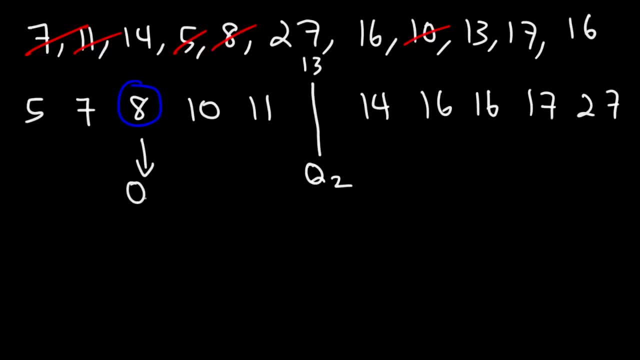 numbers. so q1 is 8. now what is the median of the upper half of the dataset? notice that the middle number is 16, so that is q3. notice that we have a total of 11 data points, and so that's why 13 is not included in the lower half or the upper half, because if it was, 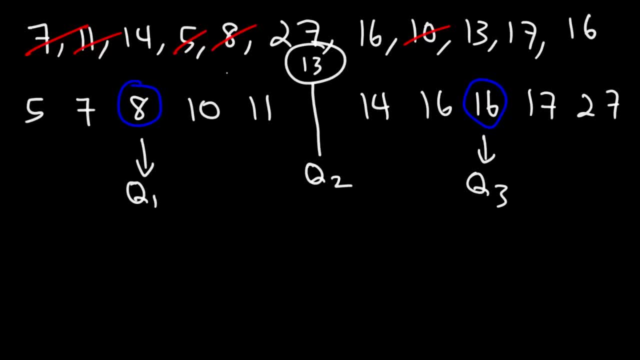 one side will have five numbers, the other side will have six, and that's why i chose to write it up here, so that the lower half is the same as the upper half. they both contain five numbers. now let's go ahead and calculate the interquartile range, iqr. so we said it's the difference between: 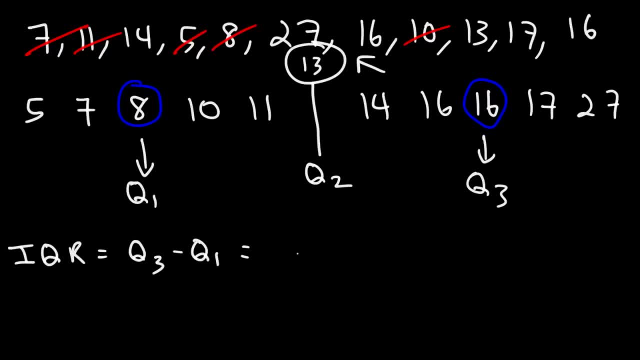 the third quartile and the first quartile. so it's going to be 16 minus 8, which is 8, and so that's how you could find the interquartile range of a data set. now, what about the presence of any outliers? so, looking at these numbers, do you think we have? 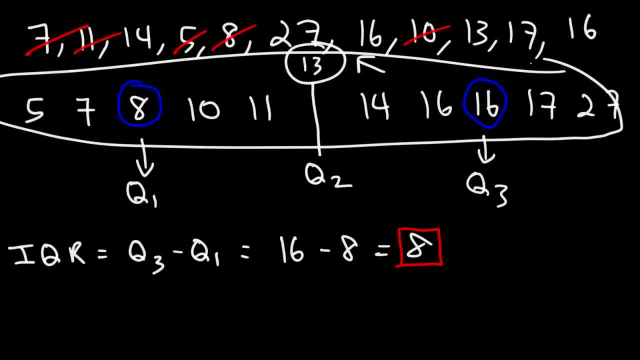 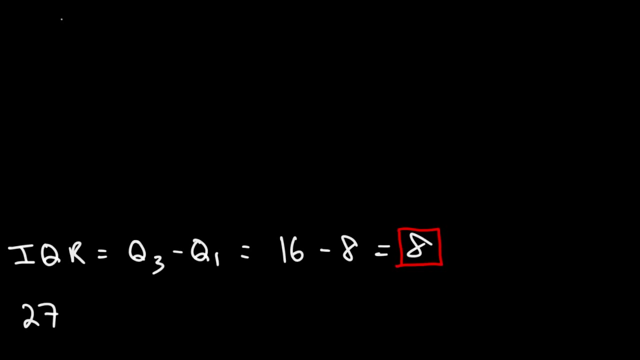 a number that really stands out, that doesn't belong. right now, 27 appears to be very far off from all the other numbers. so do you think 27 is an outlier? well, let's find out. so let's write down what we know. the presence of an outlier is based upon this range. it's q1 minus 1.5 times the iqr. 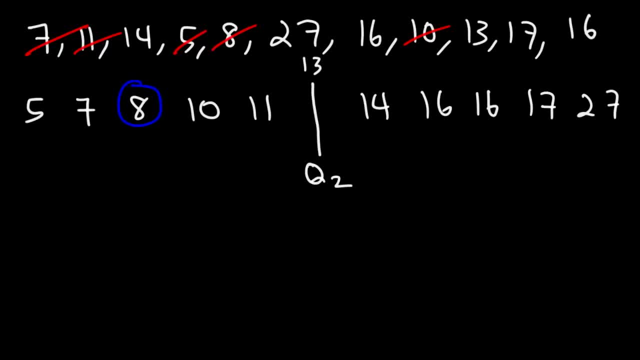 The median is simply going to be the middle number of those five numbers. So Q1 is eight. Now what is the median of the upper half of the data set? Notice that the middle number is 16.. So that is Q3.. 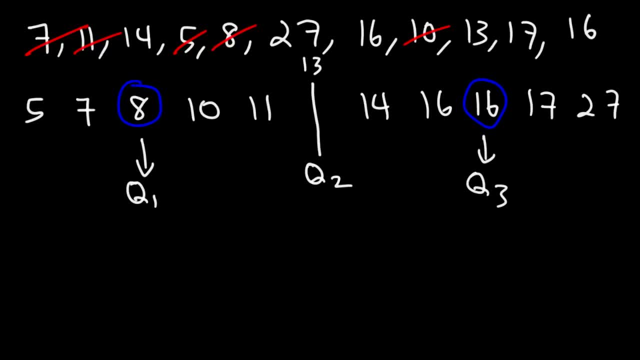 Notice that we have a total of 11 data points, And so that's why 13 is not included in the lower half or the upper half, Because if it was, one side will have five numbers, the other side will have six, And that's why I chose to write it up here. 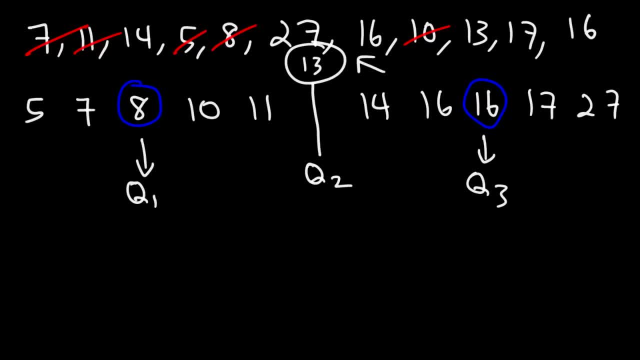 so that the lower half is the same as the upper half. So that's why I chose to write it up here, so that the lower half is the same as the upper half. So that's why I chose to write it up here, so that the lower half is the same as the upper half. 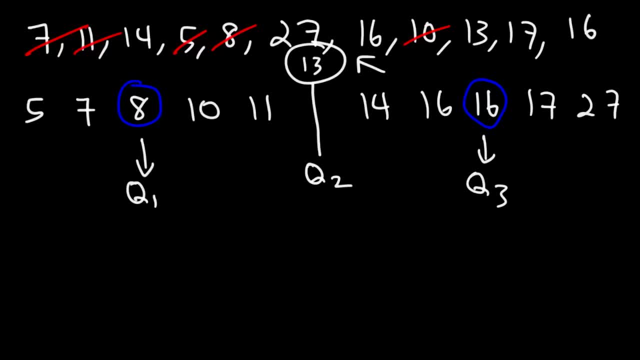 They both contain five numbers. Now let's go ahead and calculate the interquartile range, IQR. So we said it's the difference between the third quartile and the first quartile. So it's going to be 16 minus 8, which is 8.. 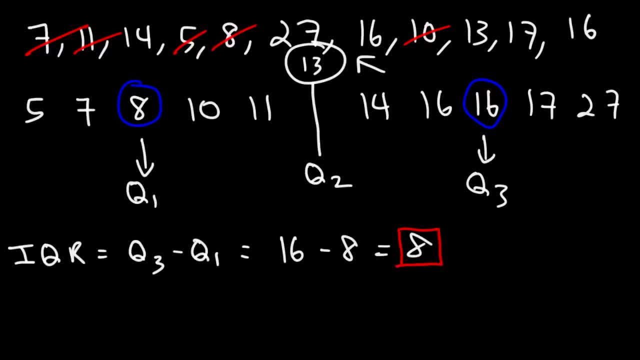 And so that's how you could find the interquartile range of a data set. Now, what about the presence of any outliers? So, looking at these numbers, do you think we have a number that really stands out? that doesn't belong? 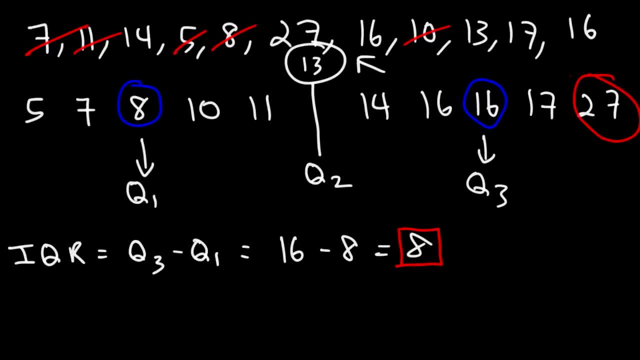 Right now, 27 appears to be very far off from all the other numbers. So do you think 27 is an outlier? Well, let's find out. So let's write down what we know. So let's write down what we know. 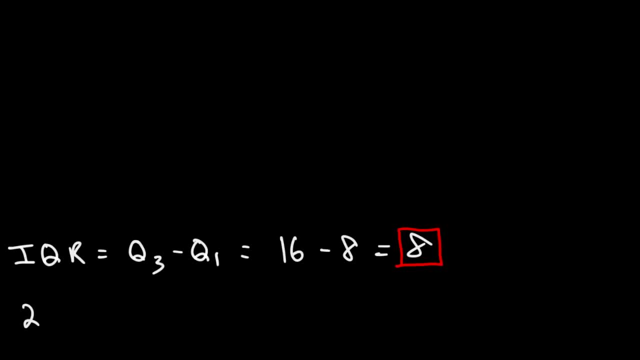 The presence of an outlier is based upon its range. It's Q1 minus 1.5 times the IQR to Q3 plus 1.5 times the IQR. So we know that Q1 is 8. And the interquartile range is also 8.. 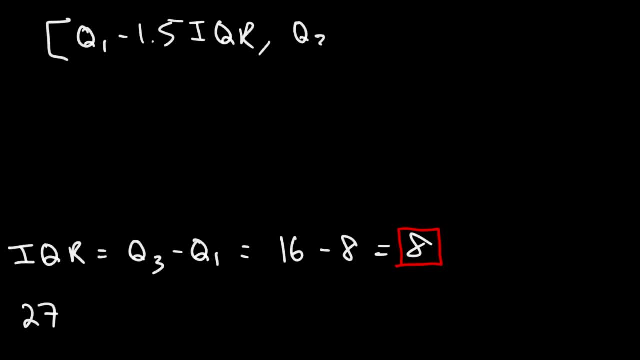 to q3 plus 1.5 times the iqr. so we know that q1 is 8, and we know that q2 is 4 and q3 is 7 And the interquartile range is also 8.. Q3 is 16.. 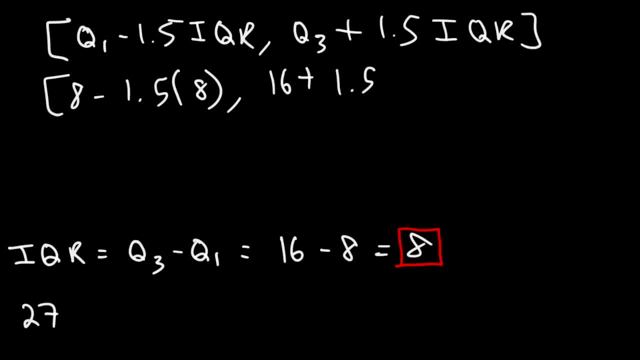 So this is going to be 16 plus 1.5 times 8.. What is 1.5 times 8?? 1 times 8 is 8.. 0.5 times 8 is 4.. 8 plus 4 is 12.. 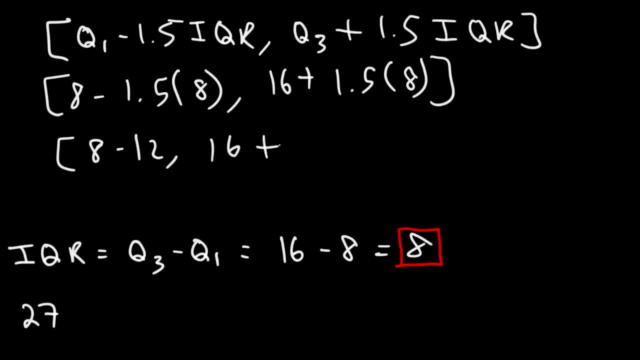 So this is going to be 8 minus 12. And this is 16 plus 12.. Now, 8 minus 12 is negative 4. And 16 plus 12 is 28.. So now, looking at what we have, 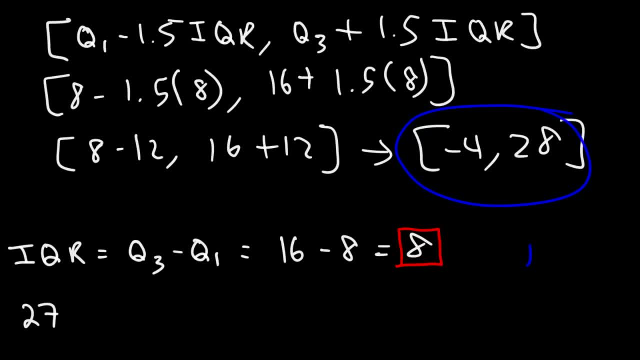 is 27 an outlier based on its range, Because 27 is between negative 4 and 28,. 27 is not an outlier. Now, if we had 29,, that would be an outlier. So now you know how to determine if a point is an outlier. 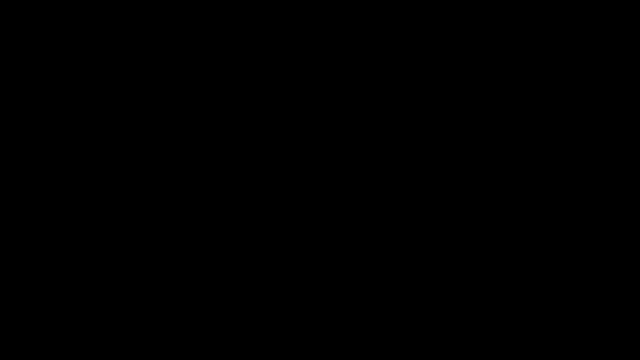 with a negative 4 or a negative 8.. And then a range. Now let's talk about how we can create a box and whisker plot. The reason why we want to talk about this now is because it's related to the values. 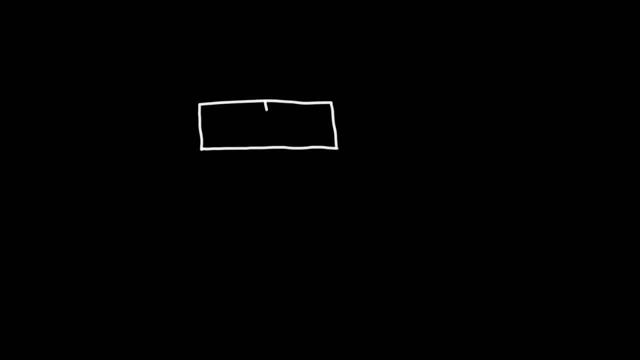 of Q1,, Q2, and Q3. So typically a box and whisker plot looks something like this: Assuming if there's no outliers, this is going to be the last outlier, The lowest value On the right we're going to have. 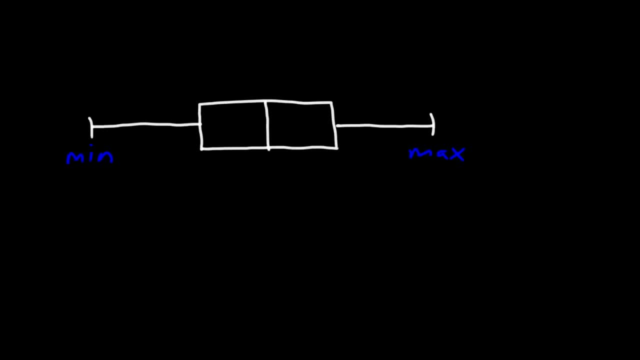 the highest value or the maximum. And then this line here represents the value of the first quartile, which is the 25th percentile. In the middle we have Q2, the second quartile, which is the 50th percentile. 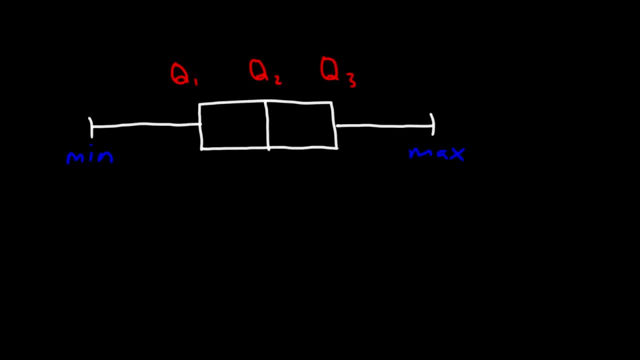 And then this is Q3, the 75th percentile, And so that's the basic shape of a box and whisker plot. Now, what about if we have an outlier? Let's say, if we have one to the right, Then this will no longer be the maximum. 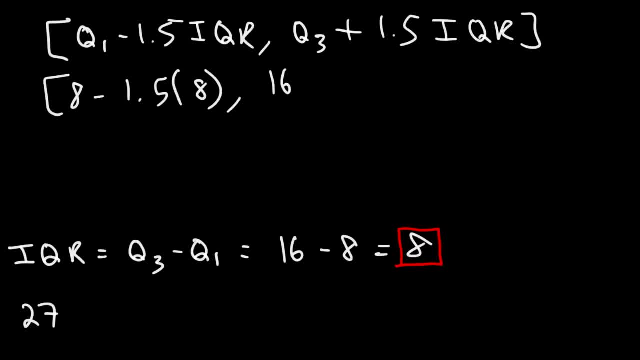 Q3 is 16.. So this is going to be 16 plus 1.5 times 8.. What is 1.5 times 8?? 1 times 8 is 8.. 0.5 times 8 is 4.. 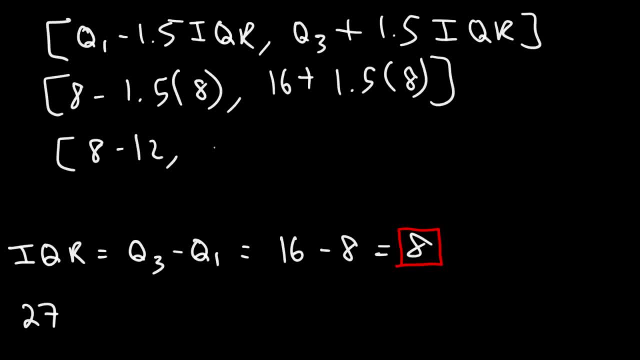 8 plus 4 is 12.. So this is going to be 8 minus 12. And this is 16 plus 12.. Now, 8 minus 12 is negative 4. And 16 plus 12 is 28.. 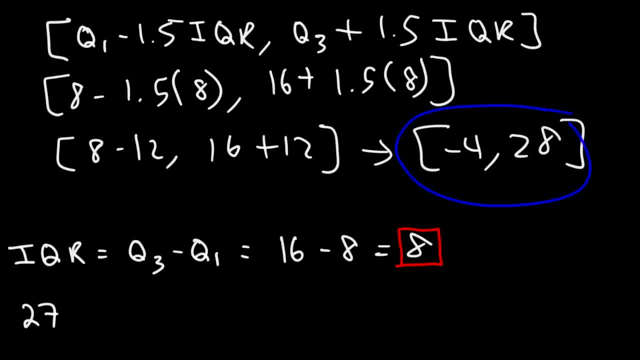 So now, looking at what we have, is 27 an outlier based on its range, Because 27 is between negative 4 and 28,. 27 is not an outlier. Now, if we had 29,, that would be an outlier. 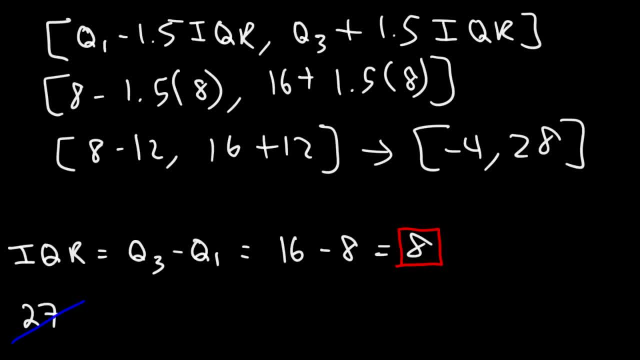 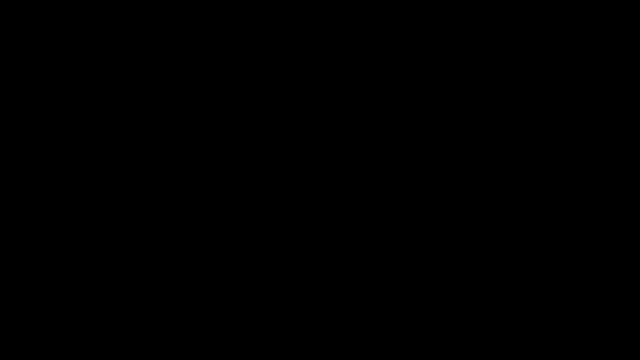 So now you know how to determine if a point is an outlier within a range. Now let's talk about how we can create a box and whisker plot. The reason why we want to talk about this now is because it's related to the values of 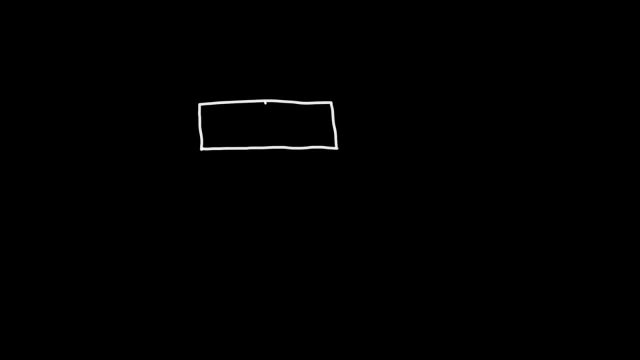 Q1,, Q2, and Q3.. So typically a box and whisker plot looks something like this: Assuming, if there's no outliers, this is going to be the lowest value, On the right, we're going to have the highest value. 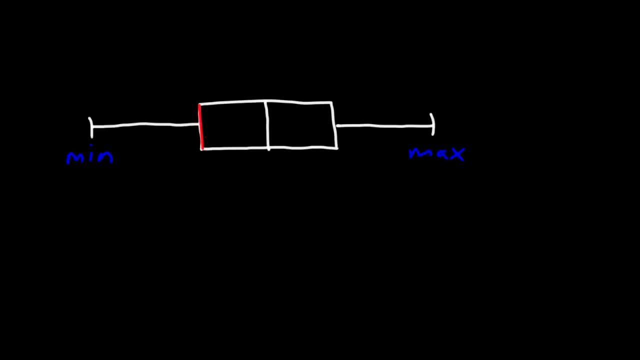 or the maximum, And then this line here represents the value of the first quartile, which is the 25th percentile. In the middle we have Q2, the second quartile, which is the 50th percentile, And then this is Q3,. 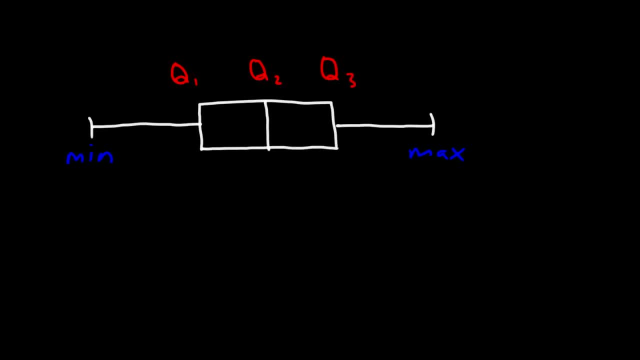 the 75th percentile, And so that's the basic shape of a box and whisker plot. Now what about if we have an outlier? Let's say, if we have one to the right, Then this will no longer be the maximum. 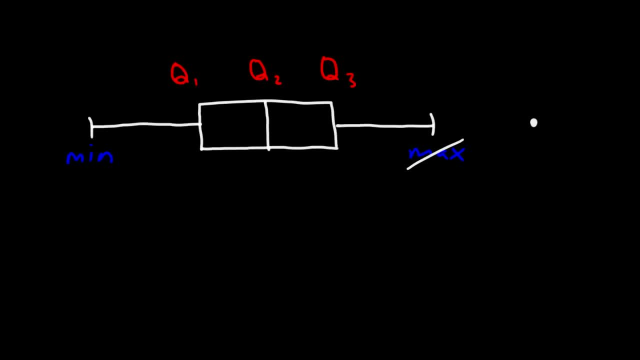 The outlier is shown as a point. It's outside of the box and whisker plot. Now, if it's on the left side, this will no longer be the minimum and that will be the outlier there. So let's work on an example. 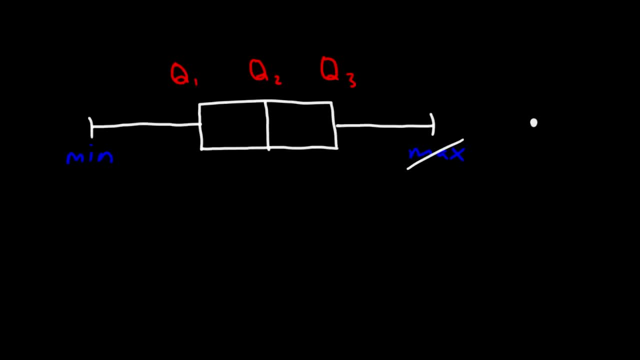 The outlier is shown as a point. It's outside of the box and whisker plot. Now, if it's on the left side, this will no longer be the minimum and that will be the outlier there. So let's work on an example. 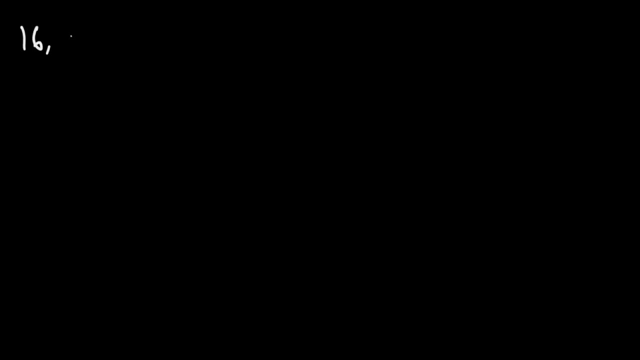 Let's say we have the numbers 16,, 18,, 28,, 13,, 50,, 31,, 25,, 22,, and let's say another 18,, 23,, 29,, 31, and 38.. 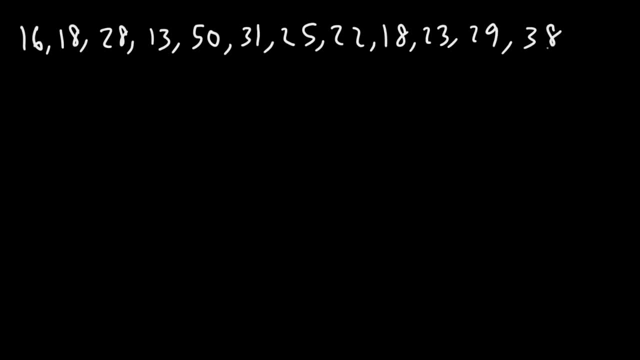 Actually I wrote down 31 already. Let's make this 38. So we have 12 numbers. Using this data set, go ahead and find the interquartile range Q1, Q2, Q3.. Identify the presence. 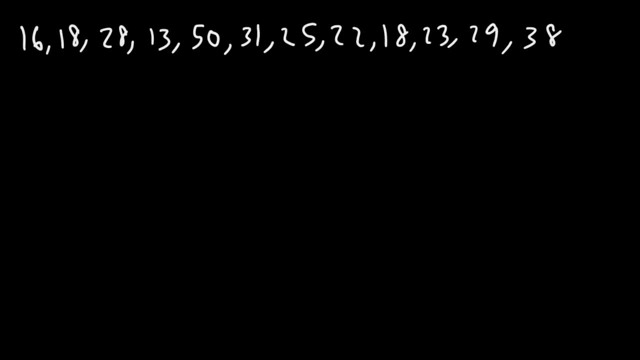 of any outliers and then, using all of that information, construct a box and whisker plot. Feel free to pause the video if you want to try that yourself Now. the first step, as always, is to write the numbers in increasing order. 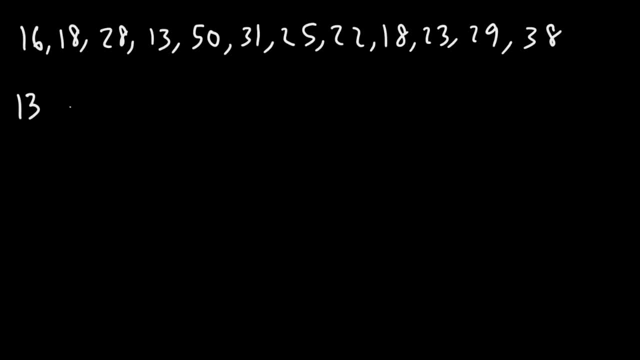 So we have 13,, 16,, 18.. So let's get rid of those numbers. And then there's another 18, and then 22, 23.. Next is 25,, and then 22,, 28,, 29,. 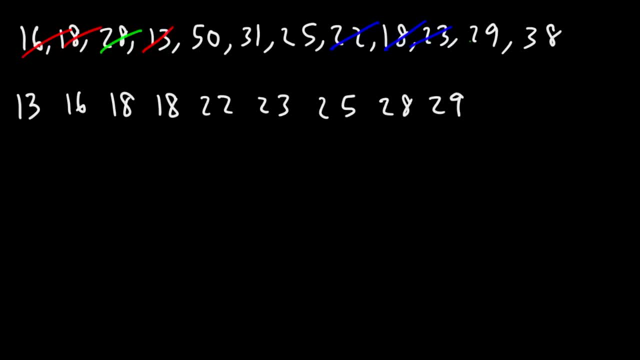 and then the last three are 31,, 38, and 50. Now what I like to do is break up the data into four quarters or four sections. Now, because we have an even number of data points, we have a total of 12, we can put. 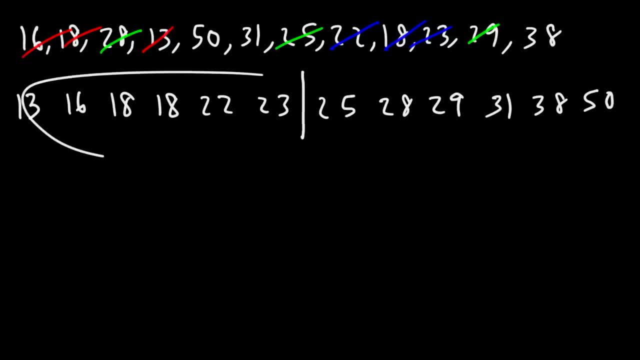 a line right in the middle. So now this is the lower half of the data set, and here we have the upper half. So let's determine the median for the entire data set, Because it's even. we can't just immediately identify the median. 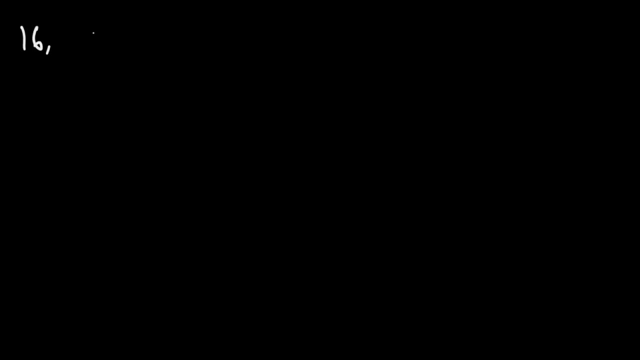 Let's say we have the numbers 16,, 18,, 68,, 13,, 50,, 31,, 25,, 22,, and let's say another 18,, 23,, 29,, 31, and 38.. 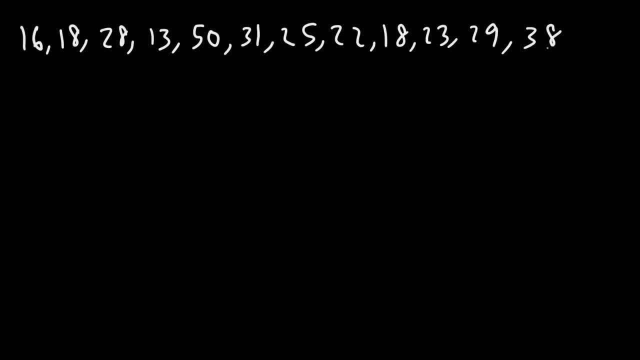 Actually I wrote down 31 already. Let's make this 38. So we have 12 notes, so we have 12 numbers. Using this data set, go ahead and find the interquartile range Q1, Q2, Q3.. 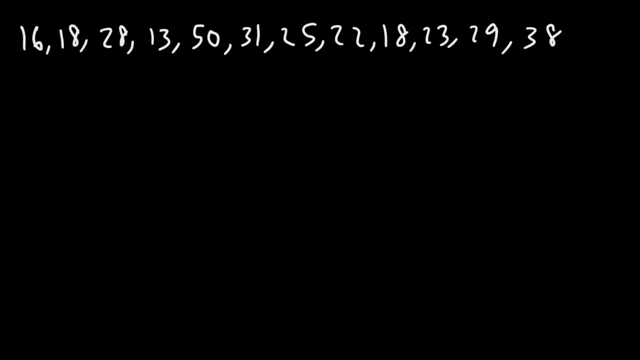 Identify the presence of any outliers and then, using all of that information, construct a box and whisker plot. Feel free to pause the video if you want to try that yourself Now. the first step, as always, is to write the numbers in. 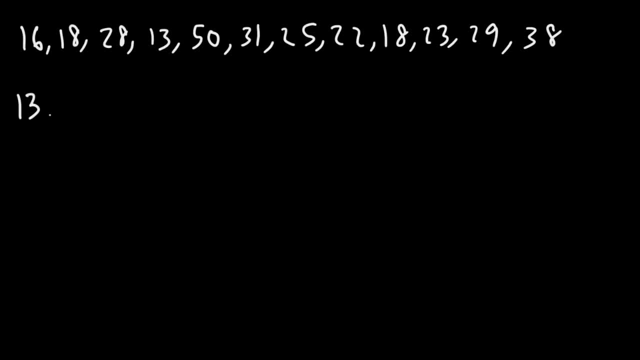 increasing order. So we have 13,, 16,, 18,, so let's get rid of those numbers. and then there's another 18,, and then 22,, 23,, next is 25,, and then 28,, 29,. 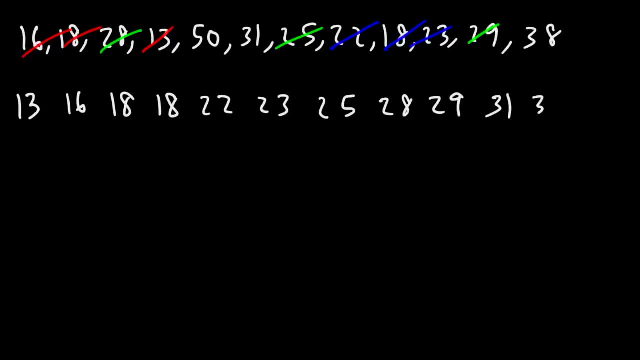 and then the last three are 31,, 38, and 50. Now what I like to do is break up the data into four quarters or four sections. Now, because we have an even number of data points. we have a total of 12,. 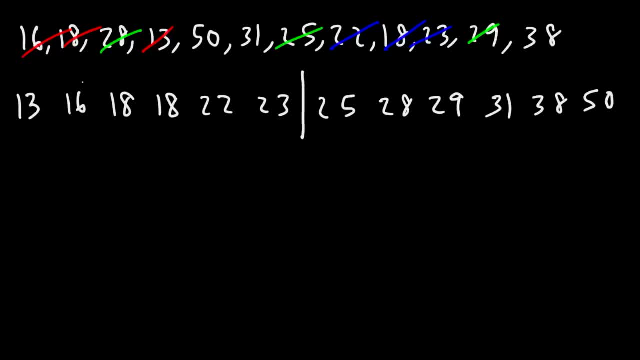 we can put a line right in the middle. So now this is the lower half of the data set, and here we have the upper half. So let's determine the median for the entire data set, Because it's even. we can't just immediately. 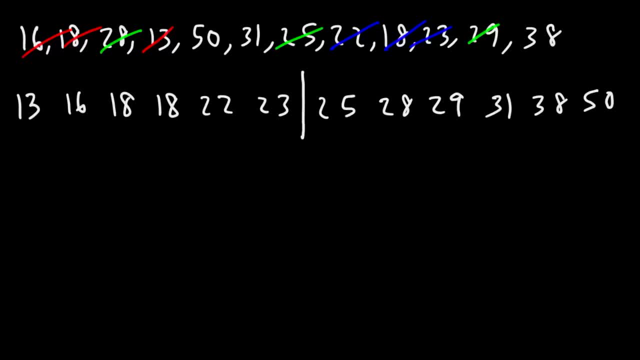 identify the median. The median is going to be an average of these two numbers. If we eliminate the first two and then the next two and so forth, we will eventually get to these two numbers. So what is the median between, or what is the average between, 23 and 25?? 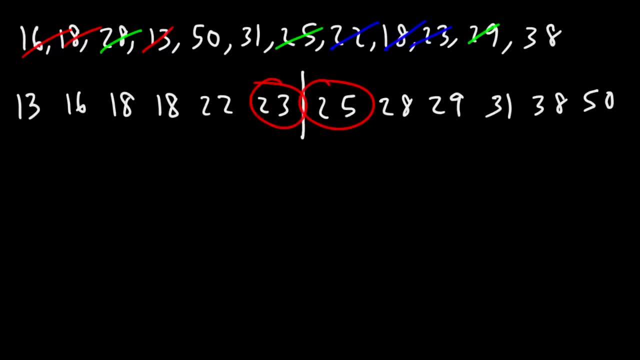 The median is going to be an average of these two numbers. If we eliminate the first two and then the next two and so forth, we will eventually get to these two numbers. So what is the median between, or what is the average between, 23 and 25?? 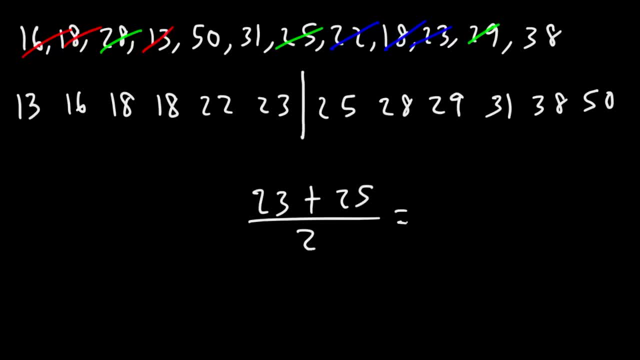 So if you add up those two numbers and divide it by two, you're just going to get the midpoint of 23 and 25, which is 24.. So 24 is the second quartile. This is the Q2 value. 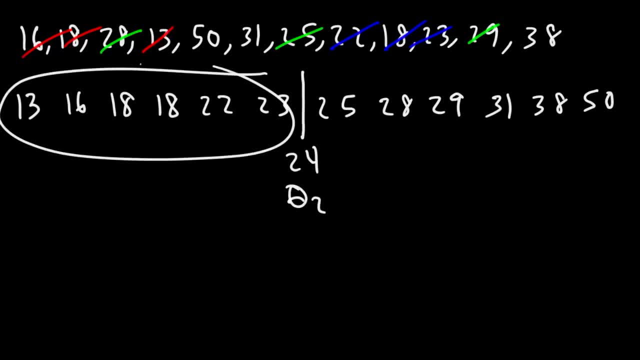 Now let's focus on the lower half of the data. What is the median of the lower half of the data? So notice that we have six data points in that section And, because it's even, the median is going to be an average of these two numbers. 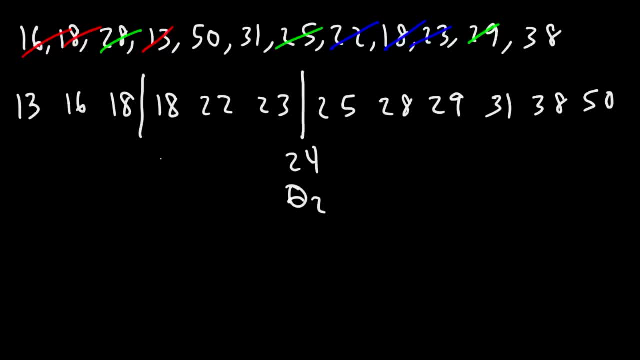 So let's put a line there. The average of 18 and 18 is 18.. So that's our Q1 value. Now, what about the median of the upper half of the data? So, because we have six numbers here, we're going to put a line right in the middle. 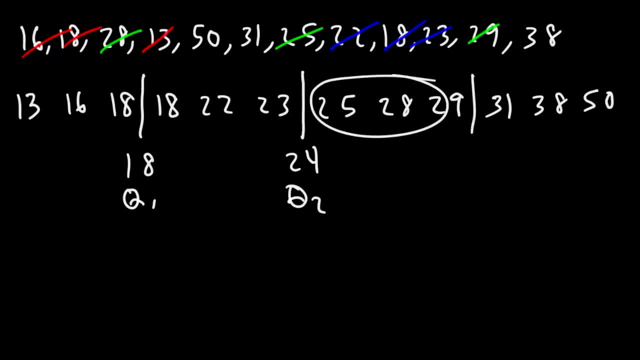 So we have three on the left, three on the right, And the median is simply going to be the average of these two numbers. The average of 29 and 31 is the number in the middle, which is 30. And so this is why I like to use these lines here. 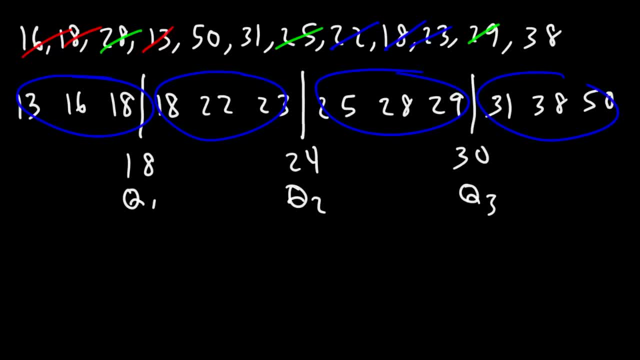 So now we have three numbers in each of the four sections of our data. So, now that we know Q1,, Q2, and Q3,, what is the interquartile range? What's our IQR value? The IQR is the difference between the third quartile and the first quartile. 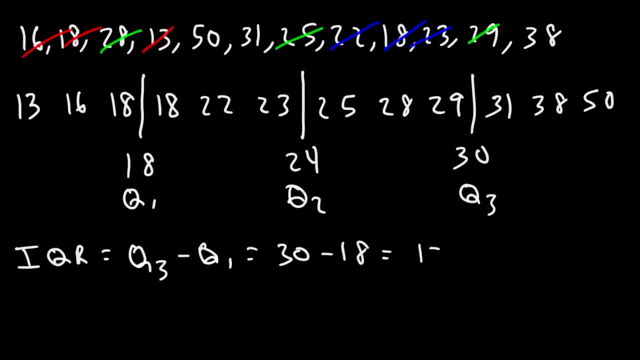 So it's going to be 30 minus 18, which is 12 in this example. So now that we have that, our next step is to determine if we have any outliers in this problem. So remember, this is what we need. 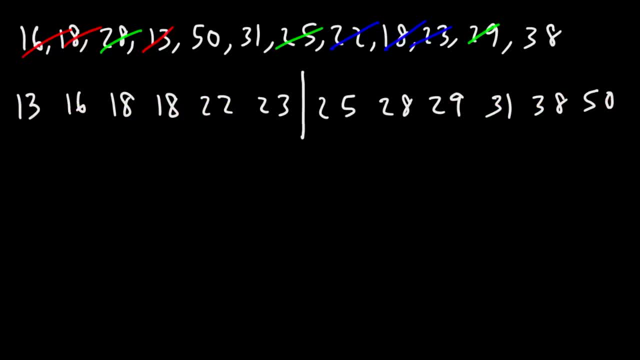 So if you add up those two numbers and divide it by two, you're just going to get the midpoint of 23 and 25, which is 24.. So 24 is the second quartile. This is the Q2 value. 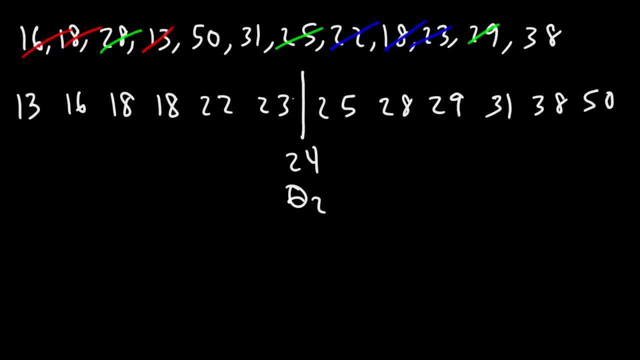 Now let's focus on the lower half of the data. What is the median for the entire data set? What is the median of the lower half of the data? So notice that we have six data points in that section And, because it's even, 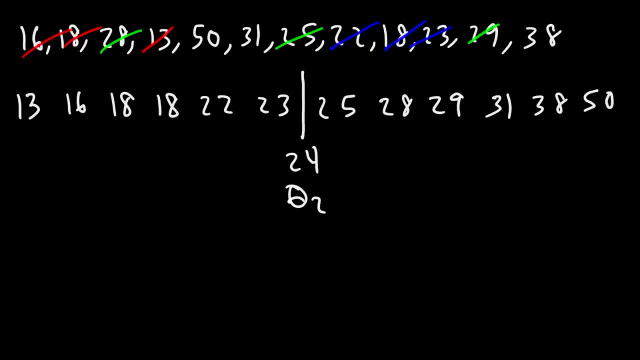 the median is going to be an average of these two numbers, So let's put a line there. The average of 18 and 18 is 18.. So that's our Q1 value. Now what about the median of the upper half of the data? 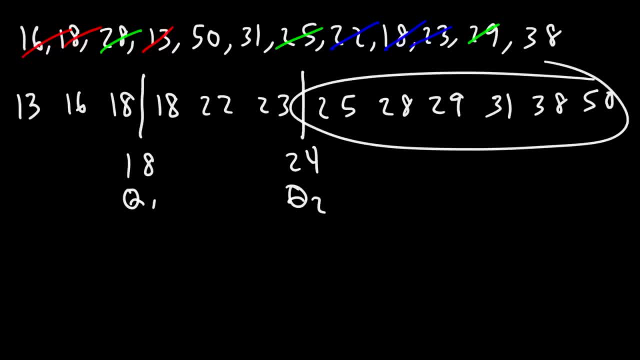 So because we have six numbers here and right in the middle, so we have three on the left, three on the right And the median is simply going to be the average of these two numbers. The average of 29 and 31 is the number in the middle. 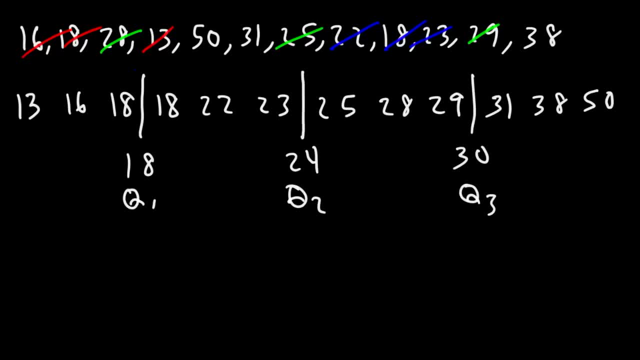 which is 30. And so this is why I like to use these lines here. So now we have three numbers in each of the four sections of our data. So now that we know Q1,, Q2, and Q3,, what is the? 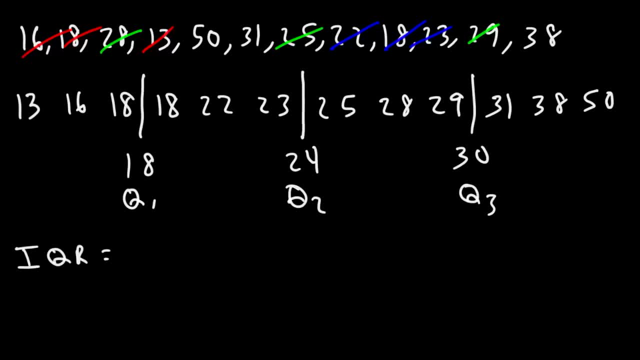 interquartile range. What's our IQR value? The IQR is the difference between the third quartile and the first quartile, So it's going to be 30 minus 18, which is 12 in this example. So now that we have, 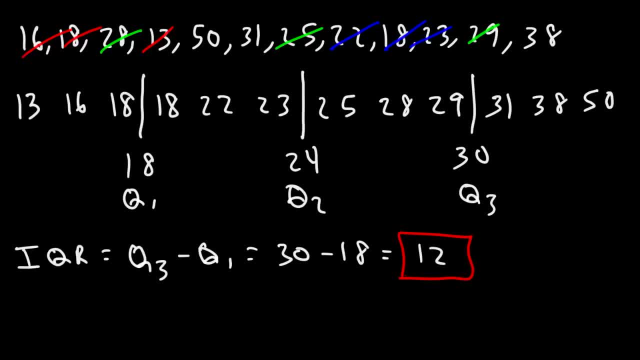 that our next step is to determine if we have any outliers in this problem. So remember, this is what we need. We need to create a range. The lowest point of it will be Q1 minus 1.5 times the IQR. 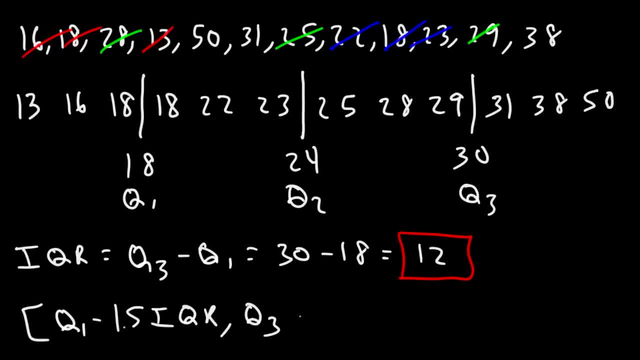 And the highest point of the range will be Q3 plus 1.5 times the IQR. Now I'm going to have to get rid of a few things, So let's write down the information that is important: Q1 is 18.. 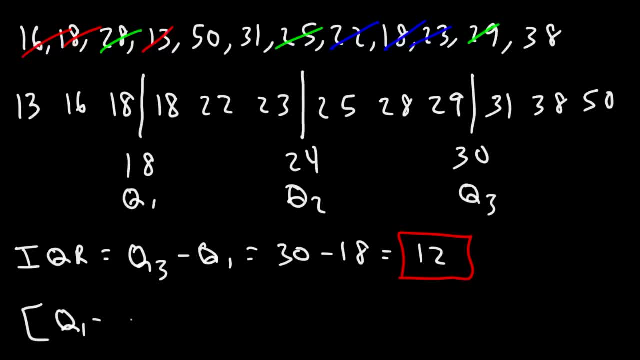 We need to create a range. The lowest point of it will be Q1 minus 1.5 times the IQR, And the highest point of the range will be Q3 plus 1.5 times the IQR. Now I'm going to have to get rid of a few things. 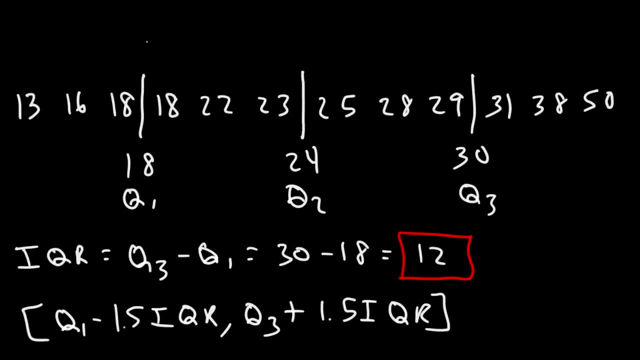 So let's write down the information that is important. So Q1 is 18.. Q2 is 24.. Q3 is 30. Our minimum, the lowest value, is 13.. And the maximum, our highest value, is 50.. 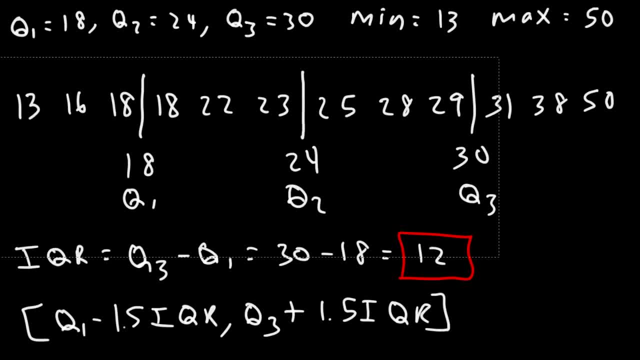 So let's keep that in mind. So now I can get rid of this. You may want to write that down, just in case we need to go back to it, And I can also get rid of this too. So let's plug in what we know into this expression. 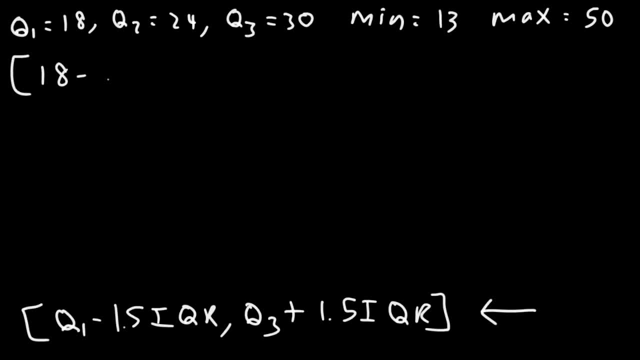 So Q1 is 18.. And the IQR- I've got to write that down again- That was 12.. It was 30 minus 18, which is 12.. So this is going to be 18 minus 1.5 times 12.. 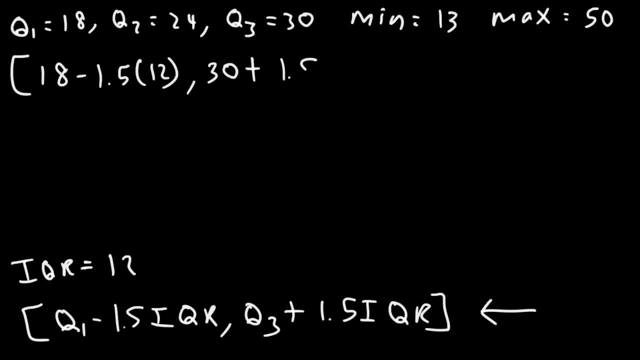 And then Q3 is 30 plus 1.5 times 12.. Now, what is 1.5 times 12?? So it's basically 12 plus half of 12, which is 6.. 12 plus 6 is 18.. 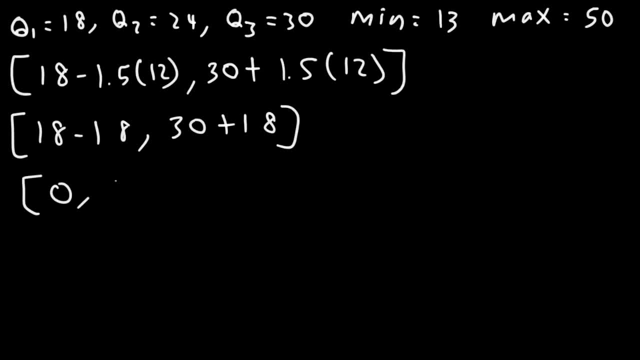 18 minus 18 is 0.. 30 plus 18 is 48.. So do we have any outliers? Are there any numbers outside of this range? And it turns out that there is The maximum 50, is not between 0 and 48.. 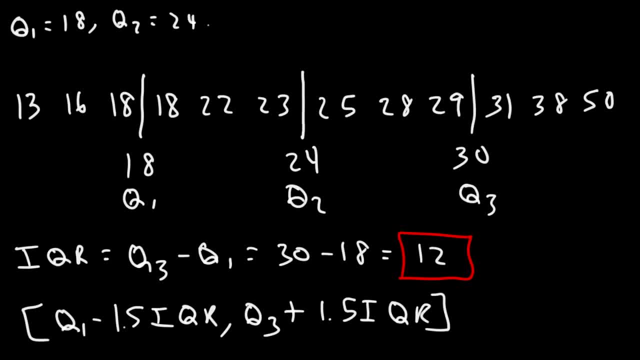 Q2 is 24.. Q3 is 30. Our minimum, the lowest value, is 13.. And the maximum, our highest value, is 50. So let's keep that in mind. So now I can get rid of this. You may want to write that down. 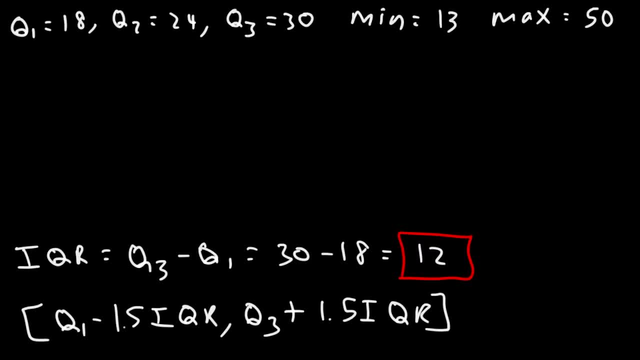 just in case we need to go back to it- And I can also get rid of this too, So let's plug in what we know into this expression. So Q1 is 18.. And the IQR? I got to write that down again. 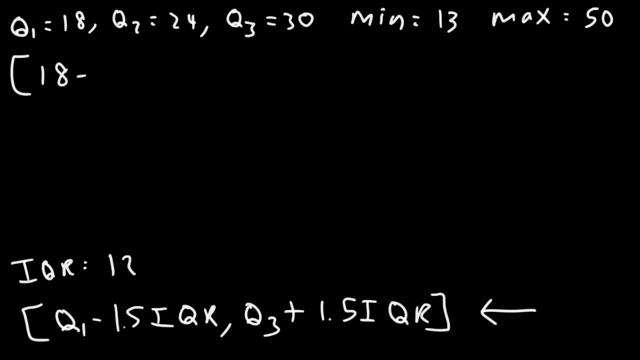 That was 12.. It was 30 minus 18, which is 12.. So this is going to be 18 minus 1.5 times 12.. And then Q3 is 30 plus 1.5 times 12.. Now what is 1.5 times 12?? 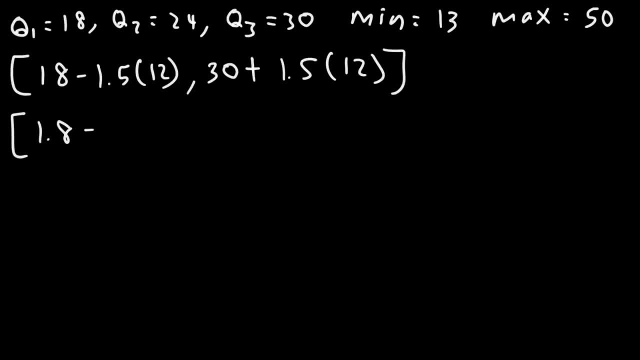 So it's basically 12 plus half of 12, which is 6.. 12 plus 6 is 18.. 18 minus 18 is 0.. 30 plus 18 is 48.. So do we have any outliers? Are there any numbers? 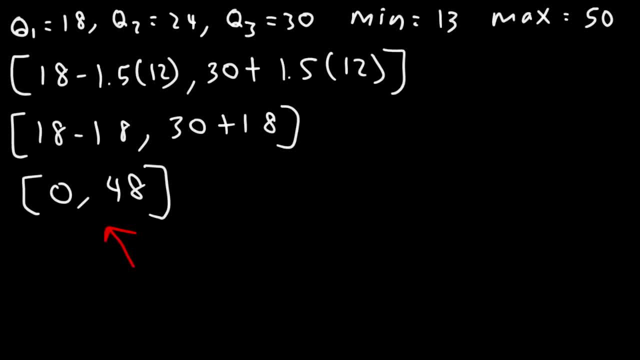 outside of this range And it turns out that there is The maximum 50, is not between 0 and 48. So this is an outlier. Now, going back to our original data, I'm just going to rewrite it so you can see everything. 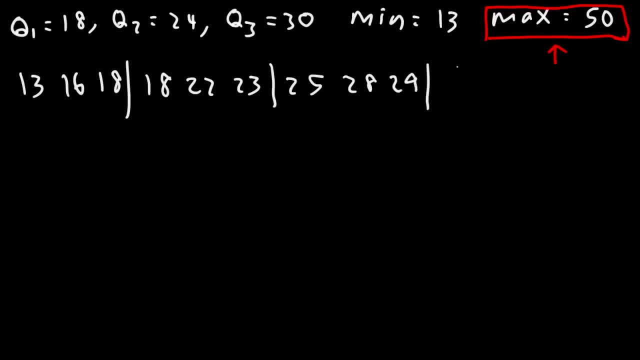 This is what we had. So now, at this point, let's go ahead and let's make a number line. So 0 is going to be our lowest point and we're going to go up to 50.. So let's go by 10s. 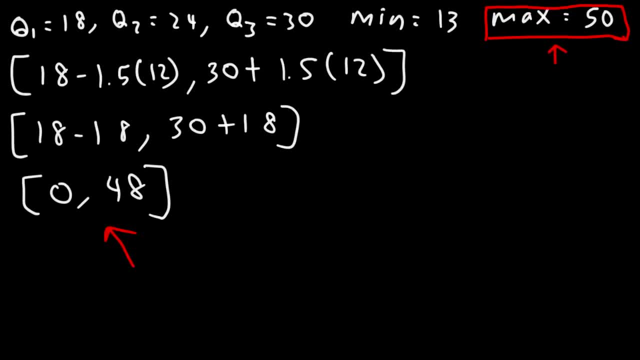 So this is an outlier. Now, going back to our original data, I'm just going to rewrite it so you can see everything. This is what we had. So now, at this point, let's go ahead and let's make a number line. 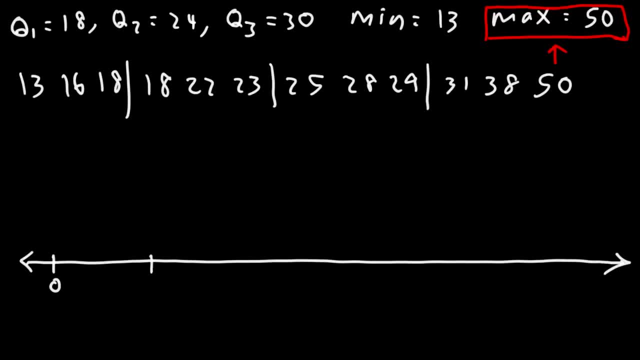 So 0 is going to be our lowest point And we're going to go up to 50.. So let's go by 10s. Now let's put a mark in the middle to represent the 5s. So let's begin by drawing a box. 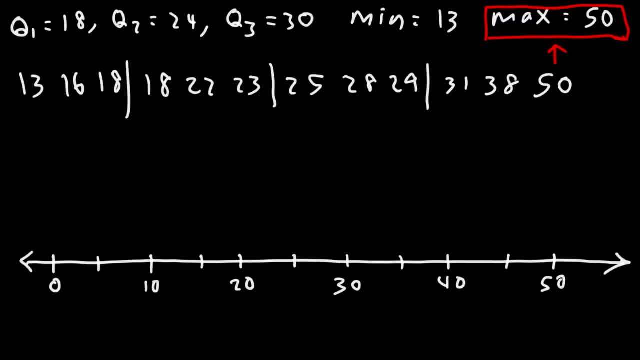 So we need to draw a box ranging from Q1 to Q3.. So that's going to start at 18.. And this is basically a rough estimate. It's not going to be perfect And the end of the box will be at 30.. 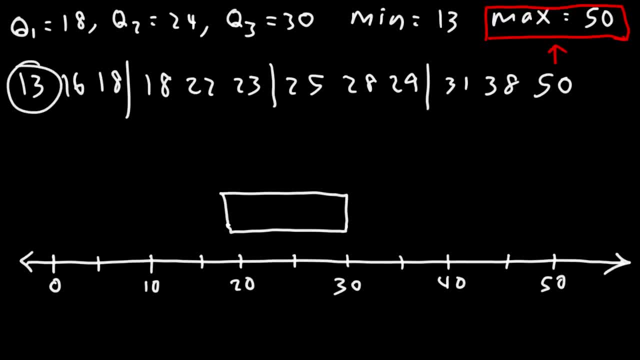 Now, 13 is the minimum, which is approximately around that area. So that's the left side of the box, And 50 is the maximum. but that's an outlier, So we're going to just put a point at 50.. 38.. 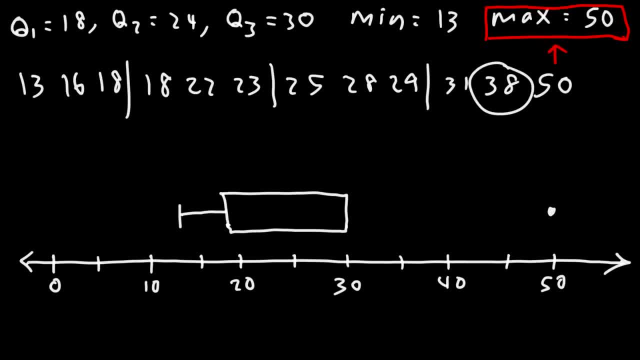 38 is the second highest, which is not an outlier. So that's going to be part of the box and whisker plot And so 38 is in this region. So we're going to say it's over there Now. Q1 is 18.. 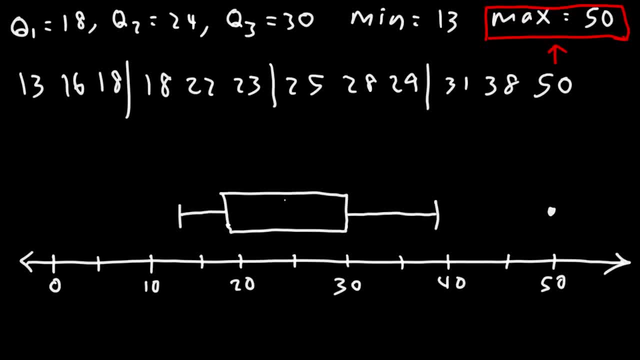 Q3 is 30. But we also need to write where Q2 is. Q2 is 24,, which is around here. So this is Q1.. That's 18,, Q2, and Q3.. So the left of the box represents the interquartile range, which is 12.. 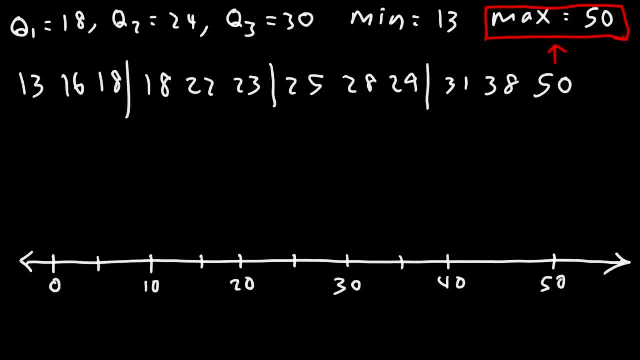 Now let's put a mark in the middle to represent the 5s. So let's begin by drawing a box. So we need to draw a box ranging from Q1 to Q3. So that's going to start at 18.. And this is basically a rough estimate. 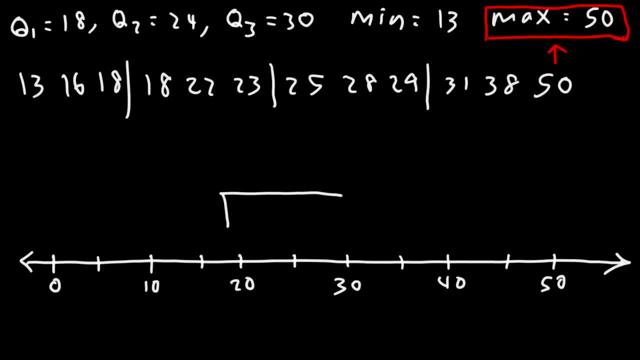 It's not going to be perfect And the end of the box will be at 30.. Now, 13 is the minimum, Which is approximately around that area. So that's the left side of the box And 50 is the maximum. but that's an outlier. 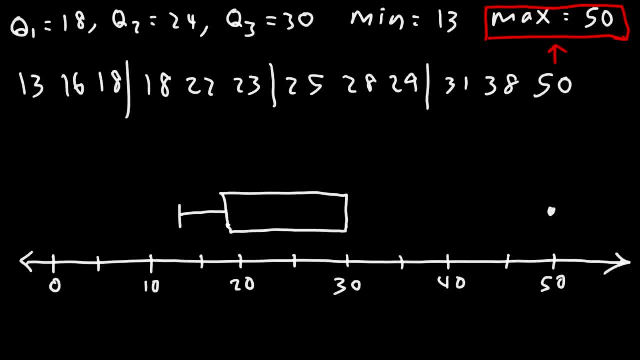 So we're going to just put a point at 50.. 38 is the second highest, which is not an outlier, So that's going to be part of the box and whisker plot. And so 38 is in this region, So we're going to say it's over there. 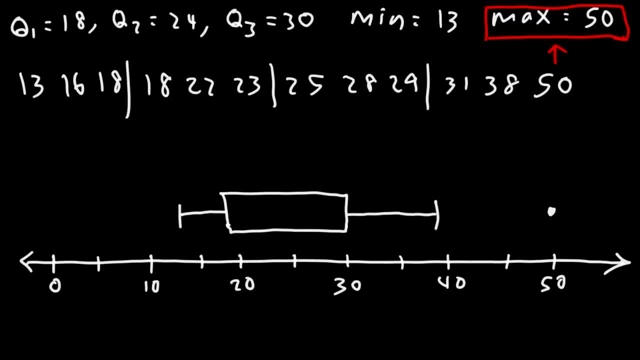 Now Q1 is 18,, Q3 is 30, but we also need to know where Q2 is. Q2 is 24, which is around here, So this is Q1.. That's 18,, Q2, and Q3. 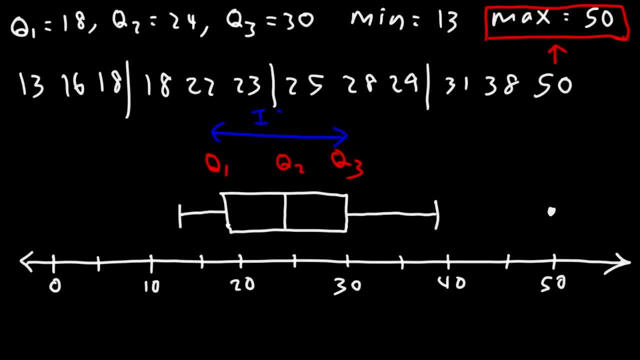 So the left of the box represents the interquartile range, Which is 12.. That's 30 minus 18.. And so here is the minimum, and this is the maximum Which is the outlier. But that's how you can construct a box, and 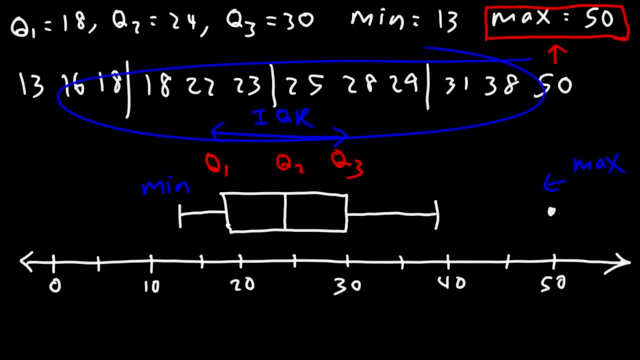 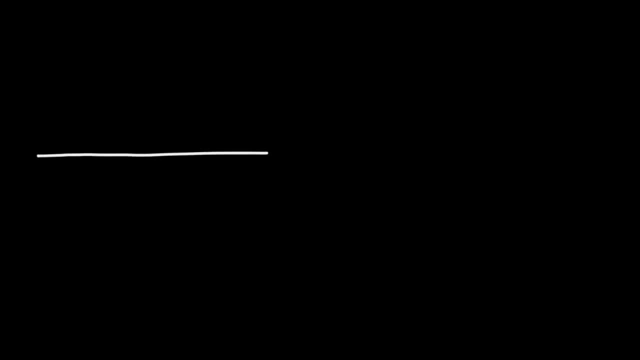 whisker plot, given a data set. Now the next topic we need to talk about is skewness. So let's say we have this representation of our data And notice that it is symmetrical. This line represents the median And if you have a data that 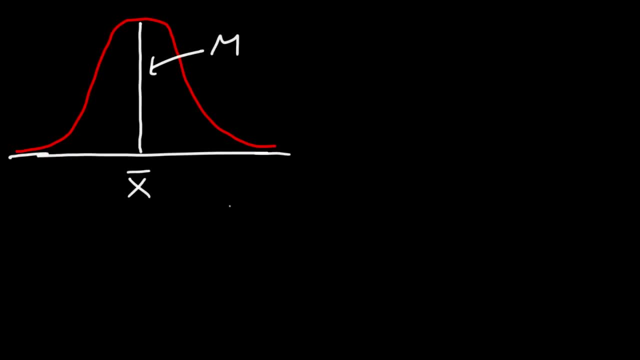 is perfectly symmetrical. the mean- this is the sample mean. it's going to be equal to the median. Now the box and whisker plot will look something like this: Q2 is going to be right in the middle of Q1 and Q3.. 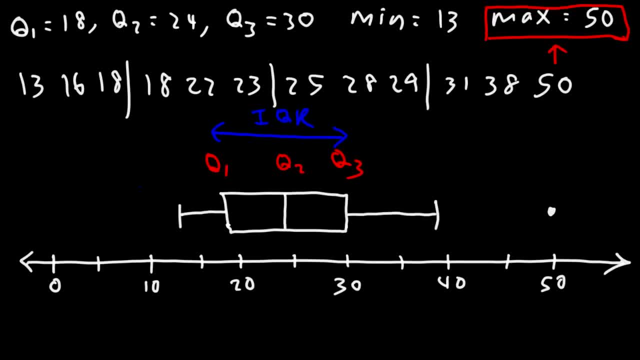 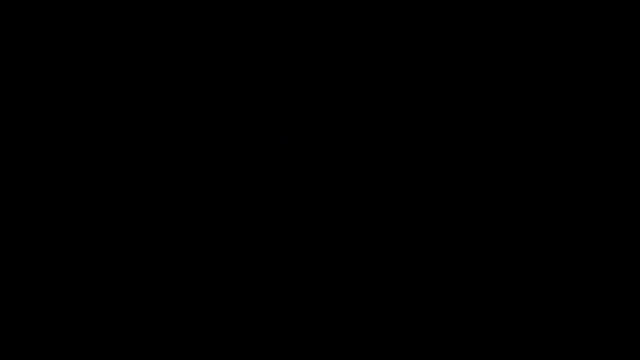 That's 30 minus 18.. And so here is the minimum, And this is the maximum, which is the outlier, But that's how you can construct a box and whisker plot, given a data set. Now, the next topic we need to talk about is skewness. 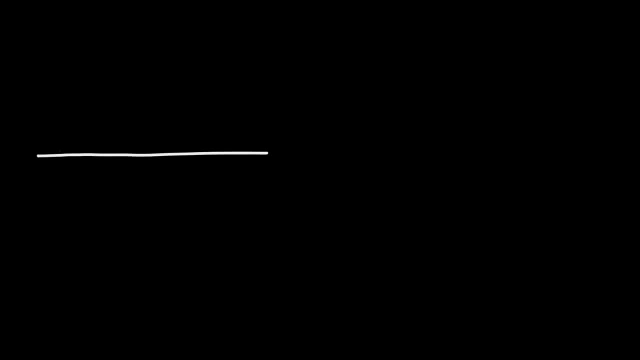 So let's say we have this representation of our data And notice that it is symmetrical. This line represents the median And if you have a data that is perfectly symmetrical, the mean- this is the sample mean- it's going to be equal to the median. 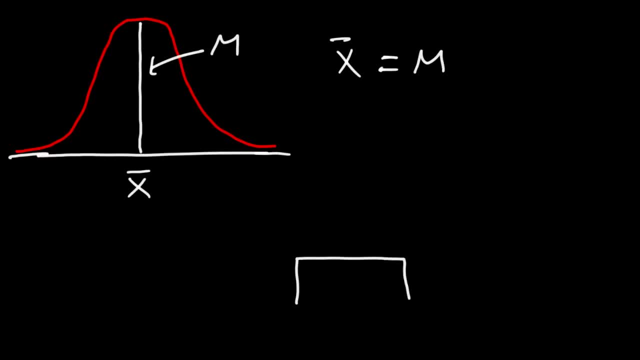 Now the box and whisker plot will look something like this: Q2 is going to be right in the middle of Q1 and Q3.. So notice that the box plot is evenly distributed. The left side is the same as the right side and left. 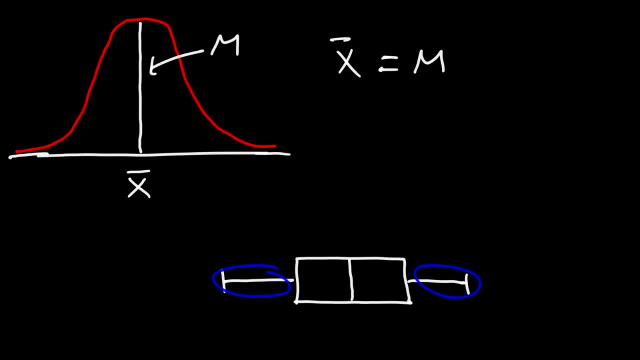 And also these lines are equal in length, So that represents a symmetric distribution. Now, what if it's not symmetrically distributed? What's going to happen in that case? There are two possibilities: The data can be skewed to the right, or it can be skewed to the left. 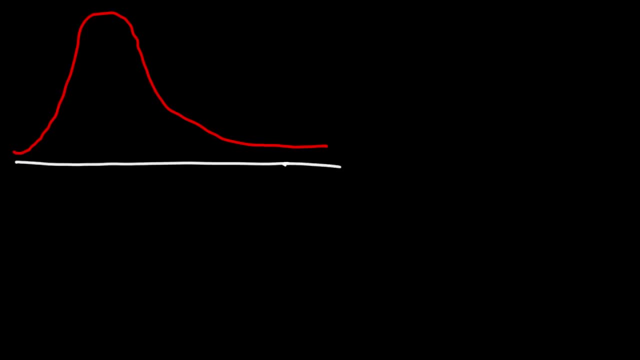 So which one would you say this particular shape represents? Would you say it's skewed to the right or skewed to the left? Notice that we have a tail that extends towards the right. So this particular data or this graph, we'd say that it's skewed to the right. 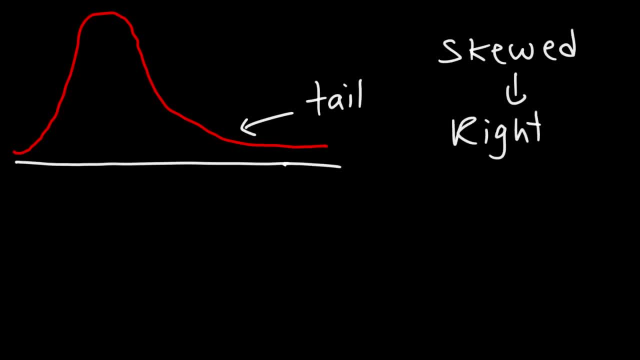 Now, what is the relationship between the sample mean and the median in this case? So what is the relationship between the sample mean and the median in this case? So the median, the middle portion of the data, will be somewhere in this region And the sample mean will be to the right of the median, since it's skewed to the right. 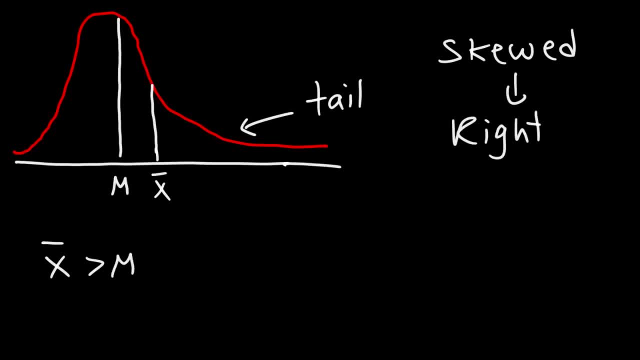 So the mean will be greater than the median in this case. By the way, whenever you have a shape that's skewed to the right, some textbooks will refer to this as a positive skew, And it makes sense because positive numbers on a number line. 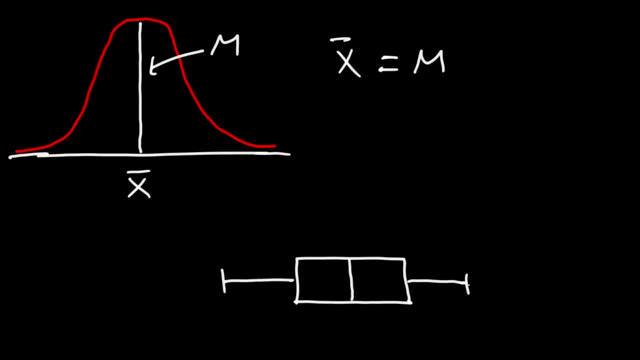 So notice that the box and whisker plot is evenly distributed. The left side is the same as the right side and left, And also these lines are equal and left. So that represents a symmetric distribution. Now, what if it's not symmetrically distributed? 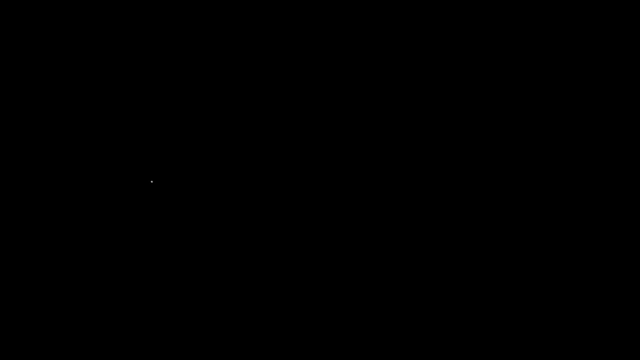 What's going to happen in that case? There are two possibilities: The data can be skewed to the right or it can be skewed to the left. So which one would you say this particular shape represents? Would you say it's skewed to the right or skewed to the left? 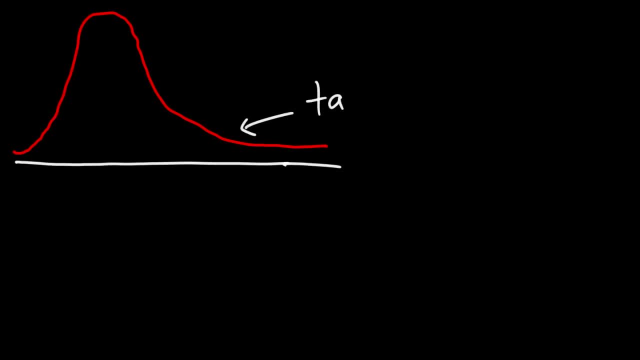 Notice that we have a tail that extends towards the right. So this particular data or this graph, we say that it's skewed to the right. Now, what is the relationship between the sample mean and the median in this case? So the median, the middle portion of the data. 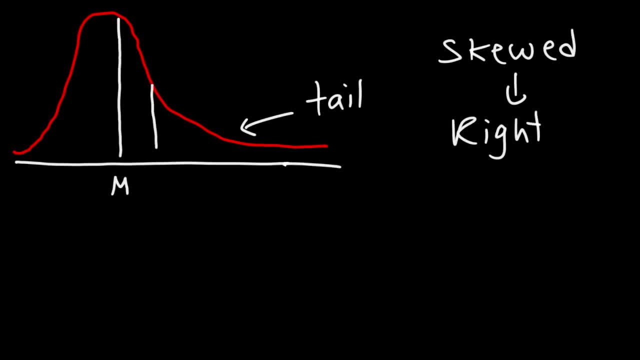 will be somewhere in this region, And the sample mean will be to the right of the median, since it's skewed to the right, So the mean will be greater than the median in this case. By the way, whenever you have a shape that's skewed to the right, 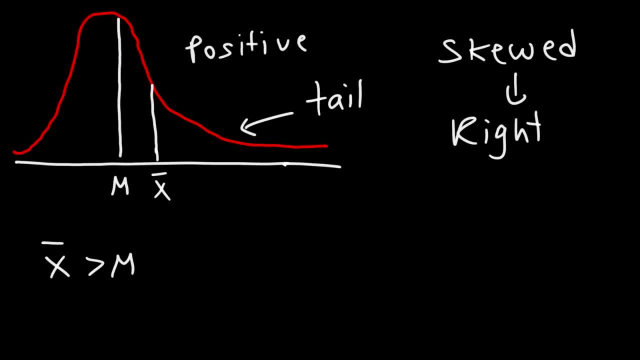 some textbooks will refer this as a positive skew, And it makes sense because positive numbers on a number line will be on the right side. Now you need to be familiar with the box and the whisker plots for this type of distribution. So here's one example. 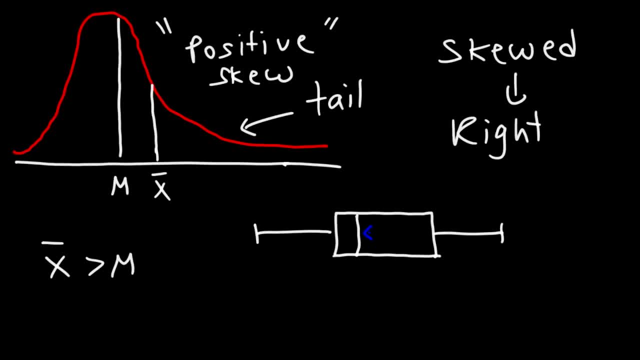 Notice that the right side of the box is longer than the left side. So this tells us that Q3 minus Q2 is greater than Q2 minus Q1.. And so in that case, looking at the box and whisker plot, you can see. 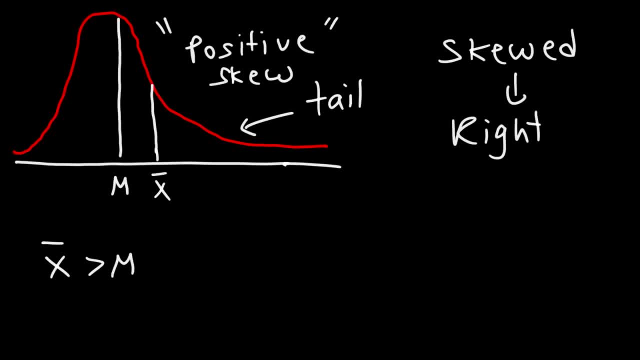 will be on the right side. Now you need to be familiar with the box and the whisker plots for this type of distribution. So here's one example. Notice that the right side of the box is longer than the left side. So this tells us that Q3 minus Q2 is greater than Q2 minus Q1. 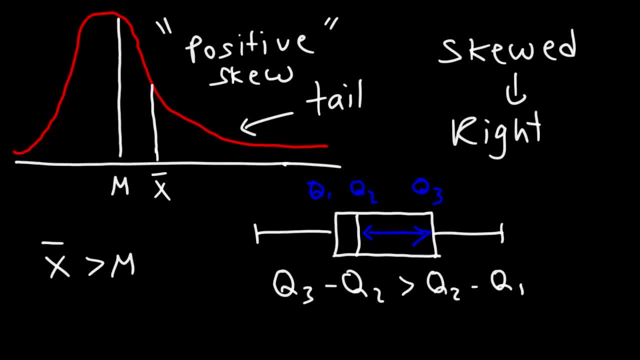 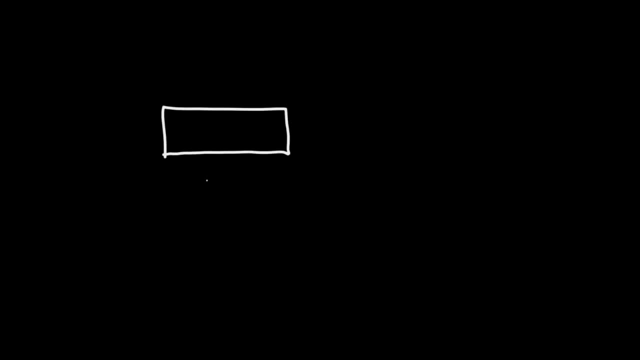 And so in that case, looking at the box and whisker plot, you can see that it's skewed to the right. Now, sometimes these two boxes may be equal in length. Nevertheless, this side might be longer than this side. So even if the boxes are of the same length, 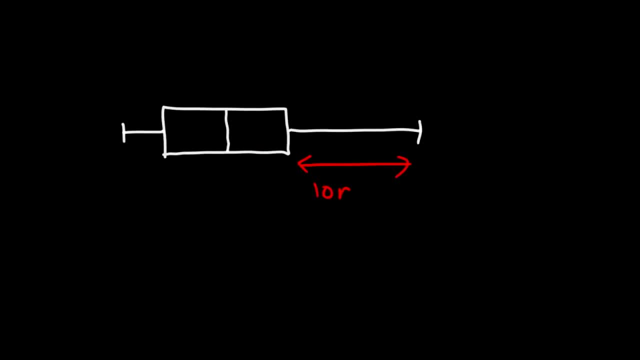 if this side is longer, it will also be skewed to the right. Now what about if it's skewed to the left? In this case, the graph is going to look something like this: Let me try that again. So notice that the tail is on the left side. 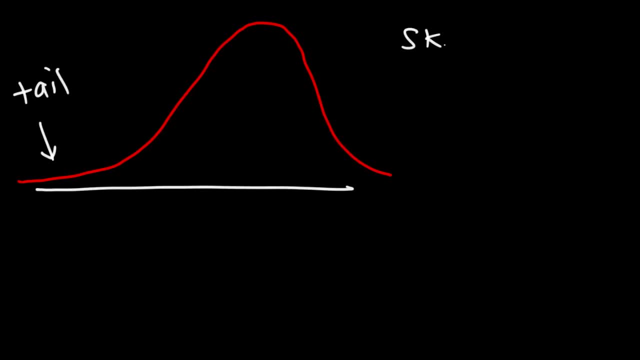 So in this case we have a negative skew, Or we could say that it's skewed to the left. Now the median will be somewhere in this region And the mean is going to be to the left of the median, Since it's skewed to the left. 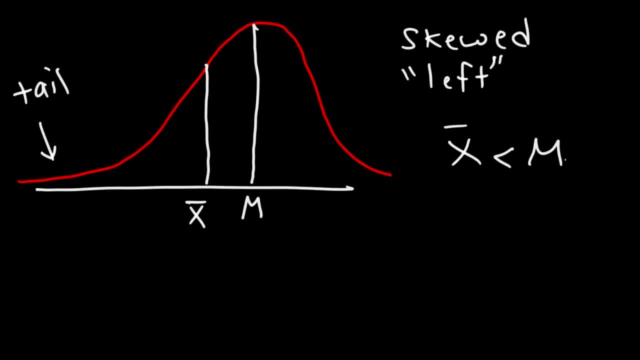 So the sample mean is less than the median. Now, how can we represent this using a box plot? Well, here's one possibility. So in this case, Q2 will be closer to Q3 in the box plot. So, as you can see, the left side is longer than the right side. 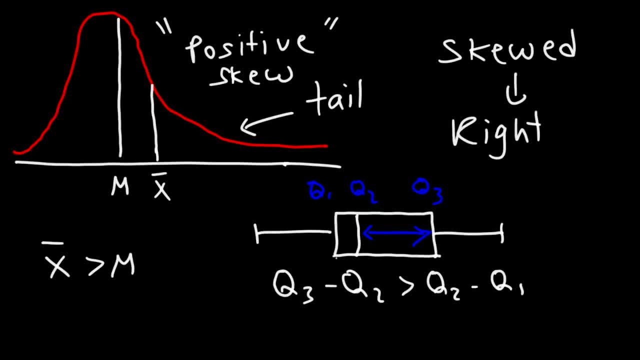 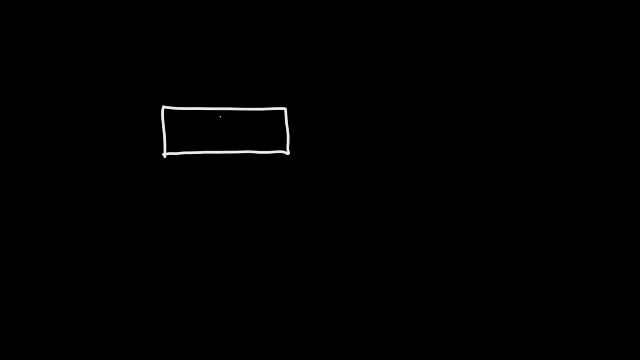 that it's skewed to the right. Now. sometimes these two boxes may be equal in length. Nevertheless, this side might be longer than this side. So even if the boxes are of the same length, if this side is longer it will. 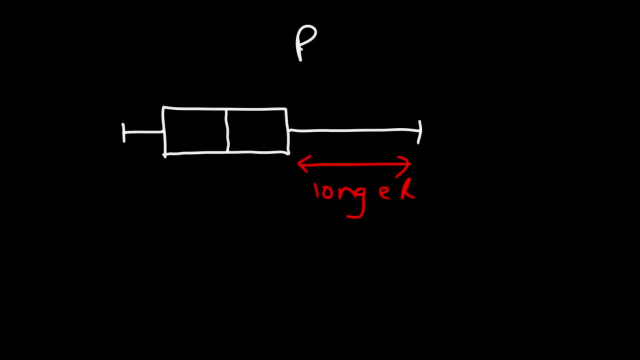 also be skewed to the right. Now what about if it's skewed to the left? In this case, the graph is going to look something like this: Let me try that again. So notice that the tail is on the left side. So in this case we have a negative skew. 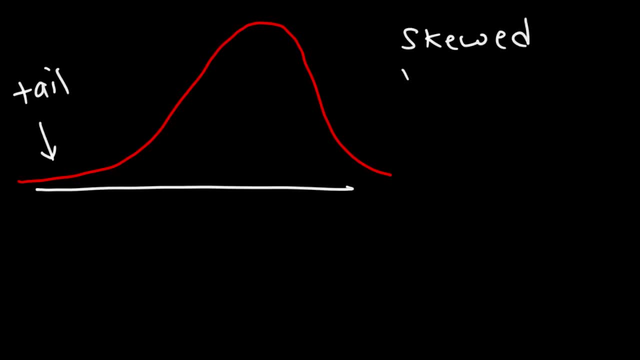 Or we could say that it's skewed to the left. Now the median will be somewhere in this region And the mean is going to be to the left of the median, since it's skewed to the left. So the sample mean is less than the median. 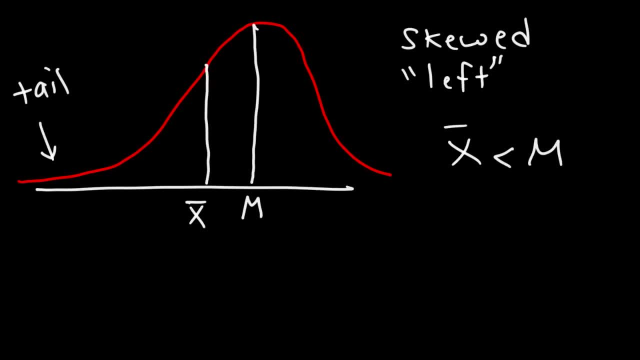 Now, how can we represent this using a box plot? Well, here's one possibility. So in this case, Q2 will be closer to Q3 in the box plot. So, as you can see, the left side is longer than the right side. 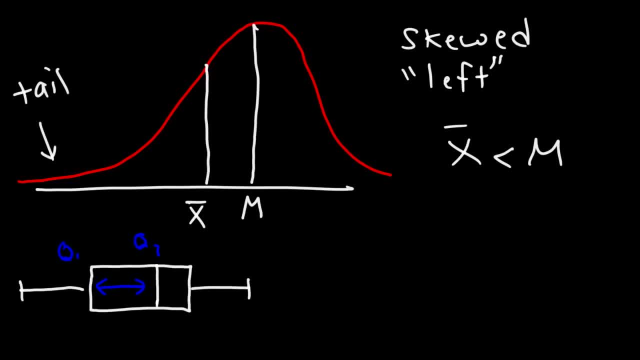 So we could say that Q2 minus Q1 is greater than Q3 minus Q2 in this case. Now, if the boxes are equal in length, you can also tell that we have a negative skew if the left side of the box plot is longer than the right side. 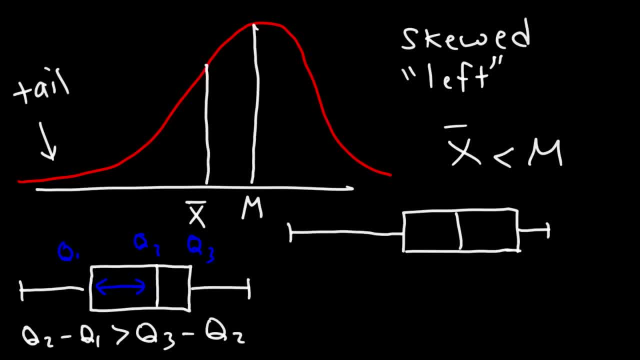 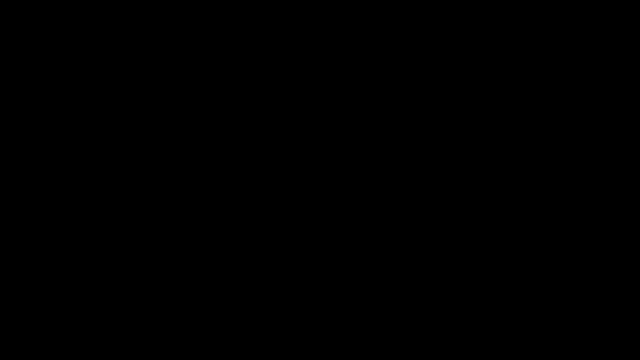 So in this case, Q2 is closer to Q3, so that's another indication that the data is skewed to the left. Now there are some other things that you need to know if you're going to take a statistics course. You need to be able to: 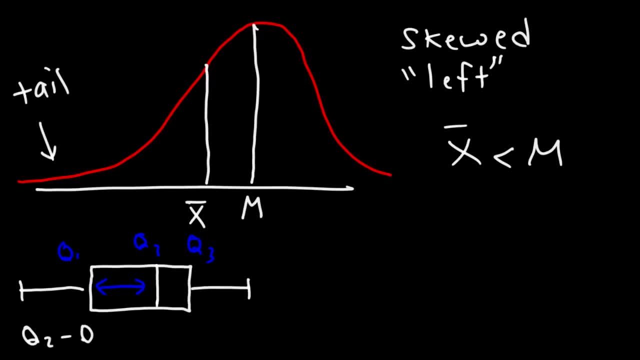 So we can say that Q2 minus Q1 is greater than Q3 minus Q2 in this case. Now, if the boxes are equal in length, you can also tell that we have a negative skew if the left side of the box plot is longer than the right side. 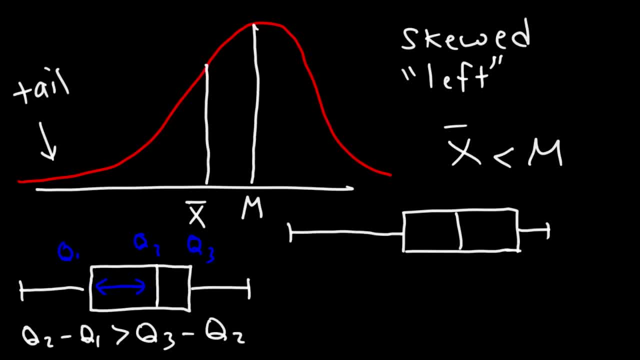 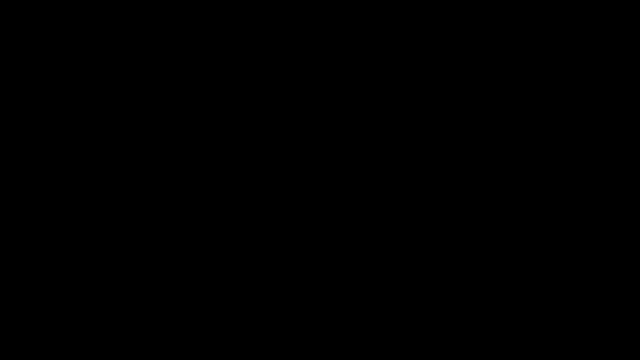 So that's another indication that the data is skewed to the left. Now there's some other things that you need to know if you're going to take a statistics course And you need to be able to create a dot plot. So let's say, if you have the numbers 5,, 8,, 3, 7,, 1,, 5,, 3,, 2,, 3,, 3,, 8,, 5.. 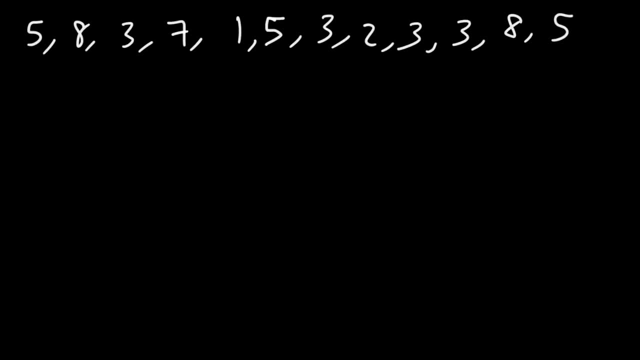 With this information, how can we construct a dot plot? Well, we can begin by drawing a number line. So let's say this is 0,, 1,, 2,, 3,, 4, and so forth. We can stop at 8, since 8 is the highest number. 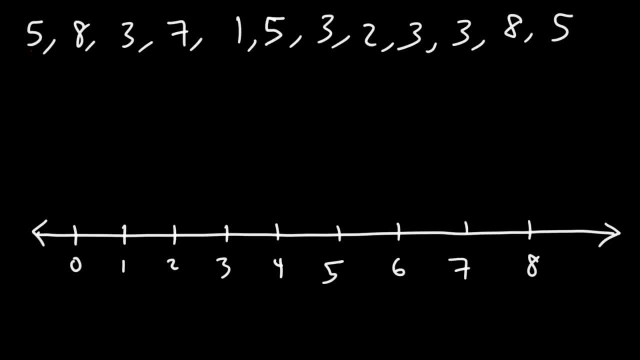 Now the first number is a 5.. So all we need to do is draw a dot above the number 5. And then let's put the dots, one at a time. Okay, So the next number is an 8.. So we're going to draw a dot at 8.. 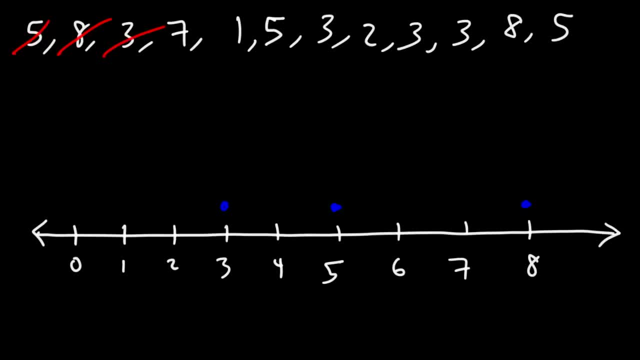 And then it's a 3.. So let's put the dot there. Next we have a 7. And then it's a 1. And then a 5.. So notice that we have a second 5.. All we need to do is draw another dot above the first one. 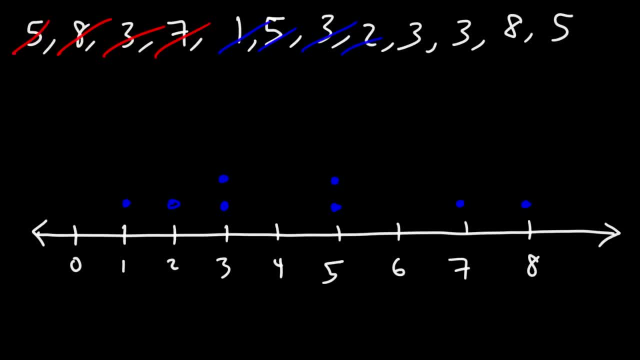 And then it's a 3., 2., And then another 3., And another 1., And then 8. And then 5.. So that's how you can make a dot plot. Now, using this dot plot, which number is the mode? 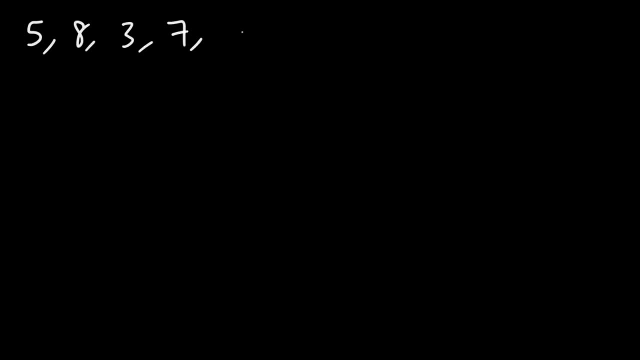 create a dot plot. So let's say you have the number 5, 8, 3, 7, 1, 5, 3, three, three, eight, five. With this information, how can we construct a dot plot? Well, we can begin by drawing a number line. So let's say this is 0,, 1,, 2,, 3,, 4, and so forth. 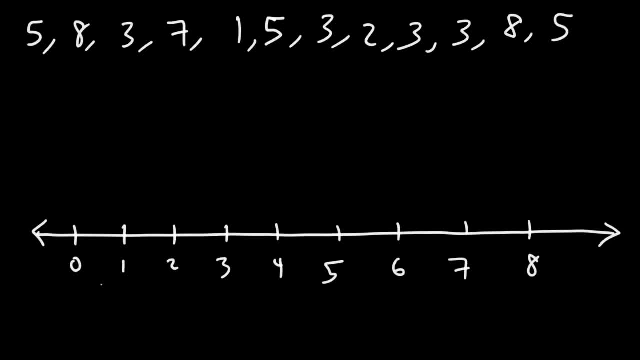 We could stop at 8, since 8 is the highest number. Now the first number is a 5.. So all we need to do is draw a dot above the number 5.. And then let's put the dots, one at a time. So the next number is an 8.. So we're going to draw a dot at 8.. 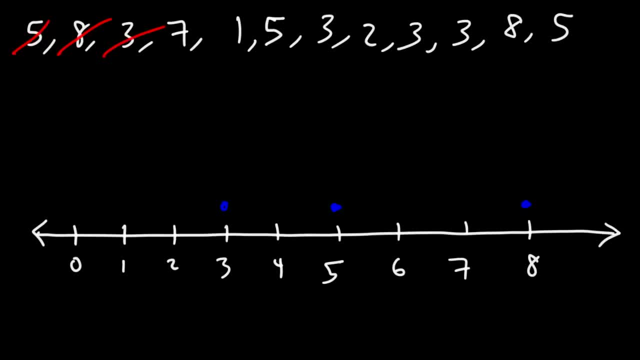 And then it's a 3.. So let's put the dot there. Next we have a 7., And then it's a 1., And then a 4. And then a 5.. So notice that we have a second 5.. All we need to do is draw another dot above the first one. 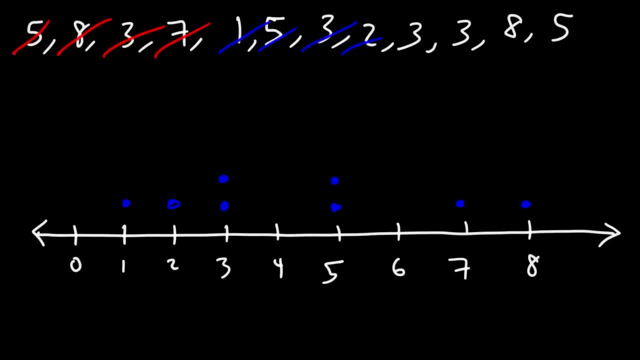 And then it's a 3,, 2,, and then another 3,, and another 1,, and then 8, and then 5.. So that's how you can make a dot plot. Now, using this dot plot, which number is the most important? 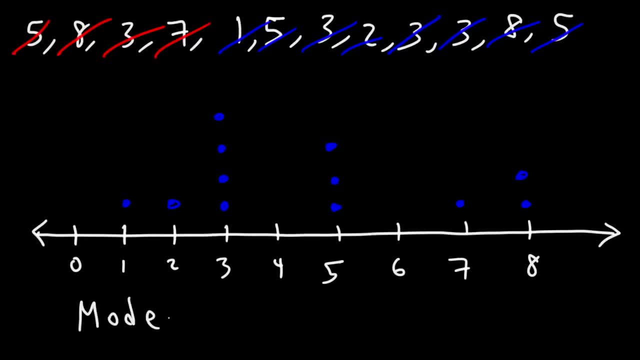 What would you say Now? if you recall, the mode is the number in the data set that occurs most frequently, So in this case it's the number with the most dots. So the mode for this data set is 3.. By the way, if you haven't done so already, don't forget to subscribe to this channel and click on that notification bell. 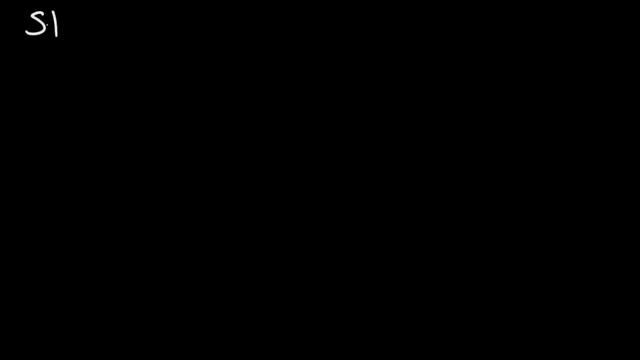 Now let's talk about how we can make a stem and leaf plot. So let's say we have the numbers 4,, 9,, 13,, 13,, 17,, 21,, 36,, 38,, let's say another 38, and then 56. 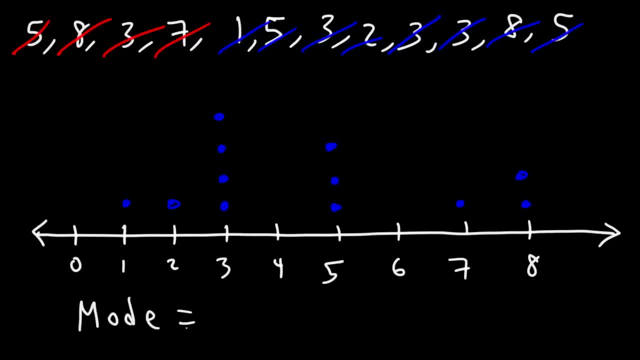 What would you say Now? if you recall, the mode is the number in the data set that occurs most frequently, So in this case it's the number with the most dots. So the mode for this data set is 3.. By the way, if you haven't done so already, 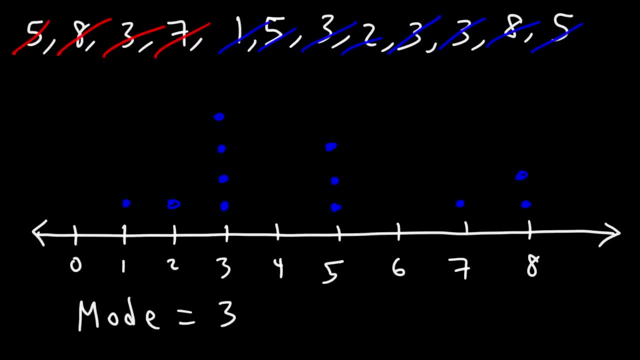 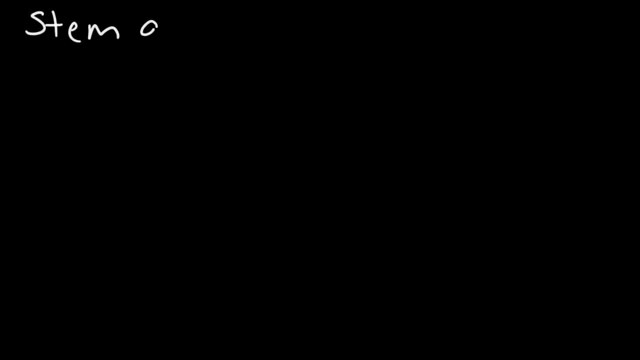 don't forget to subscribe to this channel and click on that notification bell. Now let's talk about how we can make a stem and leaf plot. So let's say we have the numbers 4,, 9,, 13,, 17,, 21,. 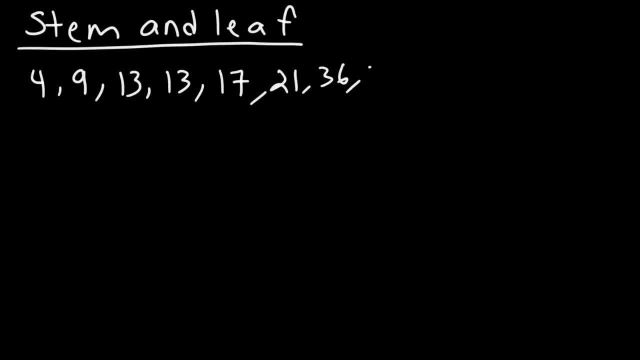 36,, 38,, let's say another 38, and then 56.. How can we make a stem and leaf plot with this data? So the first thing we need to do is we need to write two columns On. the left is going to be the stem. 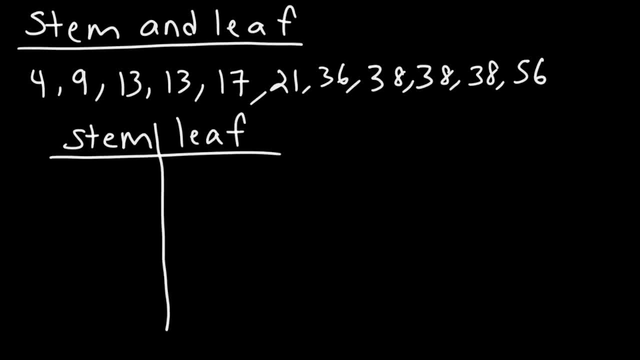 and on the right the leaf. So the first number is 4.. So for the stem we're going to write 0.. And for the leaf, we're going to put 4.. The next one is 9.. So we're going to write or represent 9 as 09.. 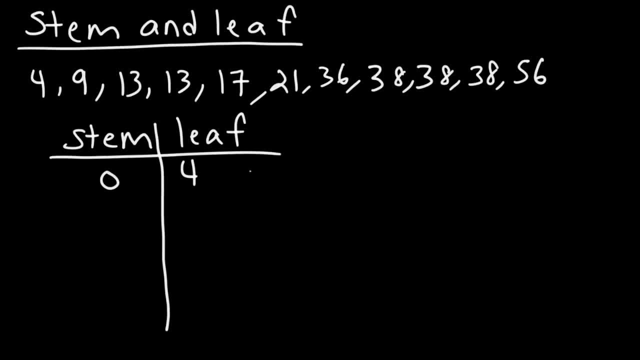 So we have 0 on the left and then we're going to put 9 on the right. The next number is 13.. So the first digit is a 1.. The second digit we're going to put in the second column. 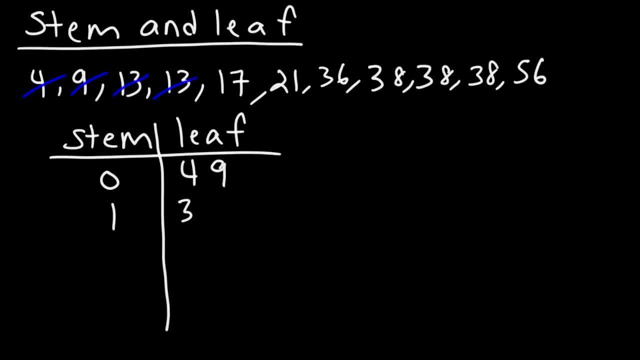 Now we have another 13.. So all we got to do is add another 3.. Now for 17,. we need 1 and 7.. We already have the 1,, but we need to write the 7 to the right side. 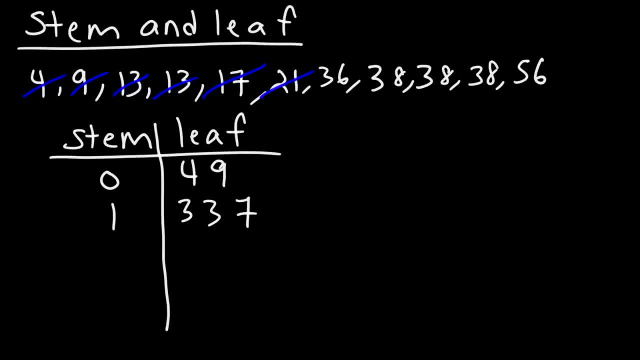 Now for 21,. we need to put a 2 in the stem column, a 1 in the leaf column. Next we have 36.. So we need a 3 in the stem column, a 6 in the leaf column. Now notice that we have three 38s. 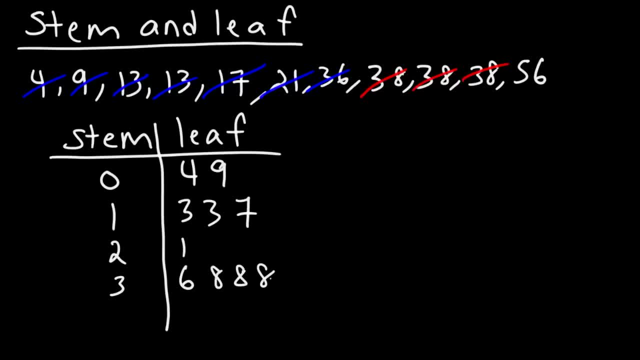 So we got to add three 8s to the leaf column And finally 56. Now we don't have anything in the 40s, So we're going to write a 4, but we're not going to put anything here. 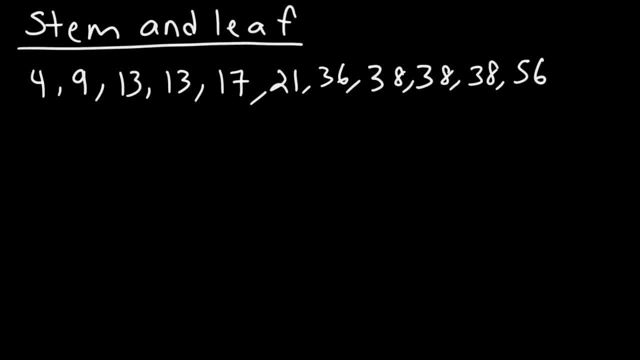 How can we make a stem and leaf plot? How can we make a leaf plot with this data? So the first thing we need to do is we need to write two columns: On the left is going to be the stem and on the right the leaf. 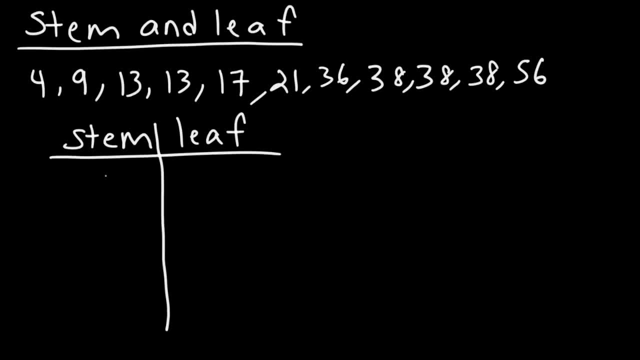 So the first number is 4.. So for the stem we're going to write 0. And for the leaf we're going to put 4.. The next one is 9.. So we're going to write or represent 9 as 0, 9.. 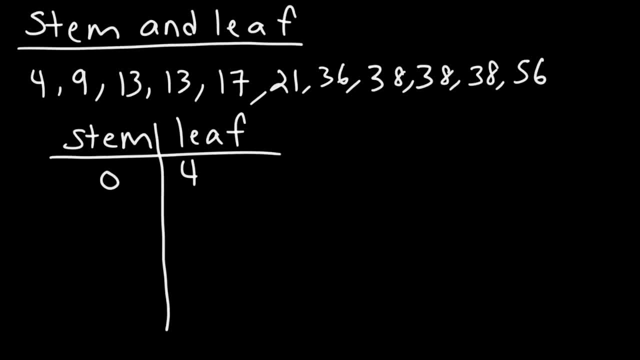 So we have 0 on the left and then we're going to put 9 on the right. The next number is 13.. So the first digit is a 1.. The second digit we're going to put in the second column. 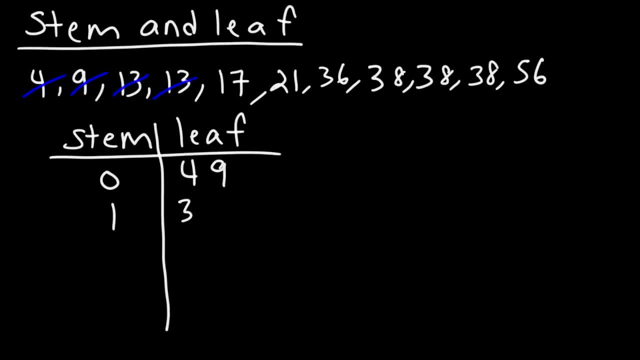 Now we have another 13.. So all we got to do is add another 3.. Now for 17,. we need 1 and 7.. We already have the 1,, but we need to write the 7 to the right side. 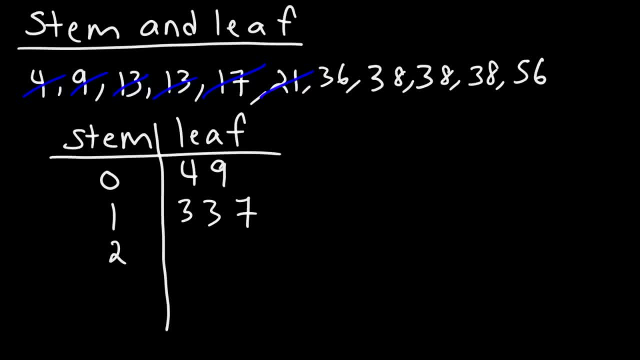 Now for 21,. we need to put a 2 in the stem column, A 1 in the leaf column. Next we have 36. So we need a 3 in the stem column, a 6 in the leaf column. 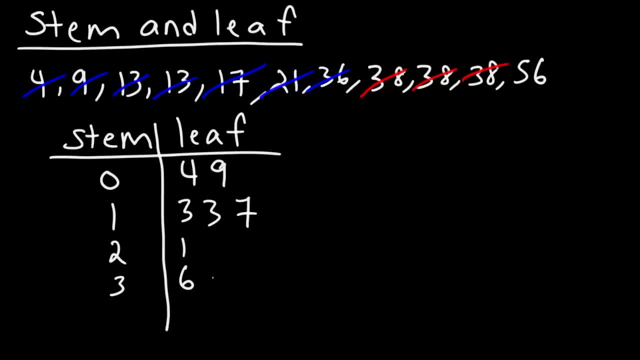 Now notice that we have three 38s, So we got to add three 8s to the leaf column And finally 56. Now we don't have anything in the 40s, So we're going to write a 4, but we're not going to put anything here. 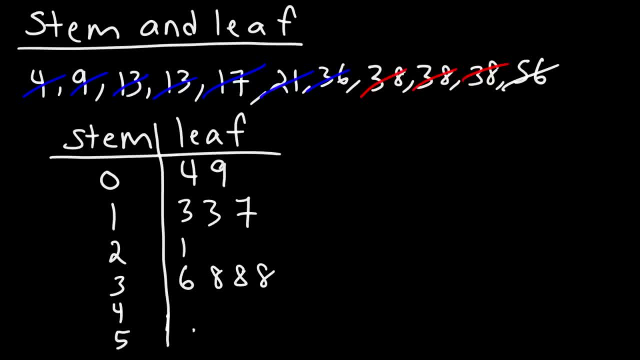 For 56, we're going to write a 5 in the stem column and a 6 in the leaf column, And so that's how you can make a stem and leaf plot. Now, it's always good to have a key, So we could say that 2, 1 represents 21.. 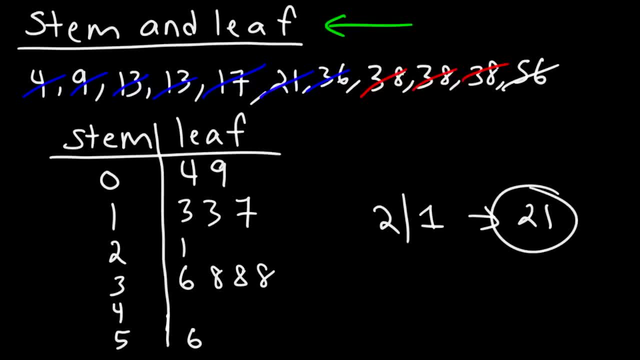 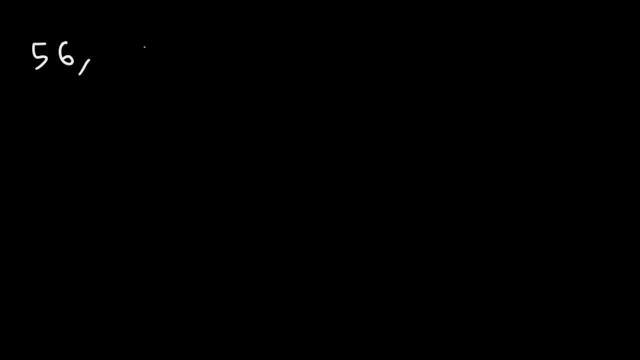 So if someone looks at the stem and leaf plot, they know what you mean. Let's try another example. So let's say we have the numbers 56.. Actually let's say 78,, 85.. 89,, 92,, 106,, 107, and 119., 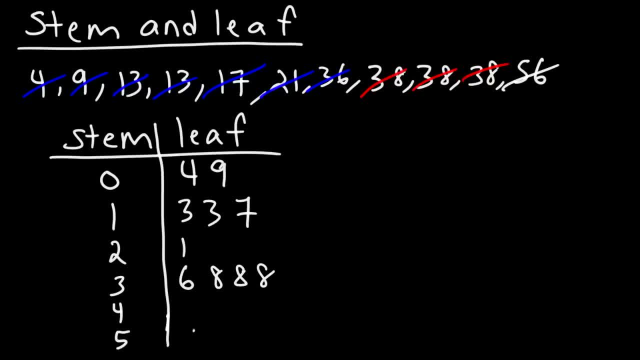 For 56, we're going to write a 5 in the stem column and a 6 in the leaf column, And so that's how you can make a stem and leaf plot. Now, it's always good to have a key, So we could say that: 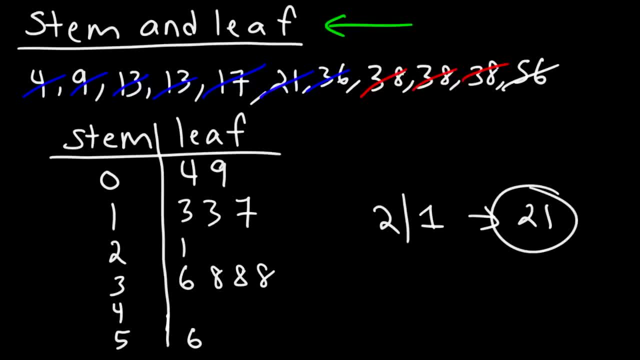 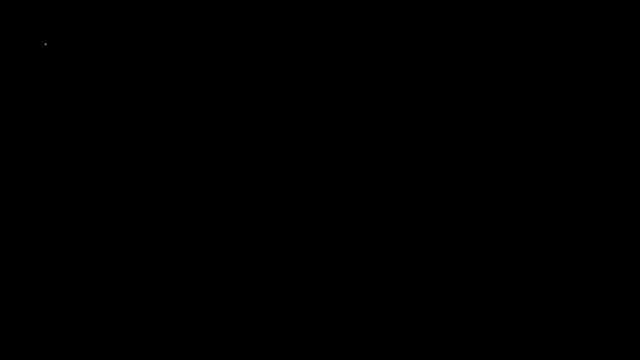 21 represents 21.. So if someone looks at the stem and leaf plot, they know what you mean. Let's try another example. So let's say we have the numbers 56, actually let's say 78,, 85,, 89,. 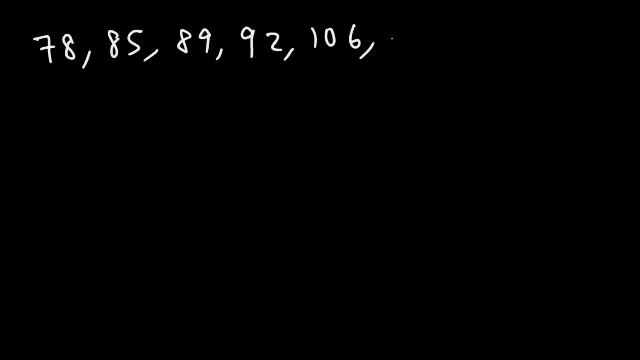 92,, 106,, 107, and 119.. Go ahead and make a stem and leaf plot with those numbers. So the first number is 78.. We're going to write a 7 in the first column and an 8 in the second column. 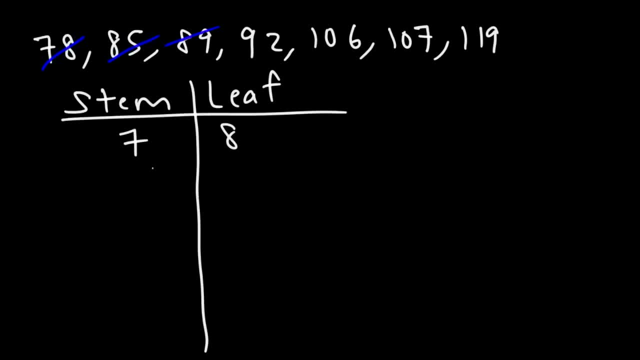 Next we have 85 and 89. So we're going to put an 8 for the first digit, and then 5 and 9 for the second, And then it's 92, so we're going to write 9 and 2.. 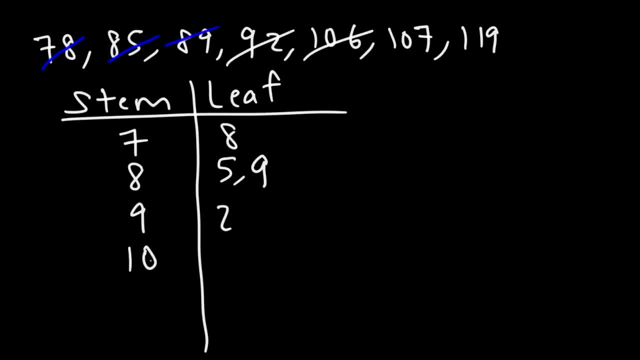 Now for 106, we're going to put a 10 in the stem column but a 6 in the leaf column, And for 107, we just got to add a 7 here, And there's usually no commas, so let's get rid of that. 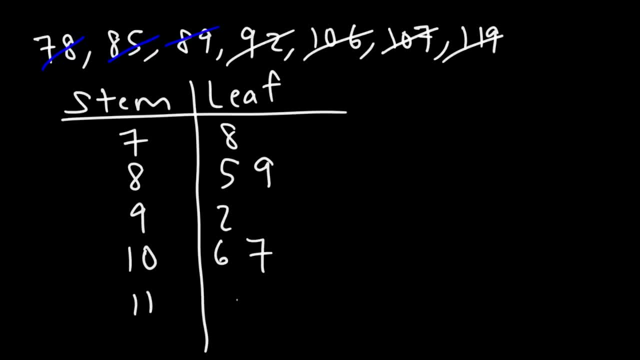 And then, finally, for 119,, we're going to write 11 in the stem plot and 9 in the leaf column, And so, for example, this will be our key. So this represents 92, and this would represent 106.. 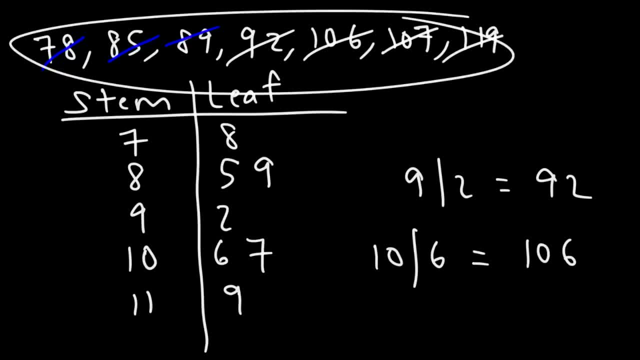 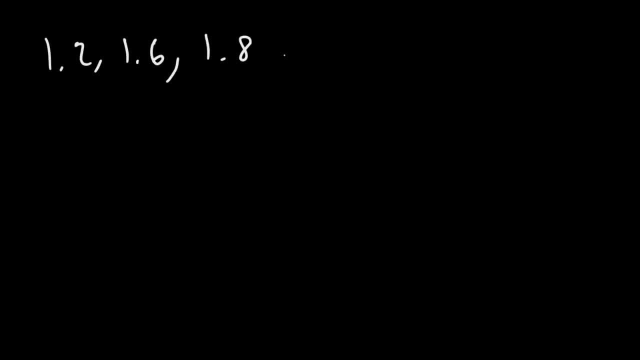 Because sometimes you could have decimal values. For instance, let's say, if we have 1.2, 1.6,, 1.8,, 2.1,, 2.3,, 2.3, and 2.5.. 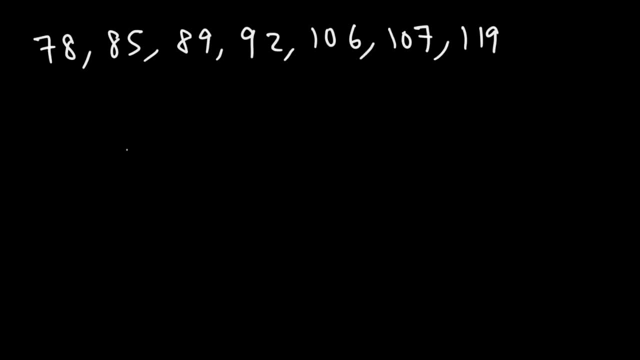 Go ahead and make a stem and leaf plot with those numbers. So the first number, 78.. We're going to write a 7 in the first column and an 8 in the second. Next we have 85 and 89.. 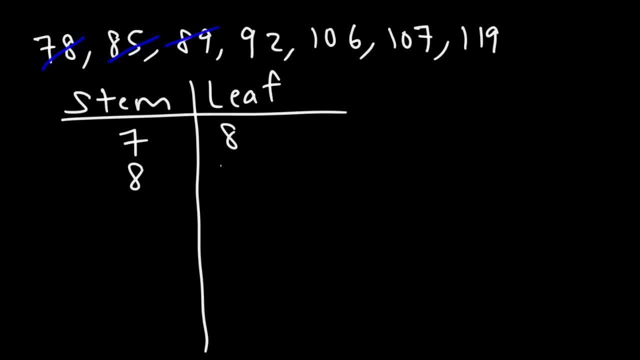 So we're going to put an 8 for the first digit and then 5 and 9 for the second, And then it's 92, so we're going to write 9 and 2.. Now for 106, we're going to put a 10 in the stem column but a 6 in the leaf column. 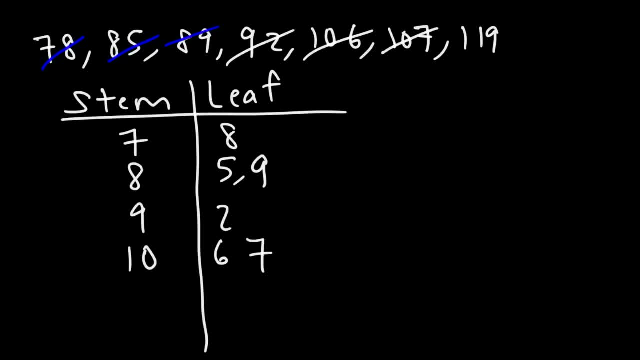 And for 107, we just got to add a 7 here And there's usually no commas, so let's get rid of that. And then, finally, for 119, we're going to write 119.. And then for 119, we're going to write 119. 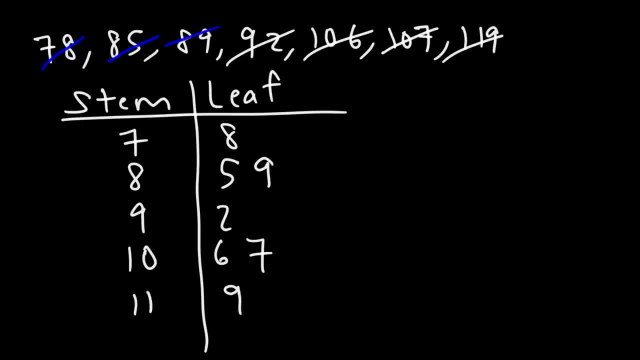 So we're going to write 11 in the stem plot and 9 in the leaf column, And so, for example, this will be our key. So this represents 92, and this would represent 106. Because sometimes you could have decimal values. 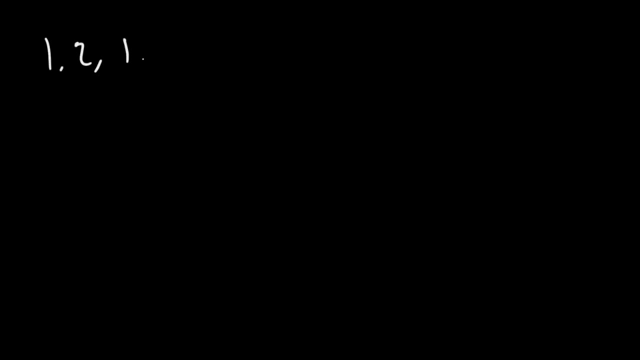 For instance, let's say, if we have 1.2,, 1.6,, 1.8,, 2.1,, 2.3,, 2.3, and 2.5.. We can construct this stem and leaf plot like this: 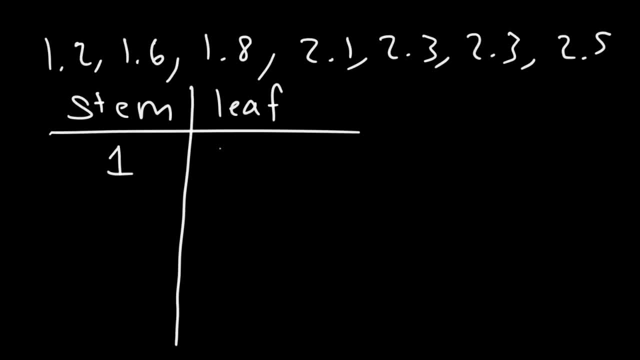 So we could start with 1, and to write 1.2, we could just put a 2 for the leaf plot. Now, for 1.6, we just got to put a 6 in the leaf column, And for 1.8, just an 8.. 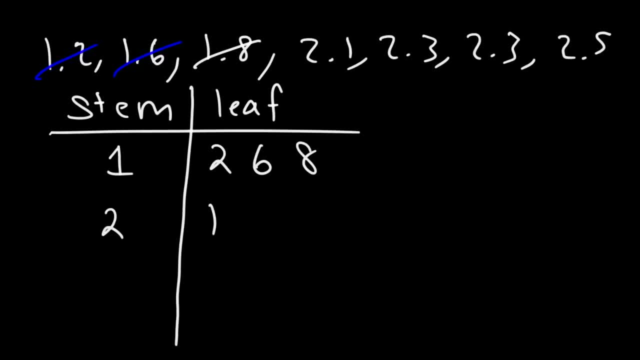 Now we can move on to the 2s. So we have 2.1,, 2.3,, 2.3, and 2.6.. So we have 2.1,, 2.3,, 2.3, and 2.6.. 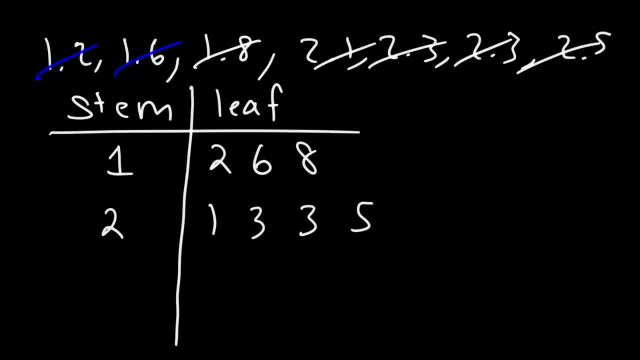 So we have 2.1, 2.3, 2.6.. So we have 2.1, 2.6. And 2.5.. And so that's how you can make a stem and leaf plot using decimal values. 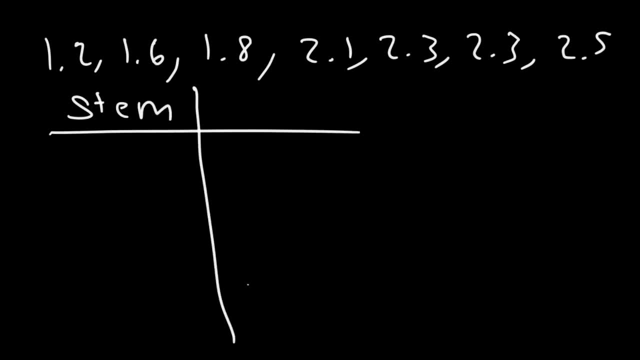 We can construct this stem and leaf plot like this, So we could start with 1, and to write 1.2, we could just put a 2 for the leaf plot. Now for 1.6, we just got to put a 6 in the leaf column. 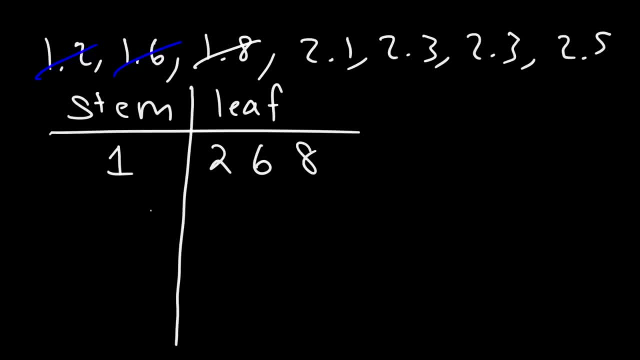 And for 1.8, just an 8.. Now we can move on to the 2s, So we have 2.1,, 2.3,, 2.3, and 2.5.. And so that's how you can make a stem and leaf plot. 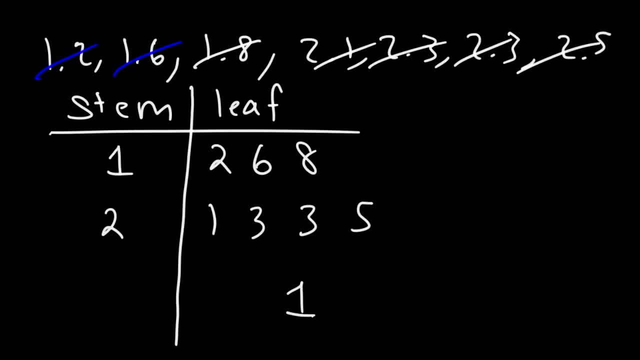 using decimal values. So we could say: 1.6 represents 1.6 in this particular example. Now the next thing we're going to talk about is something called a frequency table. So, given a data set, how can we make a frequency table? 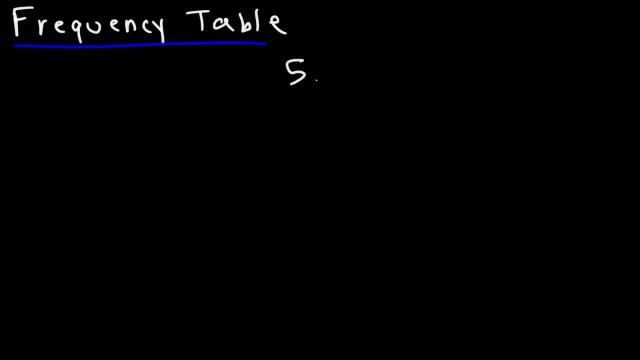 So let's say we have the numbers 5,, 9,, 8,, 7,, 8,, 12,, 9,, 8,, 10,, 8,, 9,, 7.. So using those numbers, how can we make a frequency table? 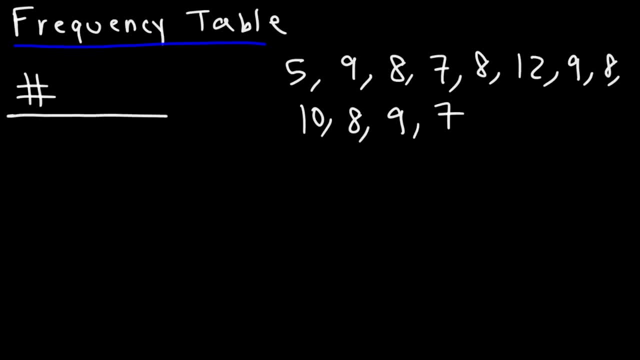 We're going to put two columns, So the first column will represent the number and the second column will represent the frequency. And let's put down what we have. So the first number is a 5.. And how many 5s do we have? 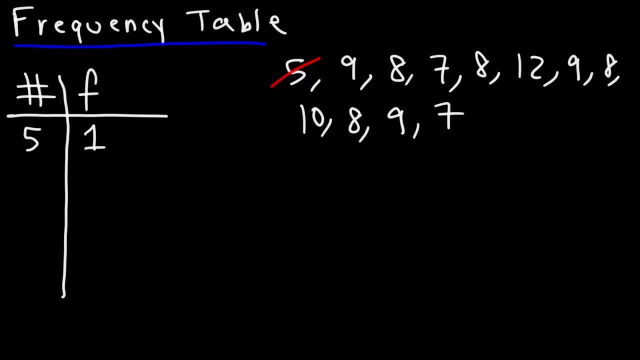 There's only one, 5,, so the frequency is 1.. The next number is a 7.. And notice that we have two 7s, so the frequency is 2.. Next is 8.. We have a total of 4- 8s. 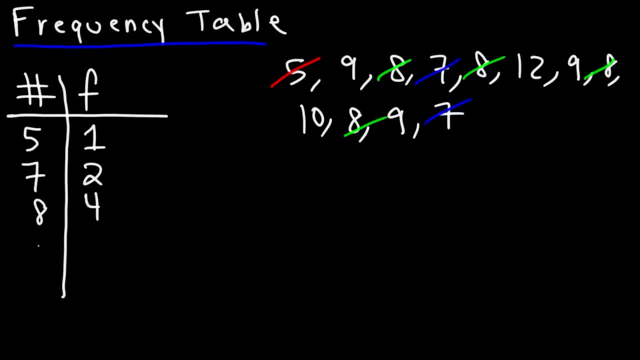 So that gives us a frequency of 4.. After that we have 9. And I've spotted three 9s, And then there's one 10. And we have one 12.. So that's a simple way in which you can make a frequency table. 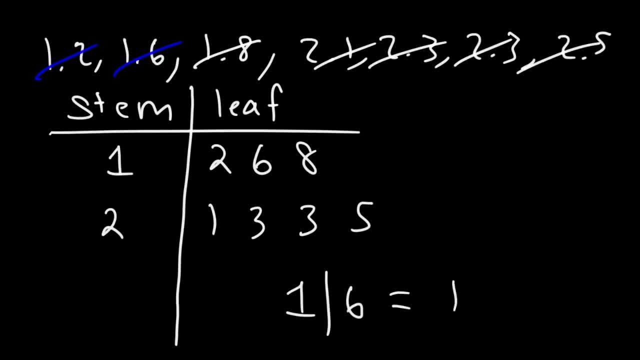 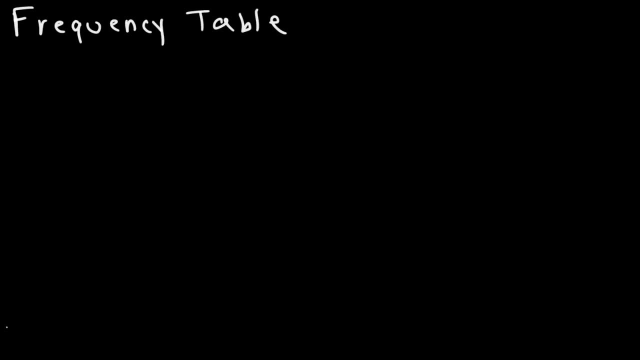 So we could say: 1.6 represents 1.6 in this particular example. Now the next thing we're going to talk about is something called a frequency table. So, given a data set, how can we make a frequency table? So let's say we have the numbers. 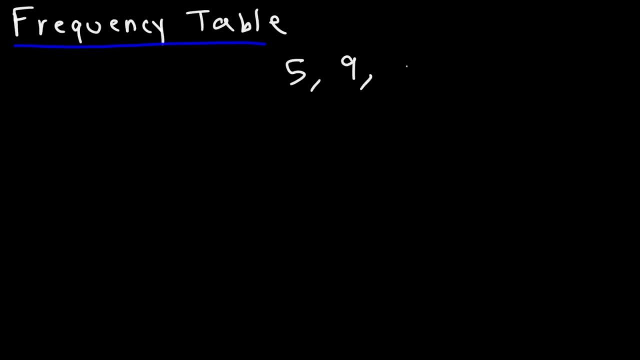 1., 2., 3., 4., 5., 9., 8., 7., 8., 12., 9., 8., 10., 8., 9., 7.. So using those numbers, how can we make a frequency table? 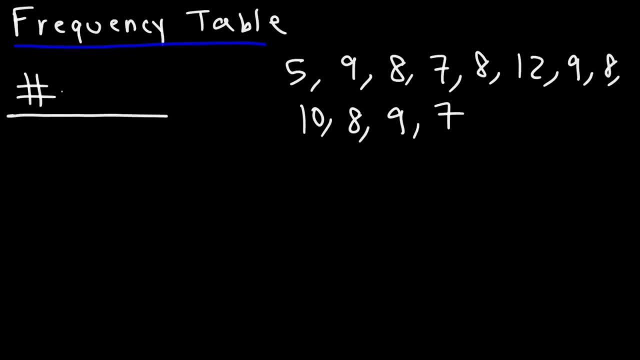 We're going to put two columns, So the first column will represent the number And the second column We'll represent the frequency. And let's put down what we have. So the first number is a 5.. And how many 5's do we have? 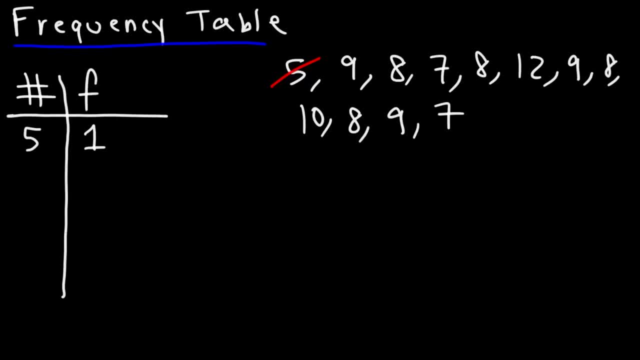 There's only one 5,, so the frequency is 1.. The next number is a 7.. And notice that we have two 7's, So the frequency is 2.. Next is 8.. We have a total of 4 8's. 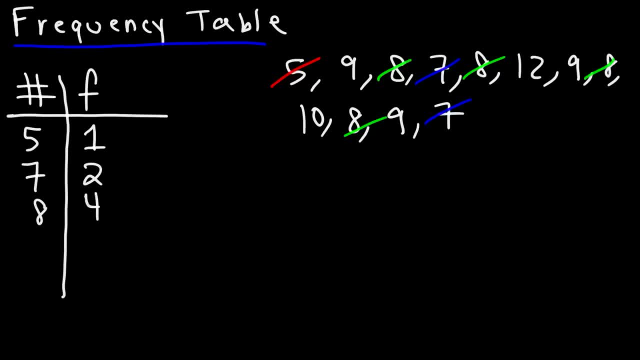 So that gives us a frequency of 4.. After that we have 9. And I've spotted 3 9's, And then there's one 10. And we have one 12.. So that's a simple way in which you can make a frequency table. 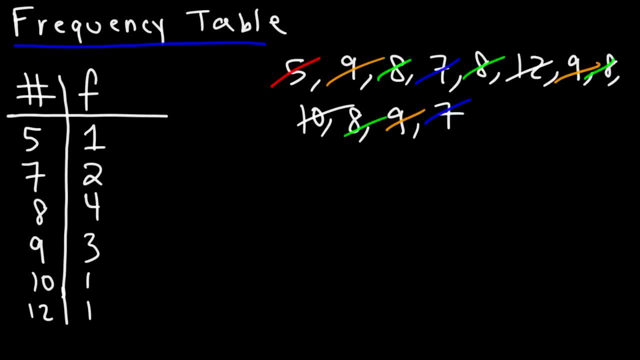 Now here's another question for you. How can we use the frequency table In order to calculate the sample mean? How can we calculate the average instead of just adding all of those numbers up and dividing by the number of data points in a set? 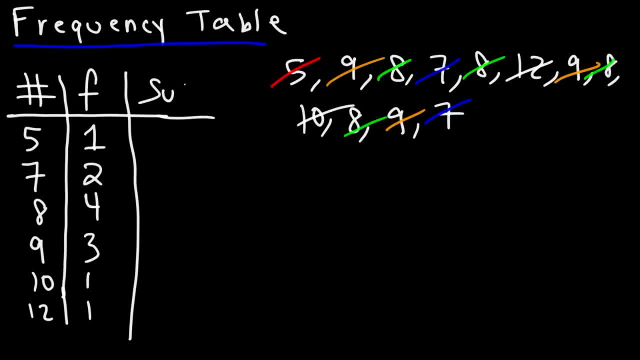 Let's add another column And we're going to call this the sum. Now we have one 5.. So 5 times 1 is 5. We have two 7's. If you add up 7 and 7, you get 14.. 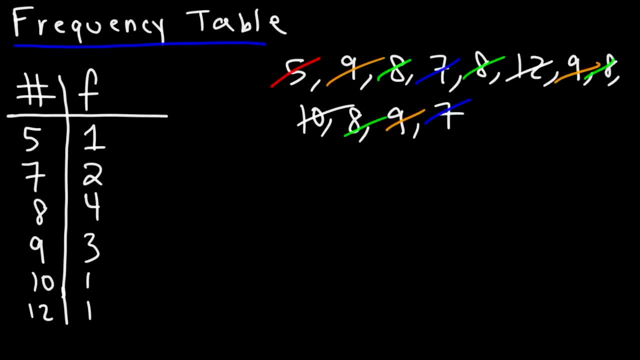 Now here's another question for you. How can we use the frequency table in order to calculate the sample mean? How can we calculate the average instead of just adding all of those numbers up and dividing by the number of data points in a set? 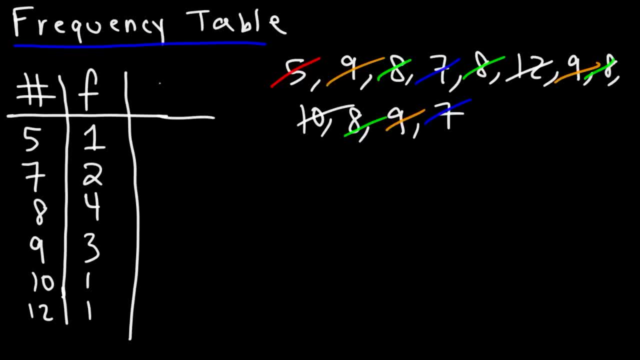 Let's add another column And we're going to call this the sum. Now we have one 5, so 5 times 1 is 5.. We have two 7s. If you add up 7 and 7, you get 14.. 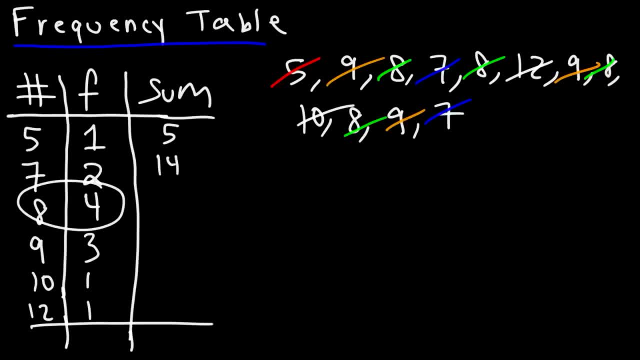 We have four 8s. 8 times 4 is 32.. Or if you add 8 four times, you get 32.. 9 times 3 is 27.. 10 times 1 is 10.. 12 times 1 is 12.. 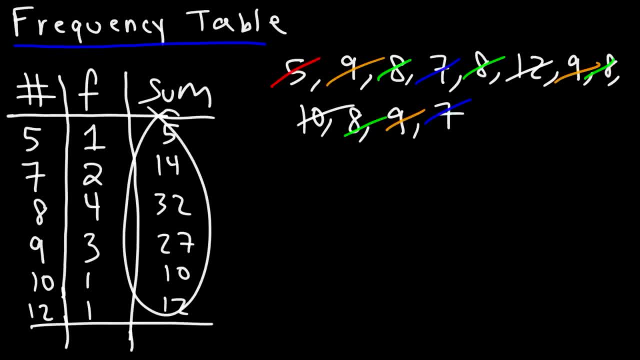 Now we're going to add up the sum column to get the total sum. So 5 plus 14 plus 32 plus 27 plus 10 plus 12, that's 100.. And we're also going to add up the frequency column. 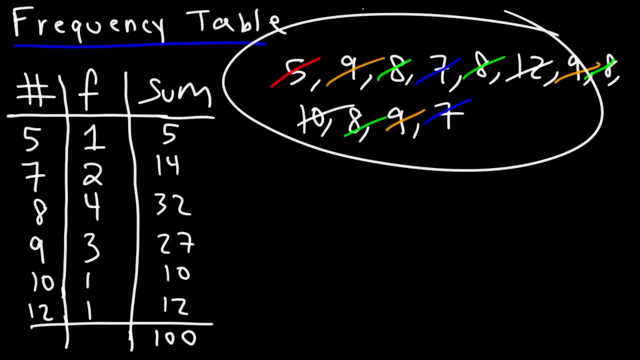 That's going to give us the total number of numbers that we have here. So we have 1 plus 2, which is 3, plus 4, that's 7, plus 3, that's 10, plus 2,, that's 12.. 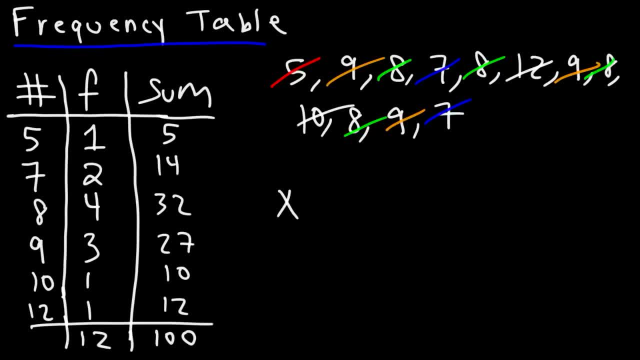 So we have a total of 12 numbers. So the mean is going to be the sum divided by the total number of points that we have in our set. So it's 100 divided by 12.. So the mean in this example is 8.3 repeated. 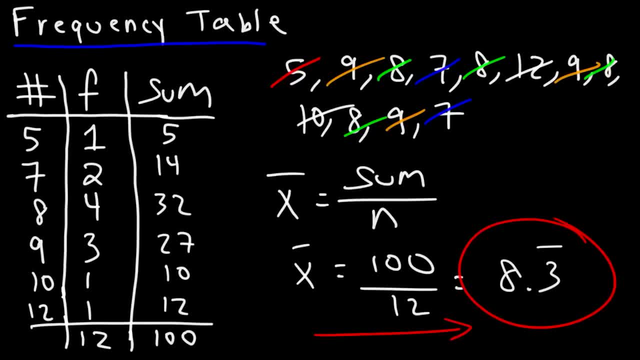 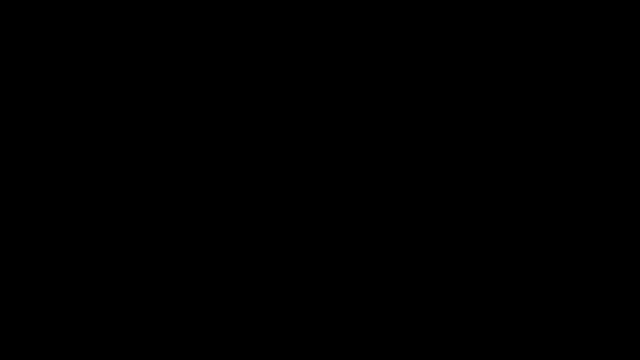 And so that's how you could use the frequency table to calculate the mean of a data set. Now, the next thing that you need to know how to do is how to create a histogram. A histogram looks like a bar graph, But unlike a bar graph. 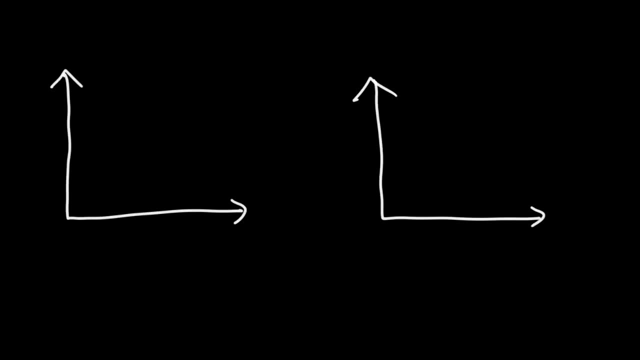 a histogram has its bars connected to each other. So here's an example of a histogram on the left side. On the right side, I'm going to draw a bar graph, So this would be a bar graph. So, as you can see, they're very similar. 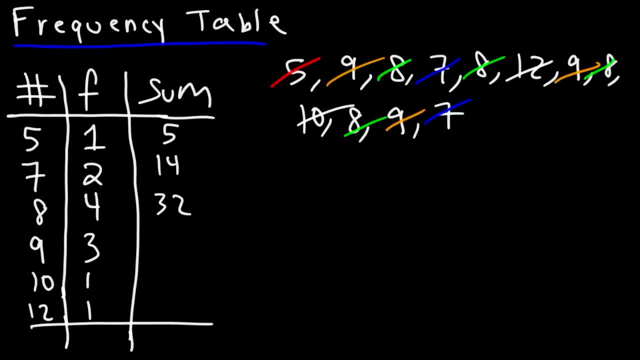 We have four 8's. 8 times 4 is 32.. Or if you add 8 four times, you get 32.. 9 times 3 is 27.. 10 times 1 is 10.. 12 times 1 is 12.. 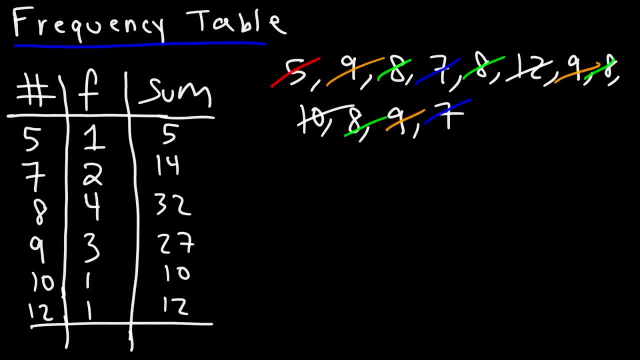 Now we're going to add up the sum column to get the total sum, So 5 plus 14 plus 32 plus 27.. We're going to add up the sum column to get the total sum, So 5 plus 14 plus 32 plus 27.. 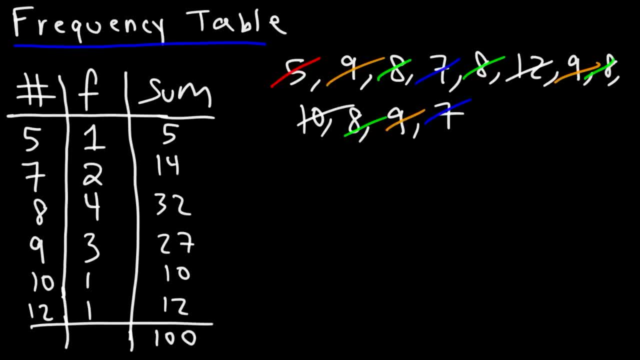 Plus 10 plus 12, that's 100.. And we're also going to add up the frequency column. That's going to give us the total number of numbers that we have here. So we have 1 plus 2, which is 3 plus 4, that's 7 plus 3, that's 10 plus 2, that's 12.. 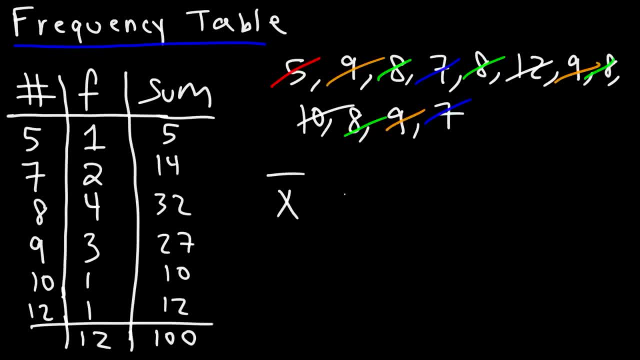 So we have a total of 12 numbers. So the mean is going to be the sum divided by the total number of points that we have in our set. So it's 100 divided by 12.. So the mean in this example is 8.3 repeated. 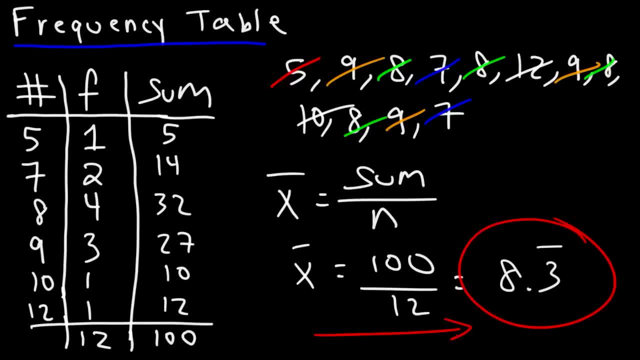 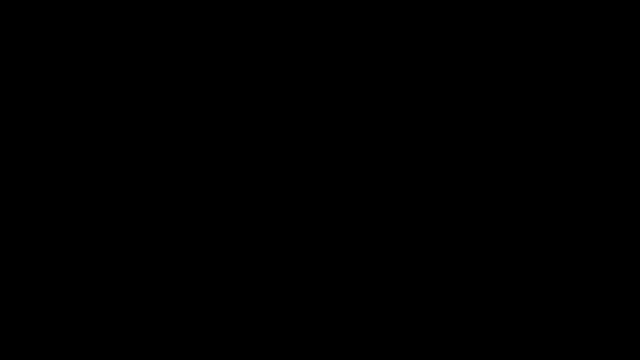 And so that's how you could use the frequency table to calculate the mean of a data set. Now, the next thing that you need to know how to do is how to create a histogram. A histogram looks like a bar graph, But unlike a bar graph. 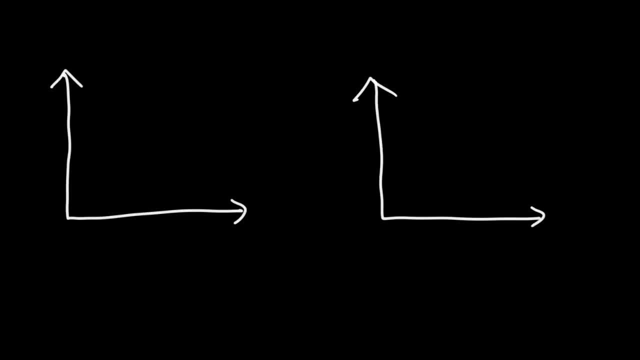 A histogram has its bars connected to each other. So here's an example of a histogram on the left side. On the right side I'm going to draw a bar graph. So this would be a bar graph. So, as you can see, they're very similar, but the bars in the histogram they're adjacent. 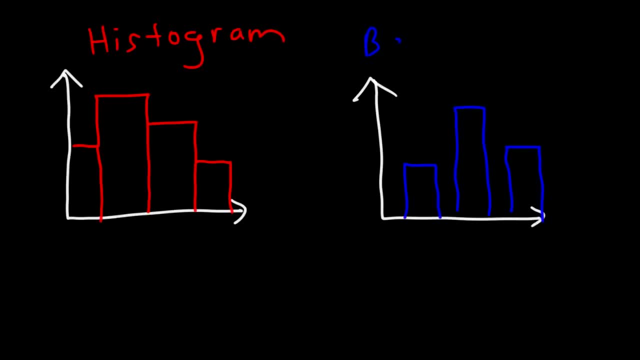 to each other. There's no space in between. But how do you do that? But how do we go about taking the data set and making a histogram? So let's say we have the test scores of students in a typical class. Let's say the test scores are 65,, 72,, 93,, 68,, 76,, 98,. let's say 84,, 85,, 96, and 98.. 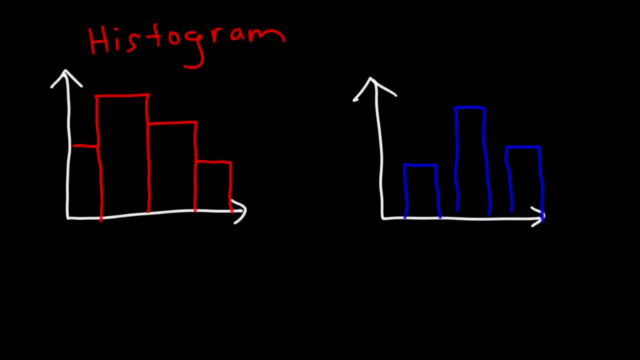 but the bars in the histogram, they're adjacent to each other. There's no space in between. But how do we go about taking a data set and making a histogram? So let's say we have the test scores of students in a typical class. 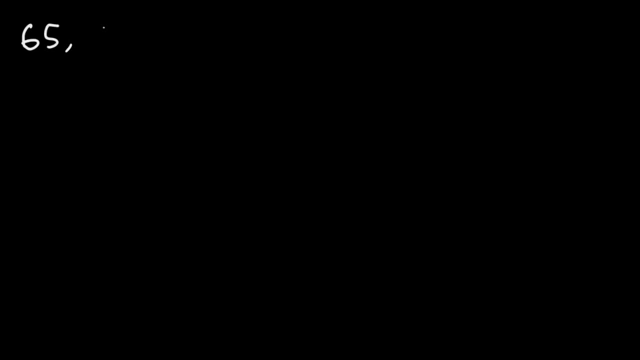 Let's say the test scores are 65,, 72,, 93,, 68,, 76, 98,. let's say 84, 85,, 79,, 88,, 90,, 82,, 83,, 87,. 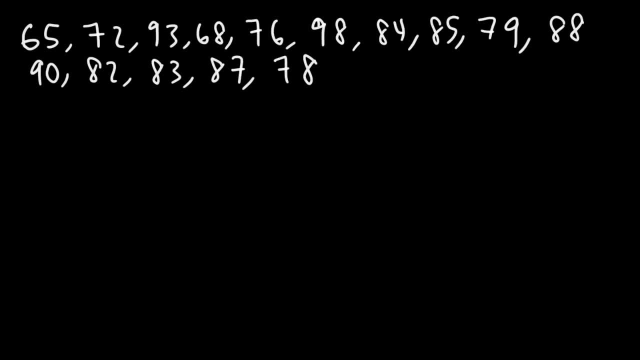 and 78.. Now, the first thing we need to do is create a frequency distribution table, And so what we're going to do this time, rather than talk about how frequent, or rather than describing the frequency of each number, we're going to break it up into categories or classes. 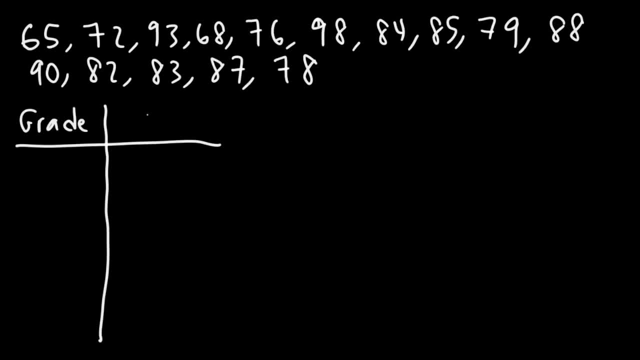 On the left side we're going to have the grade. On the right side, the frequency. Now I'm going to categorize the grades in levels of 10.. So a D would be 60 to 69.. A C would be 70 to 79.. 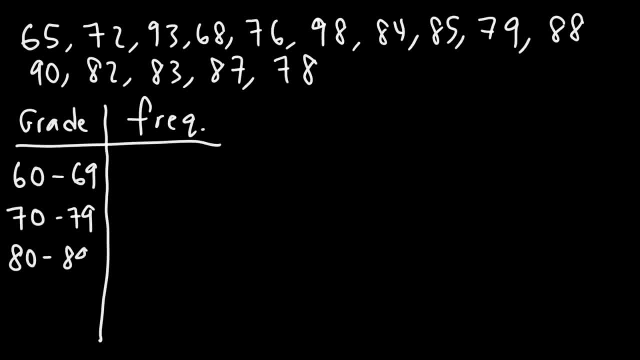 A grade of a B would be 80 to 89. And an A is going to be 90 to 100. So those are our four categories, or four classes. Now how many students received a grade between 60 and 69?? 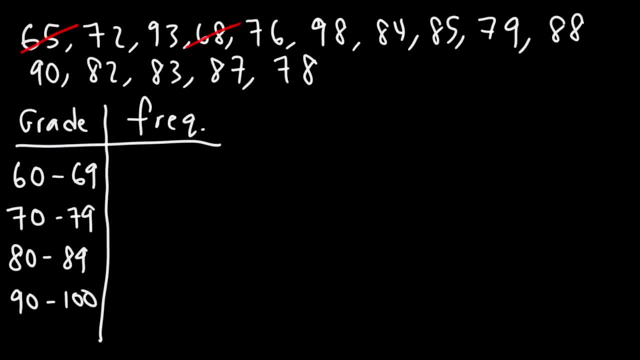 So notice that there are two students. We have the grades 65 and 68, so the frequency will be two. Now, how many students received a C on their exam? How many students received a grade of somewhere between 70 and 79?? 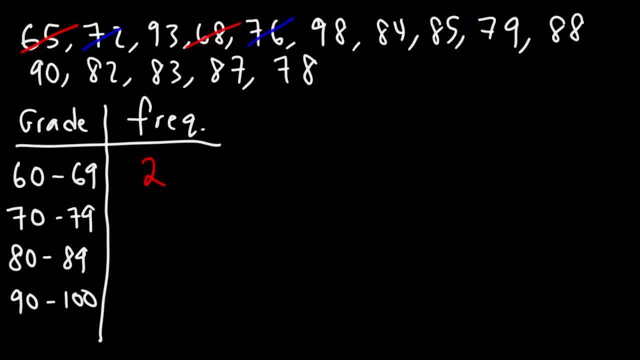 So we have one, two, three and four. So four students got a C on their exam. What about a B? So we have 84, 85,, 88,, 82,, 83, 87. So I counted a total of six. 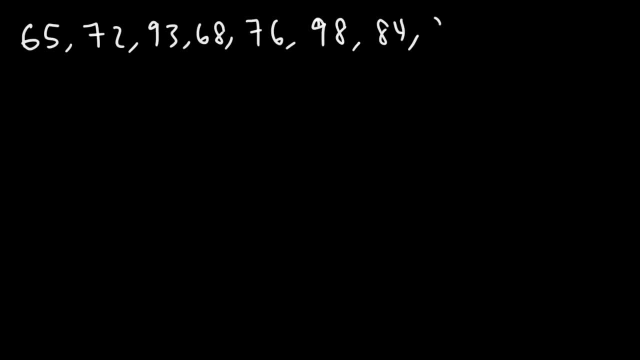 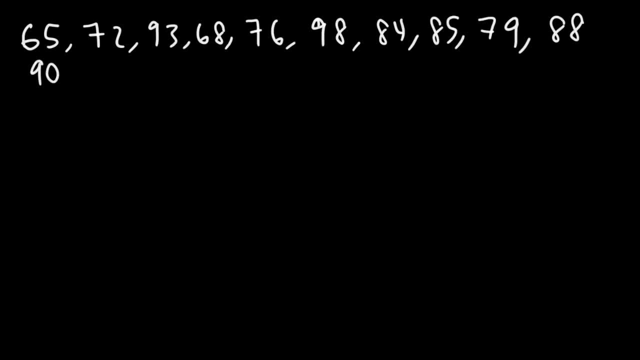 Let's say we have a bar graph. Let's say we have a bar graph. So let's say we have a bar graph, Okay, And these bar graphs are right next to what's black bar atqueское. They are very similar in shape. 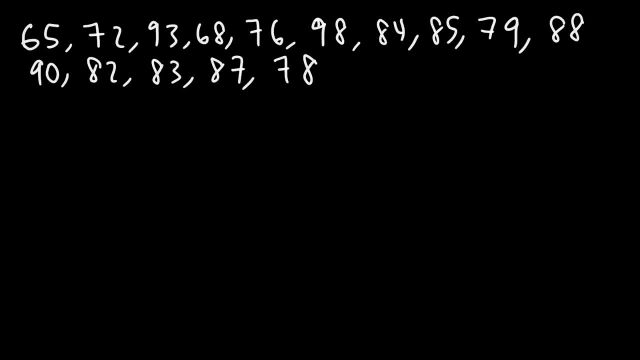 Like. In fact, what I'm saying is not only that the numbers aren't the same, into the great expectations, we're going to break it up into categories or classes. On the left side, we're going to have the grade. On the right side, the frequency. Now I'm going to categorize the grades. 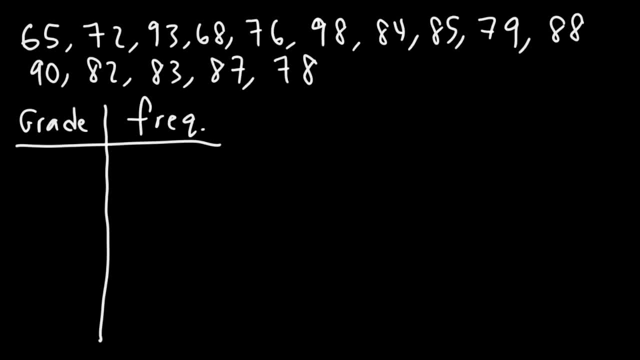 in levels of 10.. So a D would be 60 to 69.. A C would be 70 to 79. A grade of a B would be 80 to 89. And an A is going to be 90 to 100.. So those are our four categories, or four classes. 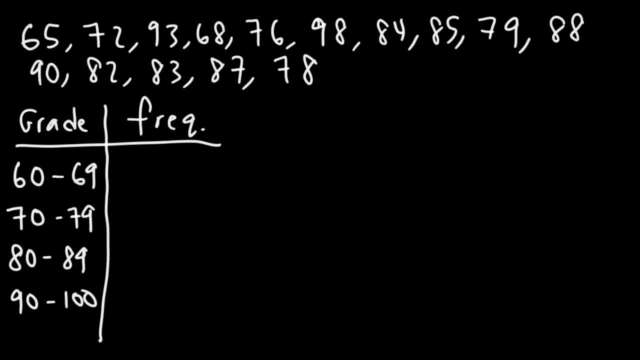 Now how many students received a grade between 60 and 69?. So notice that there are two students. We have the grades 65 and 68. So the frequency will be two. Now how many students received a C on their exam? 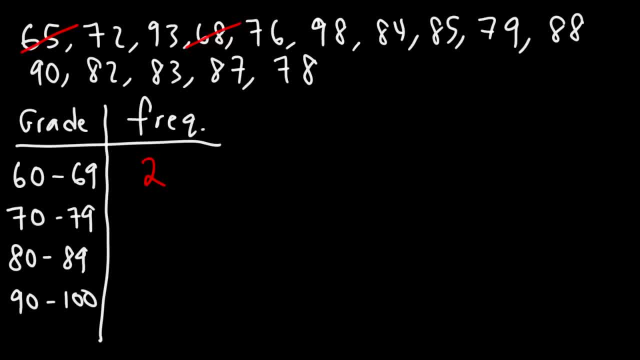 How many students received a grade of somewhere between 70 and 79?? So we have one, two, three and four. So four students got a C on their exam. What about a B? So we have 84,, 85,, 88,, 82,, 83,, 87. So I counted a total of six. 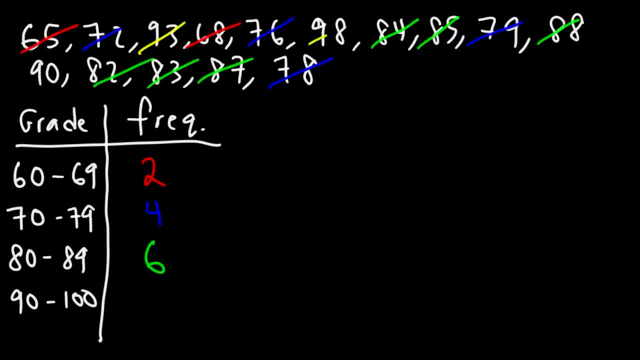 And what's left over are those who got an A 93,, a 98, and a 90.. So now that we have our frequency distribution table, we can now make a histogram. So on the y-axis, we're going to plot the frequency. 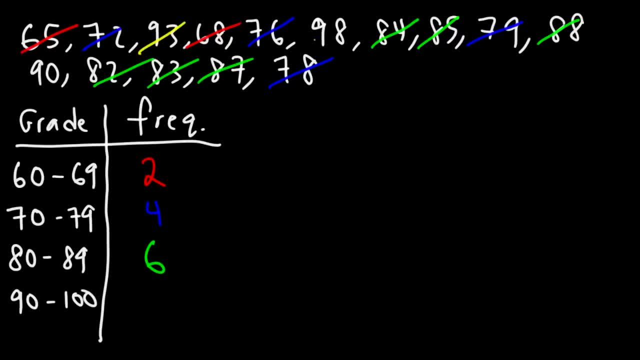 And what's left over are those who got an A, a 93,, a 98, and a 90.. So now that we have our frequency distribution table, we can now make a histogram. So on the y-axis, we're going to plot the frequency. 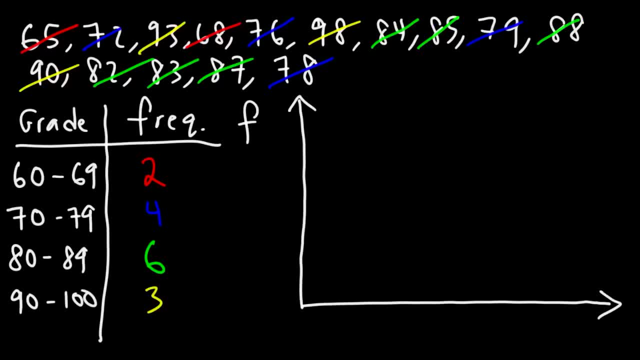 On the x-axis we're going to put the grades, So the grades will vary between 60, 70,, 80,, 90, and 100, because the classes are separated by intervals of 10, approximately. Now the highest frequency is six. 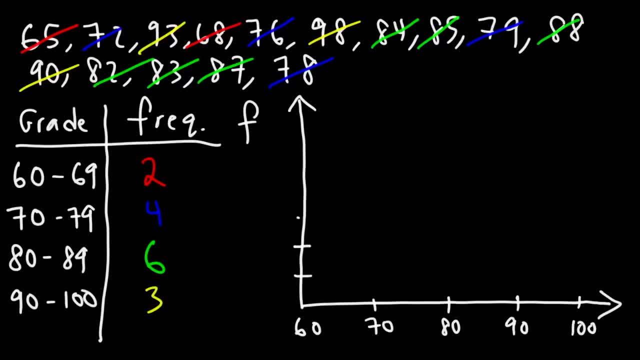 so let's go by one: One, two, three, four, five, six. So let's plot the first one Between 60 and 69,, which is close to 70, the frequency is a two, So it's going to look like that. 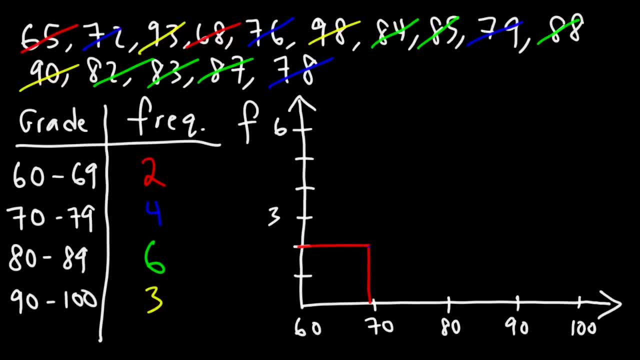 And then between 70 and 79,- four students got a grade in that region- I'm going to use the same color- And between 80 and 89, six students fall in that category And between 90 and 100, only three students. 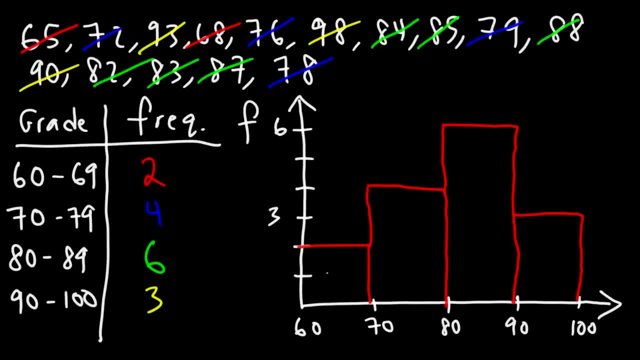 received an A. So let's put the grades. So this is a D: Two students got a D, Four students got a C And six students received a B And three students received an A. So that's how you can create a histogram. 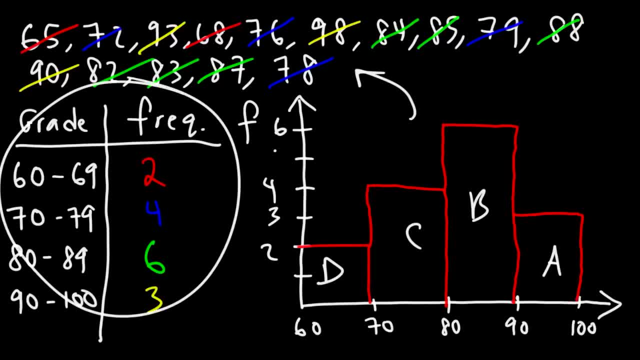 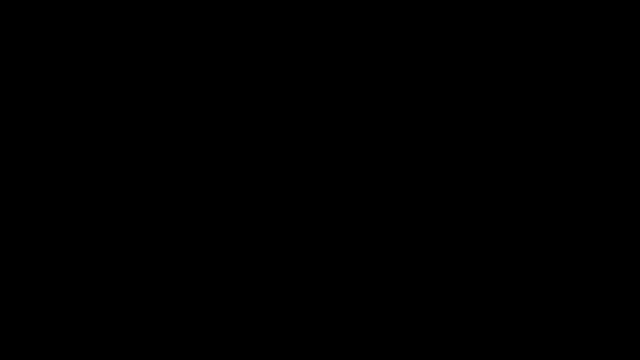 from a data set like this, using a frequency distribution table. Now there's something else that we need to go over, And that is making a table with the frequency, the relative frequency and also the cumulative relative frequency. So let's say we have the numbers. 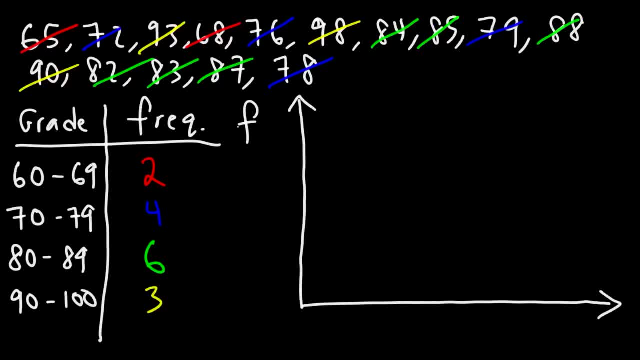 On the x-axis we're going to put the grades, So the grades will vary between 60,, 70,, 80,, 90, and 100, because the classes are separated by intervals of 10, approximately. Now the highest frequency is six, So let's go by one. One, two, three, four, five, six. 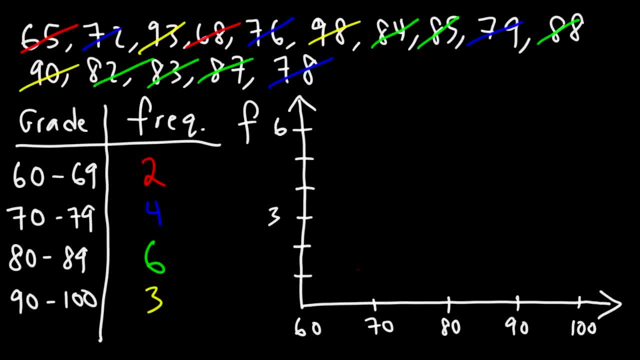 So let's plot the first one Between 60 and 69,, which is close to 70,, the frequency is a 10.. So let's plot the first one Between 60 and 69,, which is close to 70,, the frequency is a 10.. 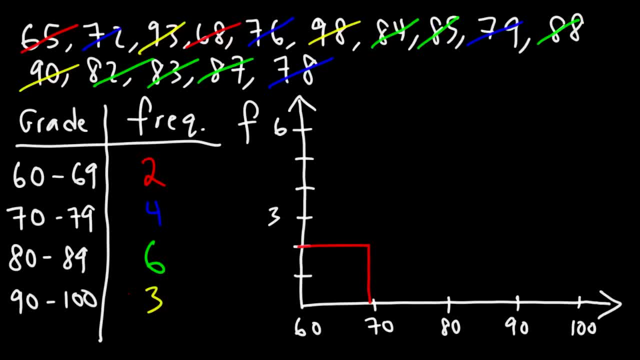 The frequency is a 2. So it's going to look like that- And then between 70 and 79,- four students got a grade in that region. I'm going to use the same color- And between 80 and 89,. 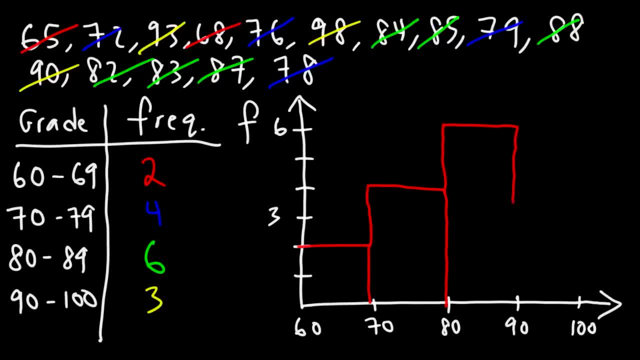 six students fall in that category And between 90 and 100,. only three students received an A, So let's put the grade. So this is a D, two students got a D, four students got a C and six students received a B and three. 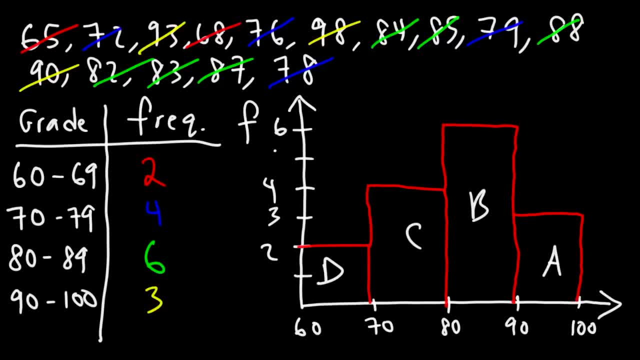 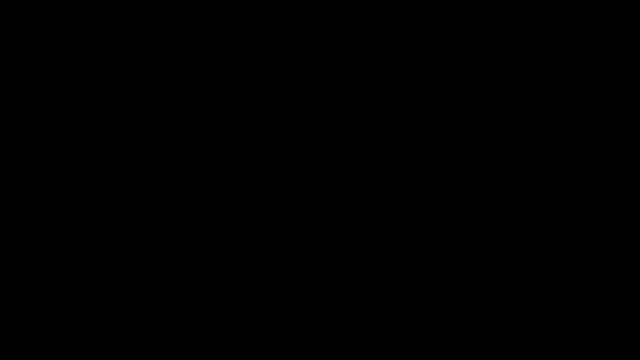 students received an A. So that's how you can create a histogram from a data set like this, using a frequency distribution table. Now there's something else that we need to go over, and that is making a table with the frequency, the relative. 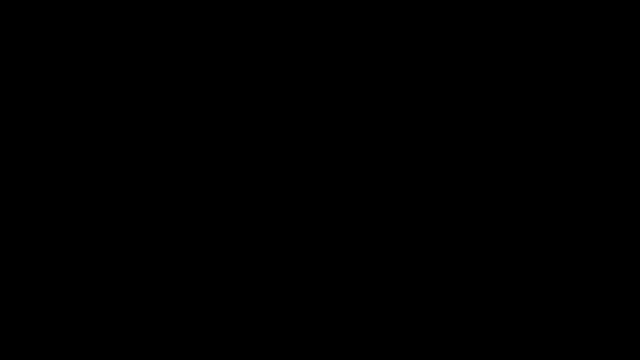 frequency and also the cumulative relative frequency. So let's say we have the numbers two, three, five, three, six, eight, seven, eight, three, three, five, three, seven, three, eight, five, two, seven, eight, three. So we're going to have four columns. The first, 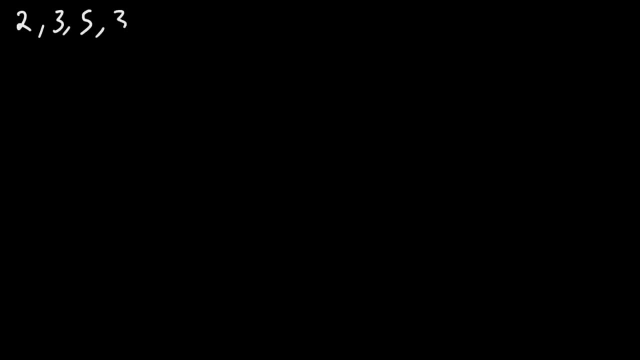 two, three, five, three, six, eight, seven, eight, three, three, five, three, seven, three, eight, five, two, seven, eight, three. So we're going to have four columns. The first column 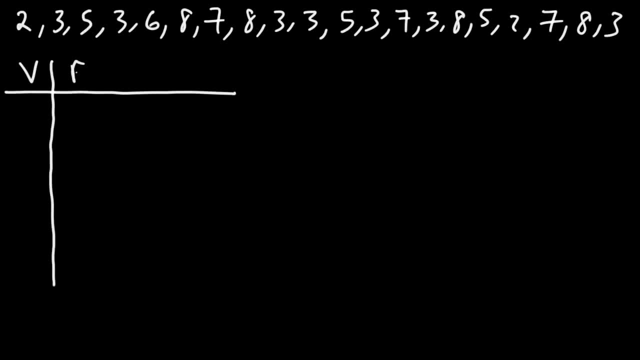 is going to be the value, The second column will be the frequency, The third column is going to be the relative frequency And the last one is going to be the cumulative relative frequency. So the lowest value that we have in our list is two. 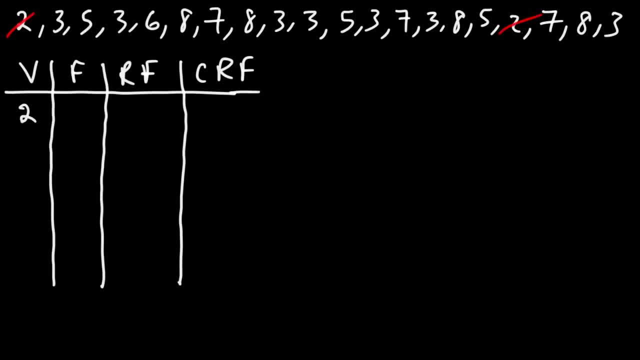 And notice that we have two twos. So the frequency for that number is two. Next we have a three And we have one, two, three, four, five, six, seven, threes. So that's the frequency. The next number in the list is five. 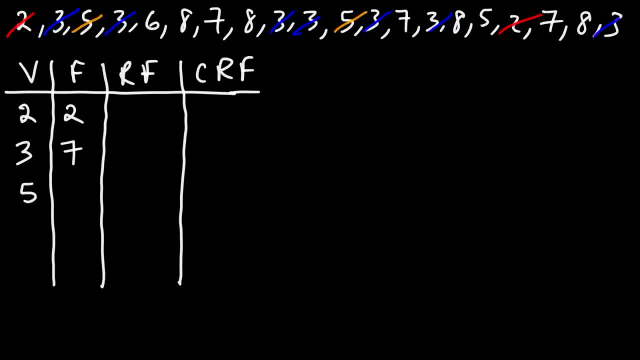 We have one, two, three, fives. Now we only have one six, which is here. Next is a seven, And there's one, two, three, sevens, And I need to extend this list- And then, finally, we have some eights. 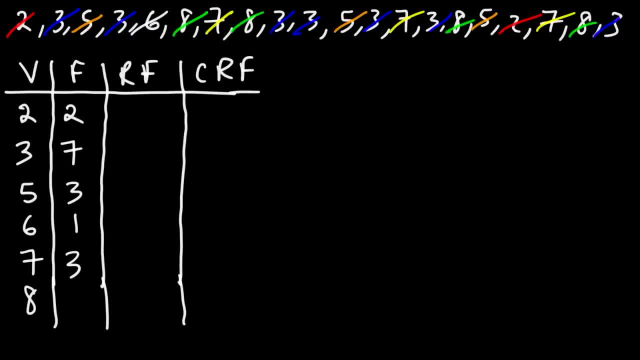 One, two, three, four, eights. Now let's take the sum of the frequency column. So if we add these numbers, two plus seven is nine plus three, that's twelve plus one is thirteen plus three is sixteen plus four is twenty. 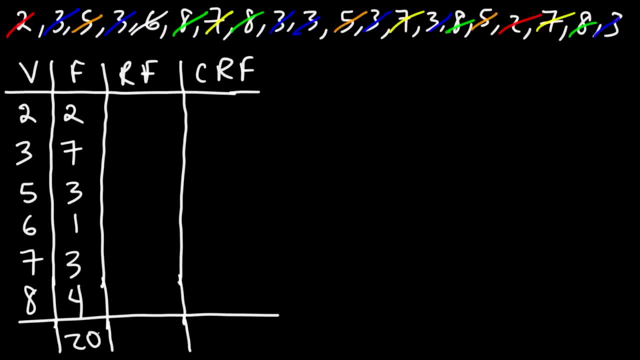 So we have a total of twenty numbers in our set. Now how do we calculate the relative frequency? So for the first entry in that column, take the frequency and divide it by the total number of numbers that you have in the data set. So the relative frequency is basically: 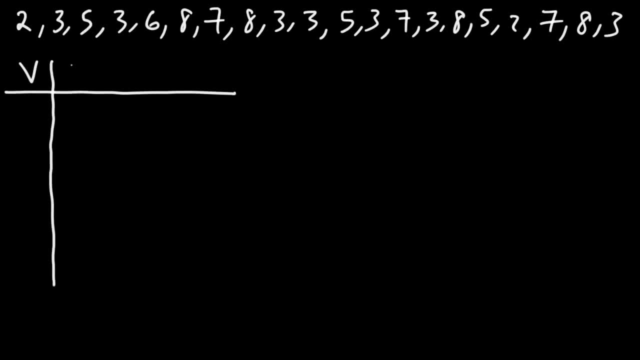 column is going to be the value, the second column will be the frequency, the third column is going to be the relative frequency and the last one is going to be the cumulative relative frequency. So the lowest value that we have in our list is two, And notice that we have two. 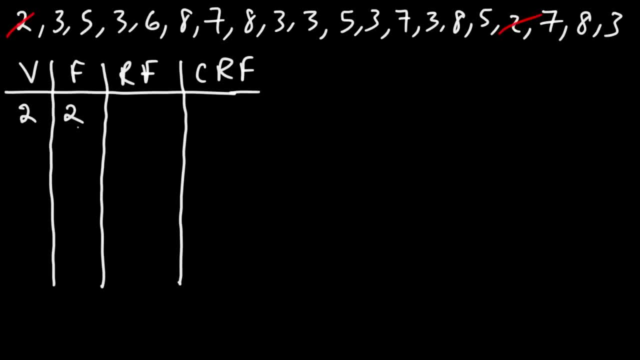 twos. So the frequency for that number is two. Next we have a three, And we have one, two, three, four, five, six, seven, threes. So that's the frequency. The next number in the list is five. We have one, two, three. 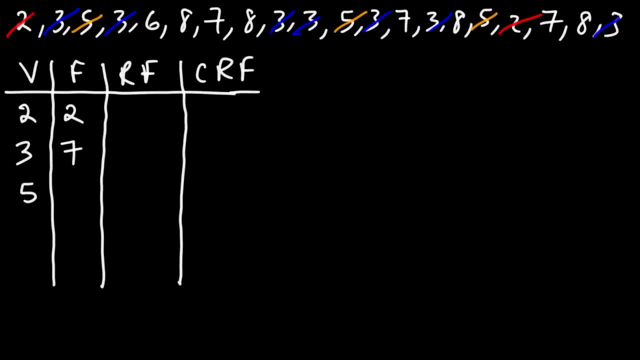 two, three, fives. now we only have one six, which is here, next is a seven, and there's one, two, three, sevens. I need to extend this list. and then, finally, we have some eights: one, two, three, four eights. now let's take the sum of the frequency. 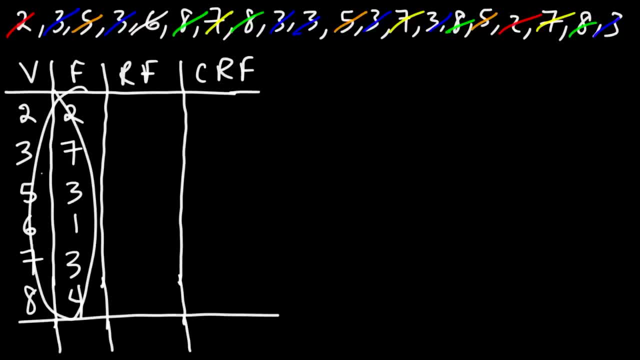 column. so if we add these numbers, 2 plus 7 is 9 plus 3, that's 12 plus 1 is 13 plus 3 is 16, plus 4 is 20, so we have a total of 20 numbers in our set. now how do we? 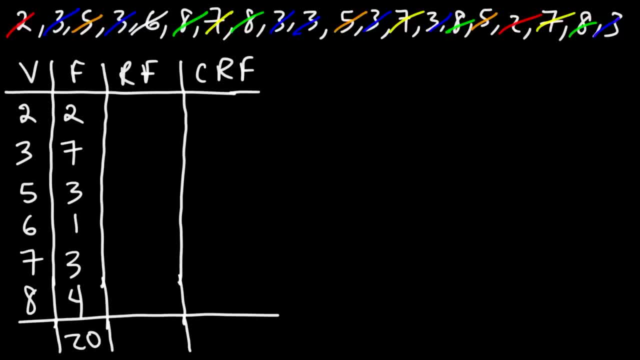 calculate the relative frequency. so for the first entry in that column, take the frequency and divided by the total number of numbers that you have in the data set. so the relative frequency is basically the frequency divided by n. so for the first one is going to be 2. 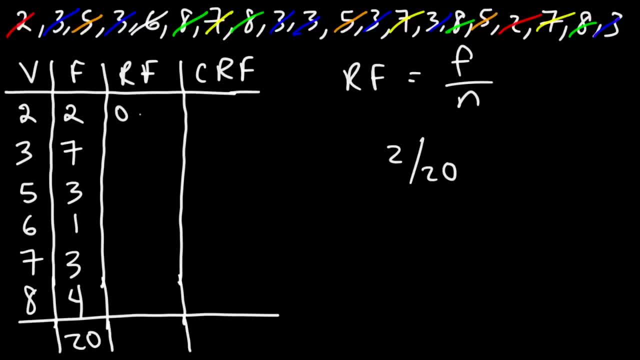 over 20, which is 1 out of 10, and so that's point 10. for this one is going to be 7 divided by 20, which is point three, five, and for the next one it's 3 divided by 20, which is point 15, and then it's 1 divided by 20, that's. 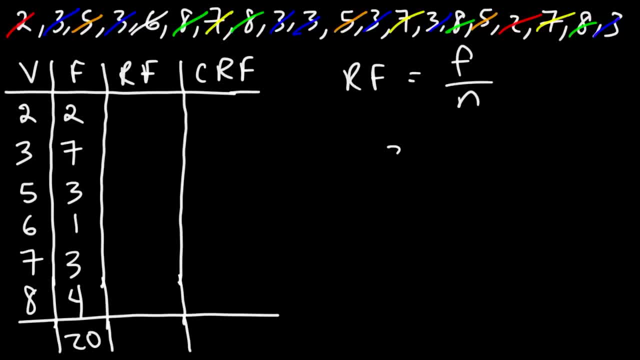 the frequency divided by n. So for the first one it's going to be two over twenty, which is one out of ten, and so that's point ten. For this one, it's going to be seven divided by twenty, which is point three. five: 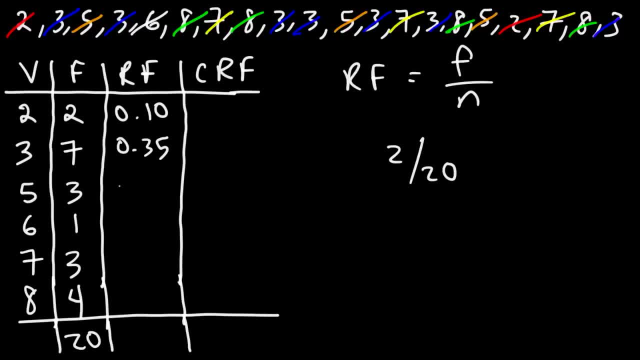 And for the next one, it's three divided by twenty, which is point fifteen, and then it's one divided by twenty, that's point zero. five, Three over twenty is point fifteen again, and then four out of twenty is point twenty. Now, if you add up all of these numbers, 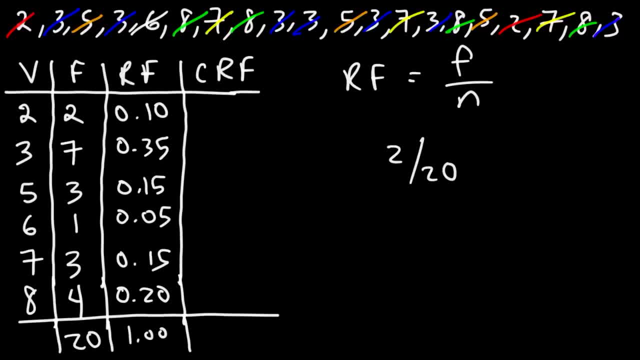 you should get one. Next we have the cumulative relative frequency. So we're going to start with point ten and then we're going to add these two numbers, Point ten plus point three. five is point four. five Now point four, five plus point fifteen. 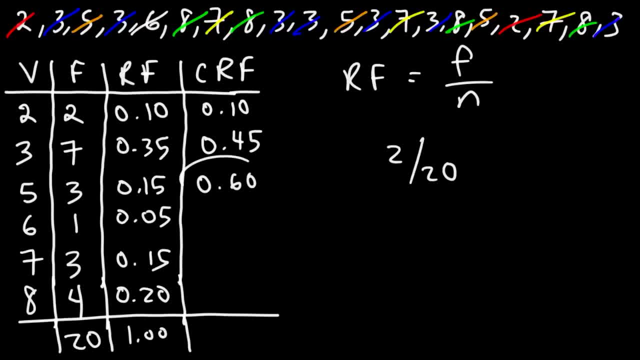 that's point sixty. And then if we add point sixty and point zero five, that's going to be point sixty five, And then add in those two numbers, that's going to give us point eighty, and then point eighty plus point twenty will give us one. 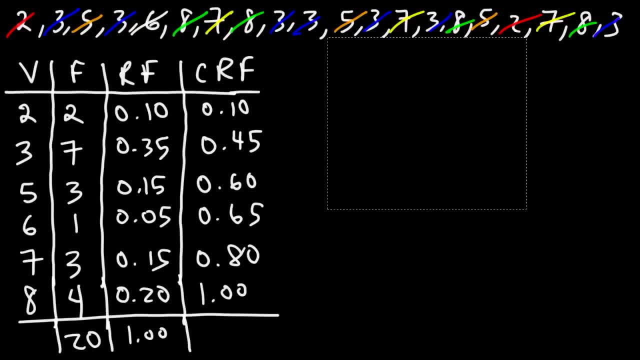 So that's how you can complete the cumulative relative frequency table, given a data set, Now let's talk about how we could use this information. Using this table, what is the value of the sixtieth percentile? What would you say? So what we need to do is look at. 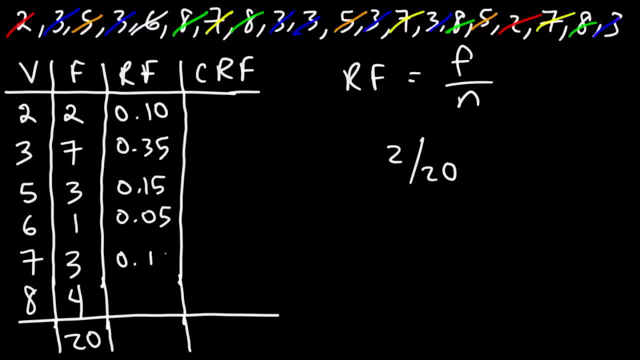 point 0, 5, 3 over 20 is point 15 again, and then 4 out of 20 is point 20. now, if you add up all of these numbers, you should get one, and next we have the cumulative relative frequency. so we're going to start with point 10 and then 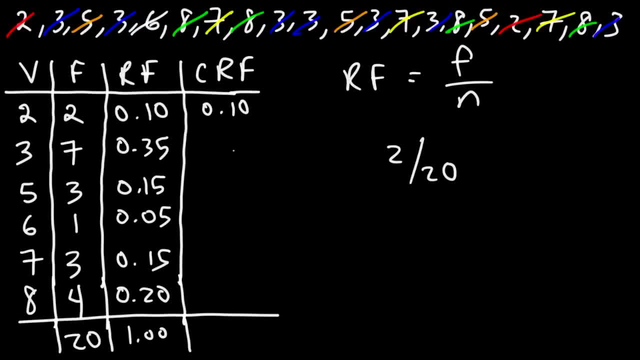 we're going to add these two numbers, point 10 plus point three, five, it's point four. five. now, point four, five plus point 15, that's point 60, and then, if we add point 60 and point 0, 5, that's going to be point 65, and then add: 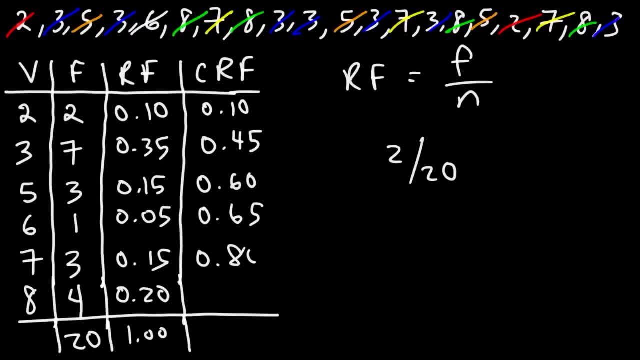 in those two numbers. that's going to give us point 80, and then point 80 plus point 20 will give us one. so that's how you can complete the cumulative relative frequency table, given a data set. now let's talk about how we could use this. 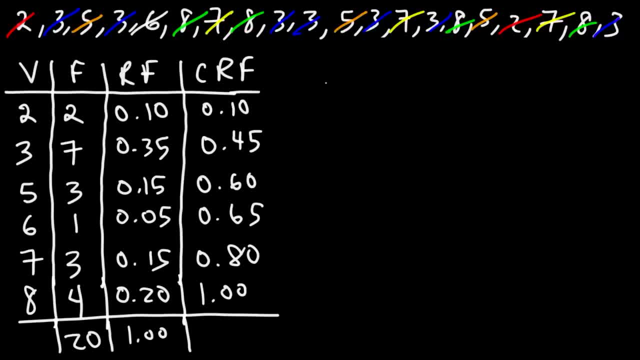 information using this table. what is the value of the 60th percentile? what would you say? so what we need to do is look at the cumulative relative frequency. so the 60th percentile will end here. now, notice that it's exactly point 60, which corresponds to sixty percent to. 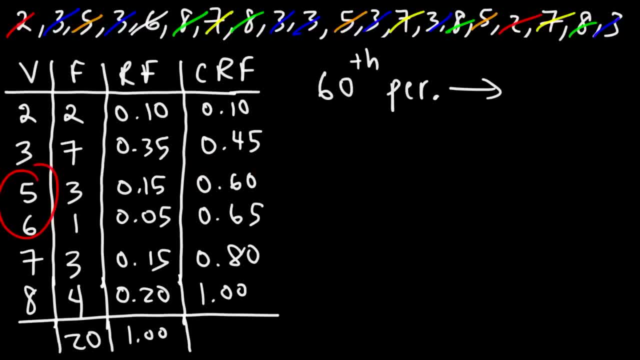 find the 60th percentile, you need to average these two values, so you have to do five plus six divided by two. the average of five and six is 5.5, and so that's going to be the 60th percentile. now what about the 80th percentile? 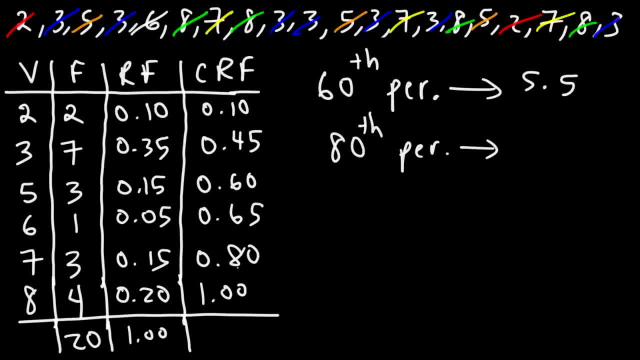 you notice that we have exactly point eight in the cumulative relative frequency column. so what we're going to do is we're going to average these two numbers. the average of seven and eight is 7.5. now what if it's not listed in the cumulative relative frequency table? for 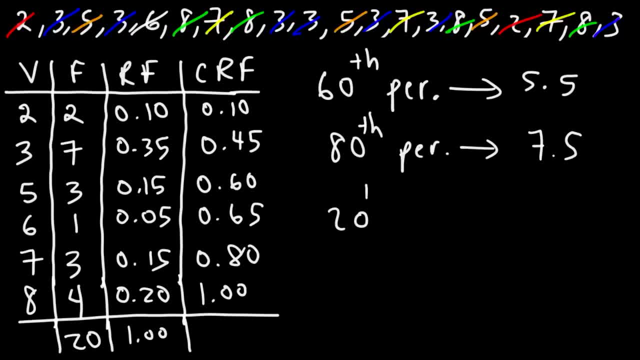 instance, let's say, if we have, or if you want to find the 20th percentile, what value corresponds to that? now, the 20th percentile is between 0.10 and 0.45. it's important to understand that after 0.10 you're going. 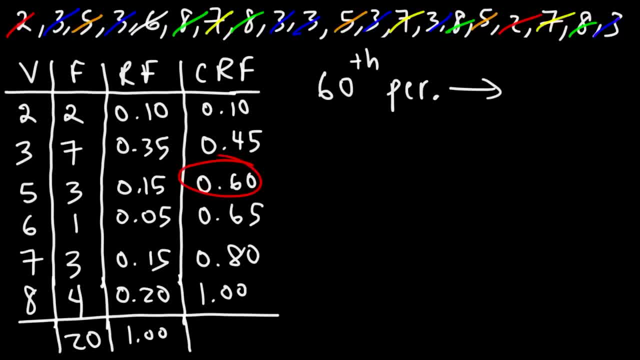 the cumulative relative frequency. So the sixtieth percentile will end here. Now notice that it's exactly point sixty, which corresponds to sixty percent. To find the sixtieth percentile you need to average these two values. So you have to do five plus six. 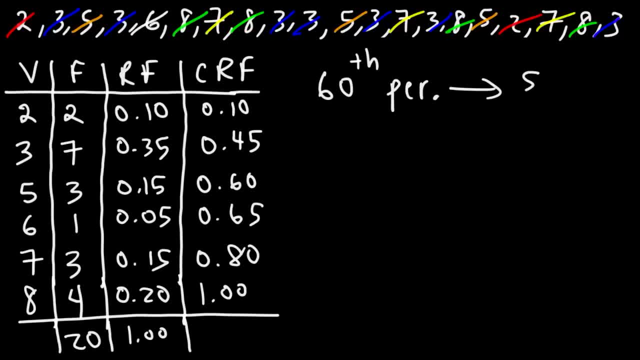 divided by two, The average of five and six is five point five, And so that's going to be the sixtieth percentile. Now what about the eightieth percentile? So notice that we have exactly point eight in the cumulative relative frequency column. 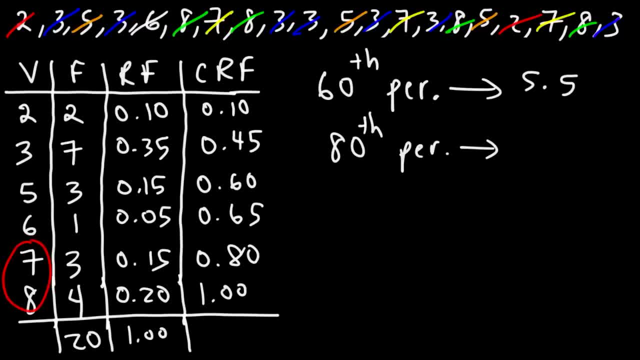 So what we're going to do is we're going to average these two numbers. The average of seven and eight is seven point five. Now what if it's not listed in the cumulative relative frequency table? For instance, let's say, if we have: 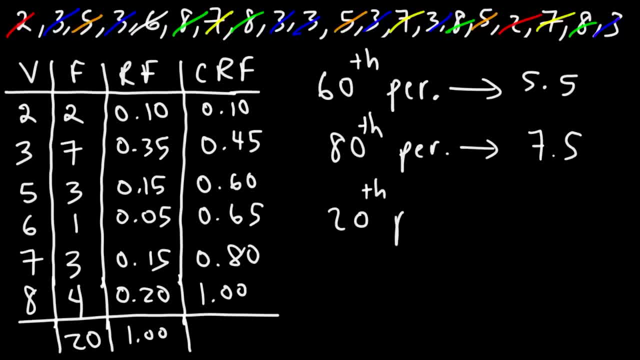 or if we want to find the twentieth percentile, What value corresponds to that? Now, the twentieth percentile is between point ten and point four, five. It's important to understand that after point ten, you're going to exceed the value of two. You're going to go into the threes. 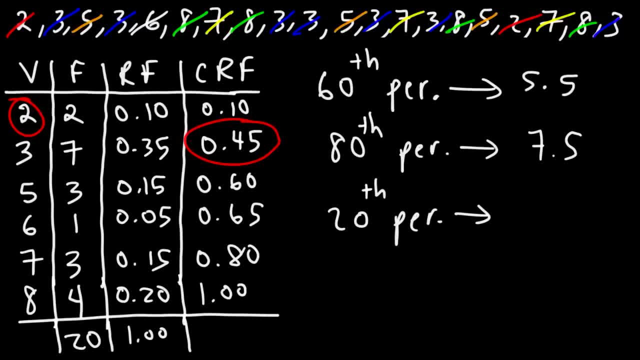 And after point four, five, you're going to move from the threes to the fives. So the twentieth percentile, because it's more than two but less than three, it's going to be three. There's no numbers in between here. 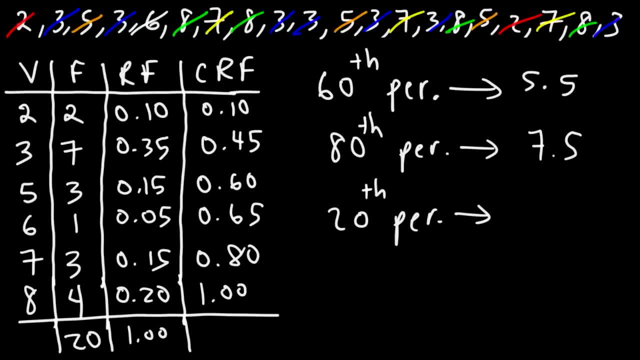 if you look at the data that we have. So the twentieth percentile is going to fall in this number. To explain it better, it's important to understand that between zero and point ten, the value is two. Between point ten and point four, five. 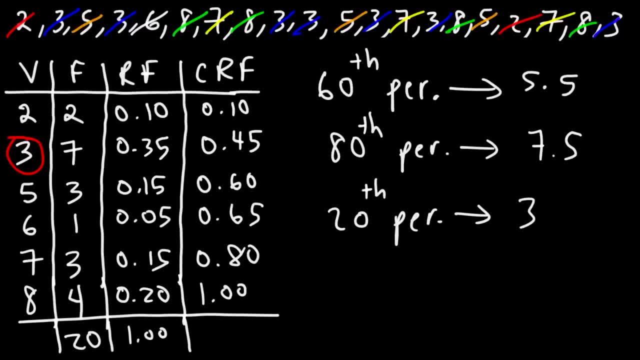 the value is three. Now, if your percentile falls between point four, five and point sixty, not including point four, five and point sixty, but if it's between those numbers, then it's going to be five, It's going to be six. if it's between point sixty and point six, five. 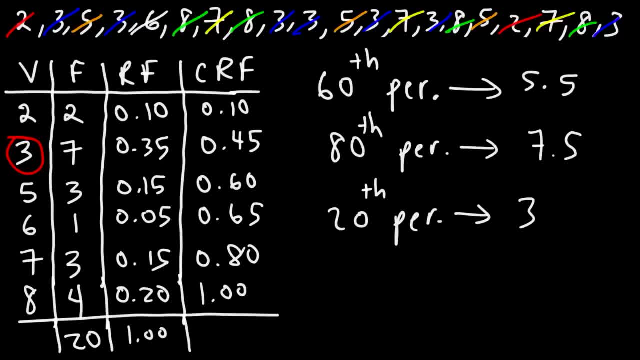 And it's going to be seven if it's between point six, five and point eight. So let's say, if we want to determine the seventy-fifth percentile, The seventy-fifth percentile is between point six, five and point eight. So, because it's more than point six, five, 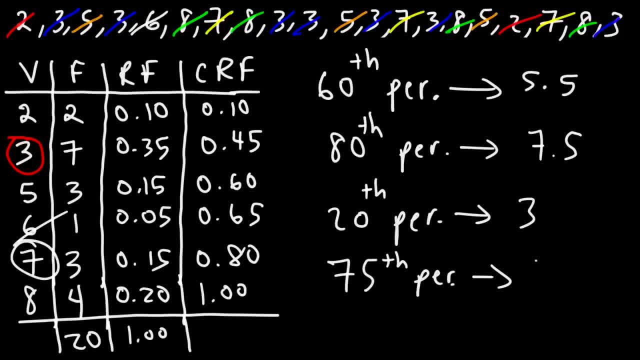 we're not going to have the value six, We're going to get seven. So that's going to be the seventy-fifth percentile. Now let me help you to see this visually so that it makes more sense. Let's begin by arranging the numbers. 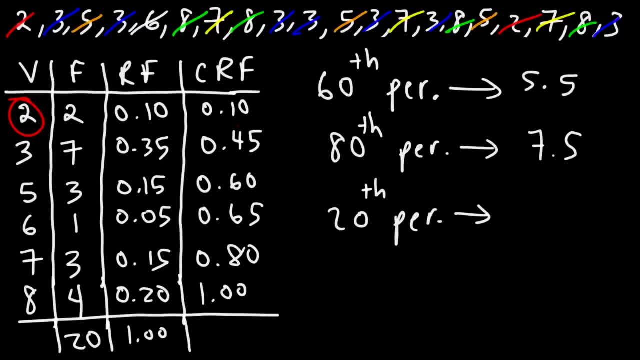 to exceed the value of two, you're going to go into the threes and after 0.45 you're going to move from the threes to the fives. so the 20th percentile, because it's more than two, but less than three, it's going to be three. there's no. 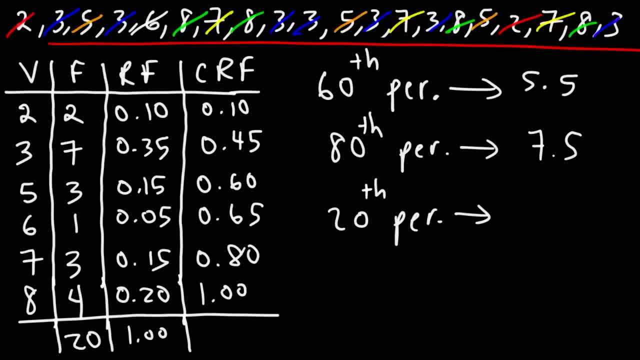 numbers in between here if you look at the data that we have. so the 20th percentile it's going to fall in this number. to explain it better, it's important to understand that between 0 and 0.10, the value is two. between point 10 and 0.45, the value is three. 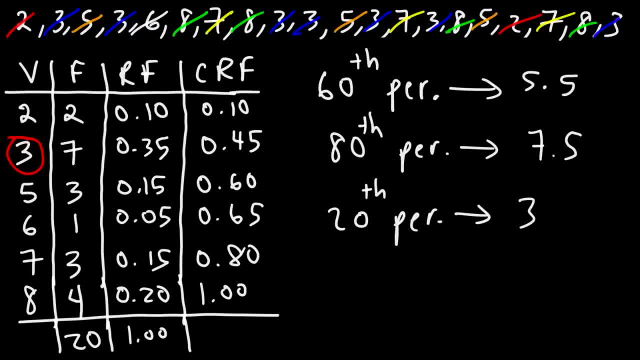 now, if your percentile falls between 0.45 and 0.60- not including 0.45 and 0.60, but it's if it's between those numbers- then it's going to be five. it's going to be six if it's between 0.60 and. 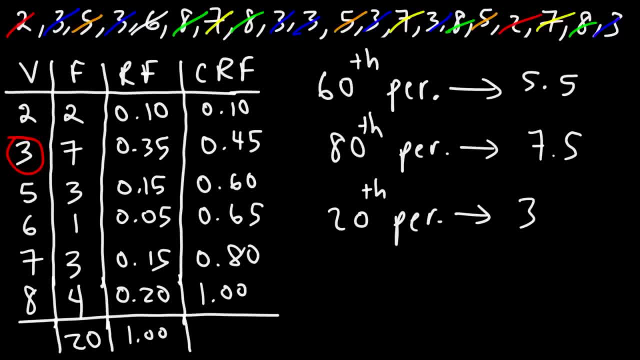 0.65 and it's going to be seven if it's between 0.65 and pointing. so let's say, if we want to determine the 75th percentile, the 75th percentile is between 0.65 and 0.8. so because it's more than 0.65, we're not going to have 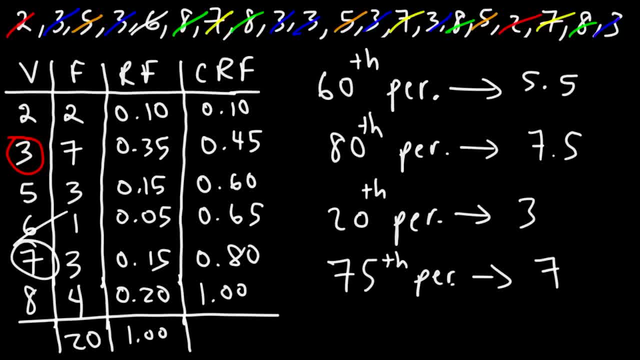 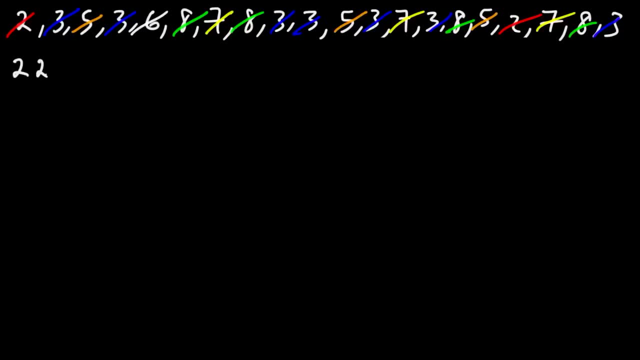 the value six, we're going to get seven, so that's going to be the 75th percentile. now let me help you to see this visually so that it makes more sense. let's begin by arranging the numbers in increasing order. so we have two, twos, we 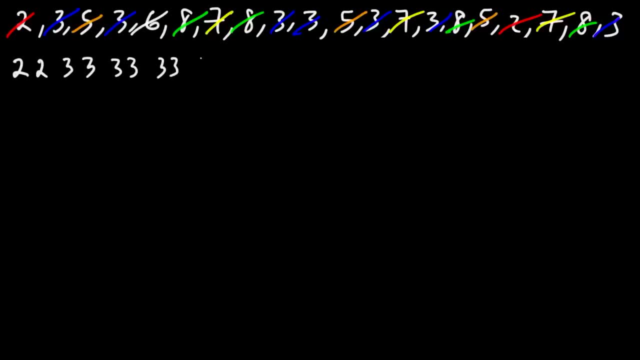 have a total of seven threes and we have three fives, one six, three sevens and four eights. now I'm writing these in pairs of twos and you'll see why we have a total of 20 numbers and if you take 20 and divided by two, you're gonna get ten equal parts. 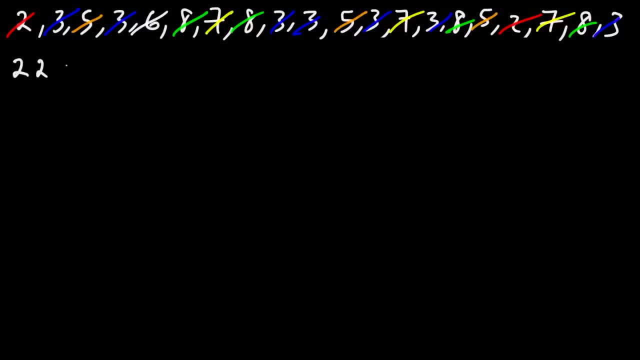 in increasing order. So we have two twos, We have a total of seven threes And we have three fives, one six, three sevens and four eights. Now I'm writing these in pairs of twos. 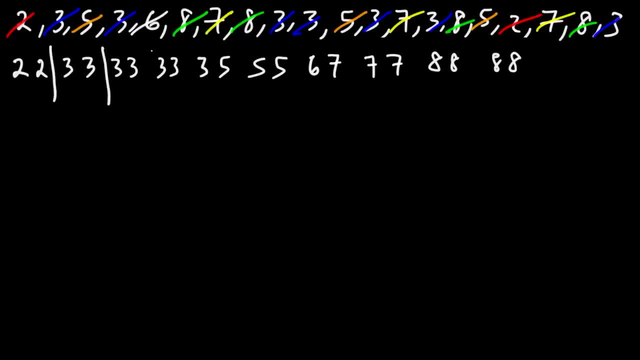 And you'll see why. We have a total of twenty numbers And if you take twenty and divide it by two, you're going to get ten equal parts. So this is going to be the tenth percentile. Let me put that in a different color. 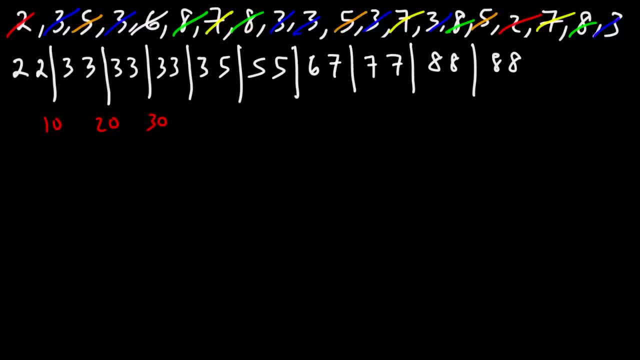 So here's the tenth percentile, the twentieth percentile, the thirtieth and so forth. So this would be the hundredth percentile. There's nothing higher than that. So the first thing that we went over was the sixtieth percentile. 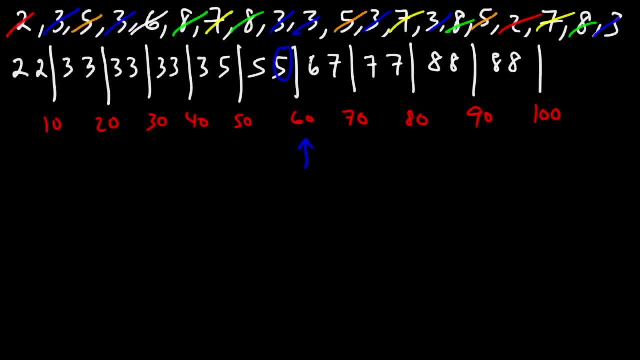 which is here. So notice that we have a five on the left and a six on the right. So we need to average that. So we need to average five and six. And so we said the sixtieth percentile was five point five. 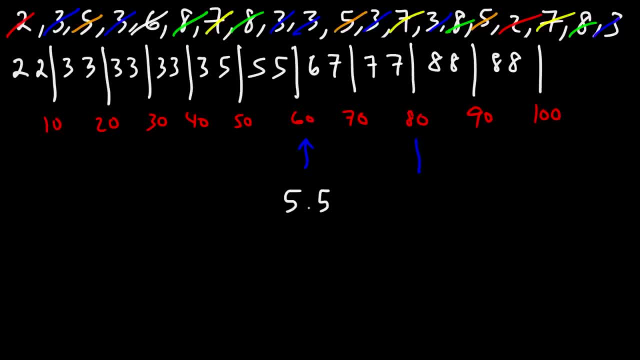 The second one was the eightieth percentile, which is here. Notice that it's between two different numbers, seven and eight. So if we average seven and eight, it will give us seven point five. Now, after that, we talked about the twentieth percentile. 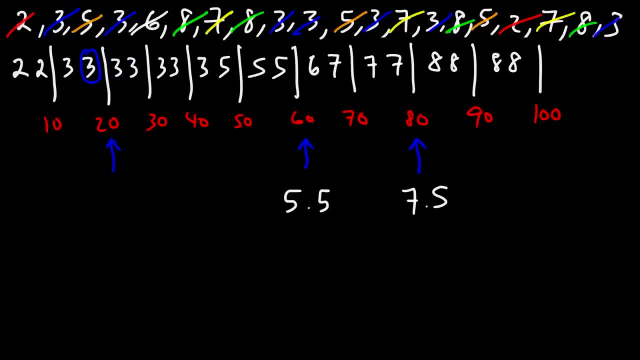 And the two numbers that it's between are identical to each other. The twentieth percentile is just three, And the last one was the seventy-fifth percentile, which is between seventy and eighty, And so these two numbers are just seven, And so the seventy-fifth percentile has to be seven. 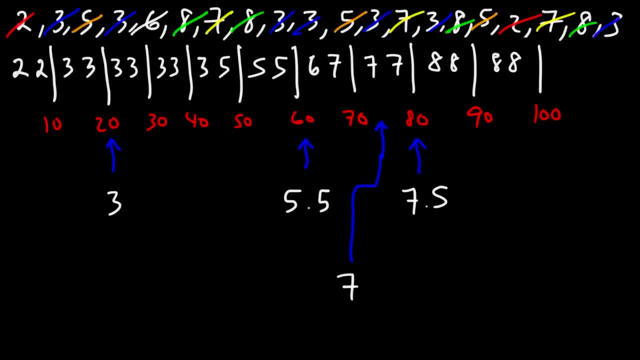 So now you can visually see the values that correspond to the different percentiles And, if you want to, you can put zero as well. I forgot to do that, But that's basically it for this video, So hopefully it gave you a good.